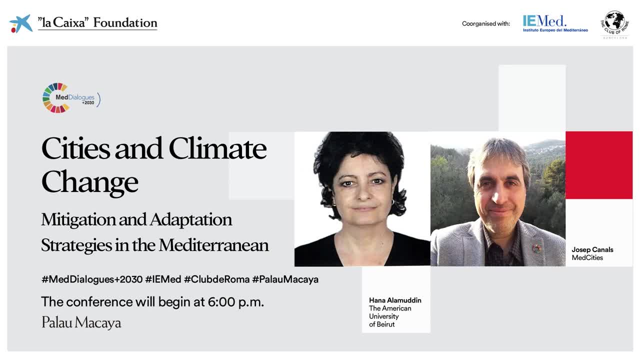 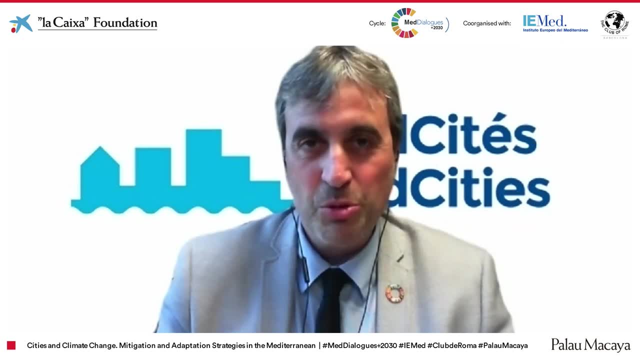 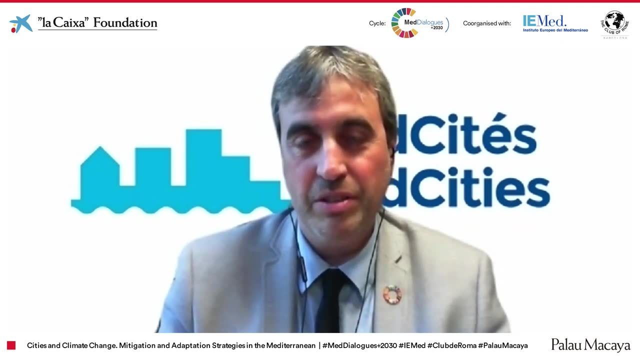 Hello, Good afternoon to everyone. Bonsoir, Thank you very much for being here. My name is Giuseppe Canals, Secretary General of MedCities, and I'm very glad and thankful for being invited by the Euro-Mediterranean Institute, the EMET, the European Institute of the Euro-Mediterranean. 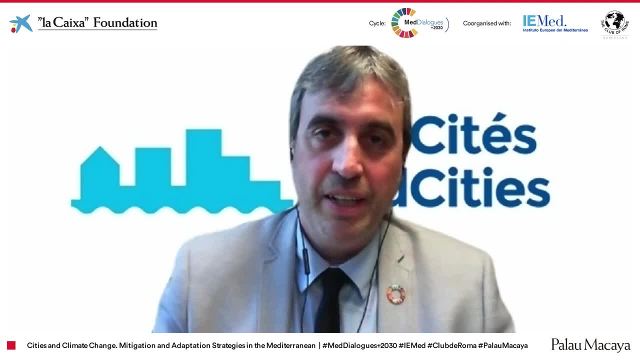 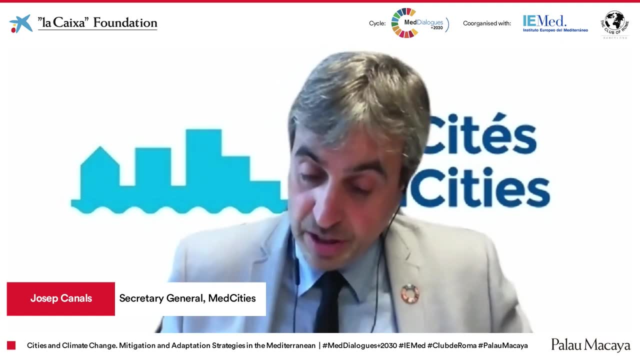 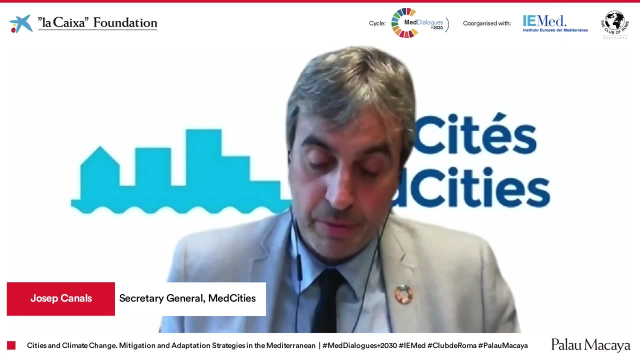 Thank you very much for having me, for having us. Let me tell you some words in my mother tongue, Catalan. Thank you very much. This is the fifth dialogue out of six of a conference cycle called The Road to a More Sustainable and Climate Resilient Mediterranean. 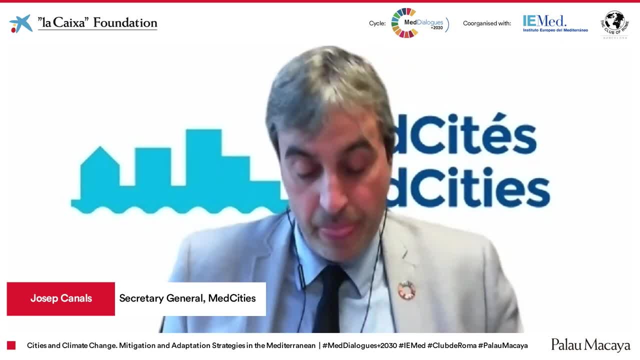 Thank you very much. This is the fifth dialogue out of six of a conference cycle called The Road to a More Sustainable and Climate Resilient Mediterranean. This is the dialogue number five: Cities and Climate Change Mitigation and Adaptation Strategies in the Mediterranean. 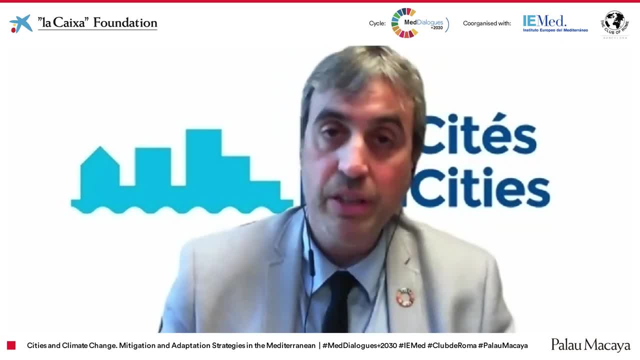 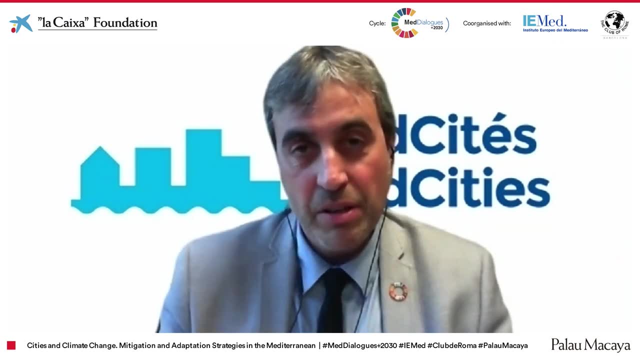 He's here with me, Hannah Alamuddin, Mrs Hannah Alamuddin, which I will introduce later more properly. Thank you very much for being here too, And let me first do some reflections that why we're doing it here. I would say that maybe this is the core of the. 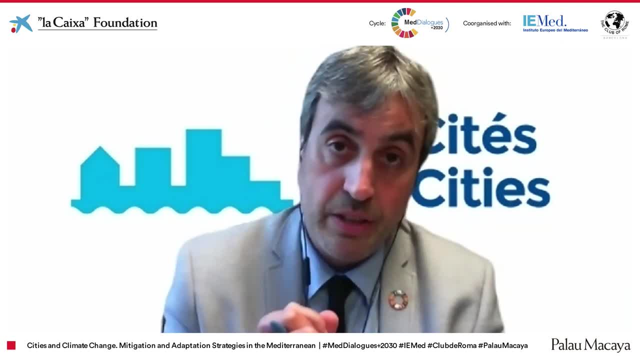 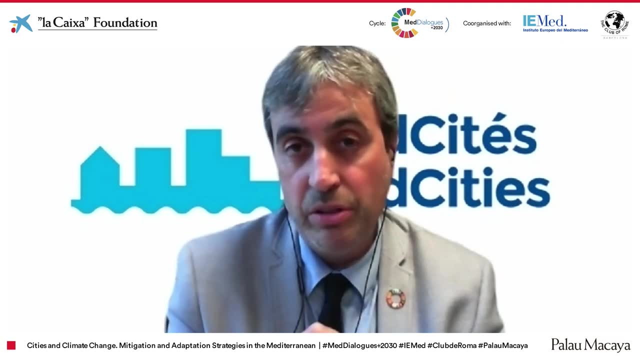 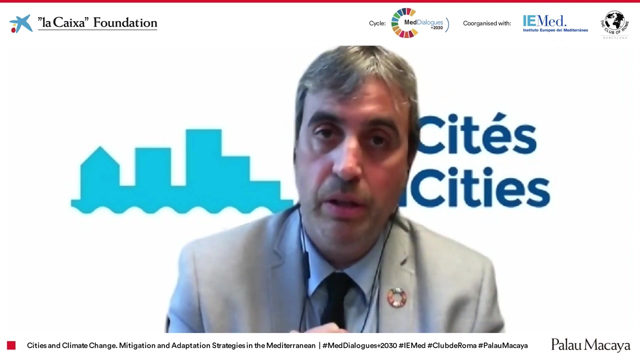 the climate change, in my opinion, because in cities are happening things, things very fast: The increasing urbanization, the type of land use, how the cities are using them, the land use. many cities are increasing their urbanizations without proper urban planning. in our region, So the impacts are so great. And then, of course, of course. of course, like many communities in Latin America, we are present in the cities' 월 USDAias, in investments and changing shoes and or对s and orbits around it. And of course, because of the climate change, it's sort of all concerned that we're doing the work well. and what'sу the main obstacles to such a market change? for my opinion? Because in cities are things very fast: the increasing urbanization, the type of land use, how the cities are using the land use. many cities are increasing the urbanizations without proper urban planning in our region, So the impacts are. 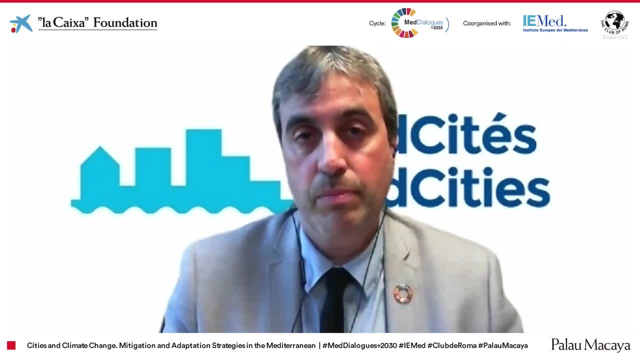 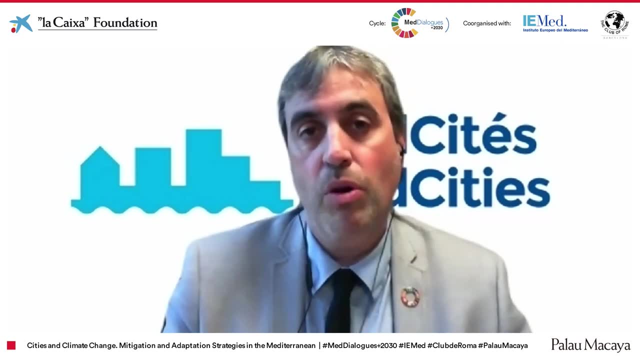 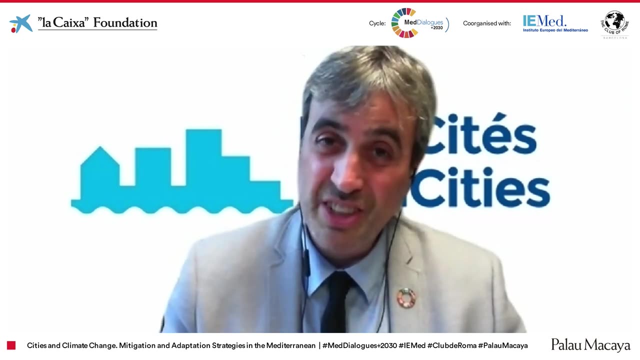 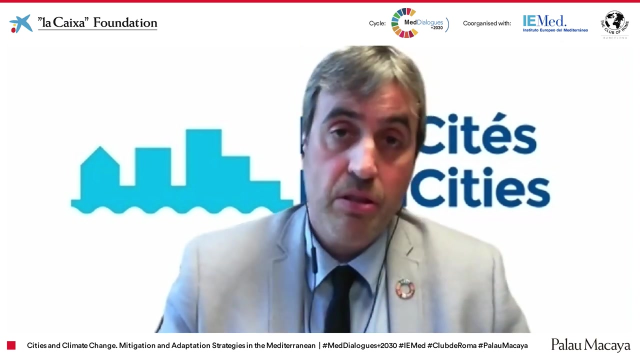 Many people have been attracted by cities because in countryside it's a difficult way of living. So they are trying. they are seeking for better lives in the Mediterranean region in cities. Cities are increasing too fast, I would say So the impact of this increasing and the existing, the already existing cities are several. 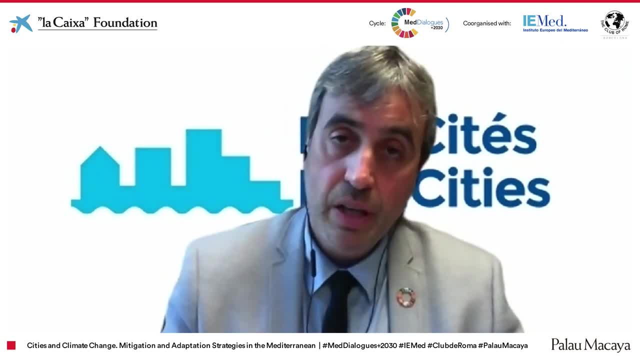 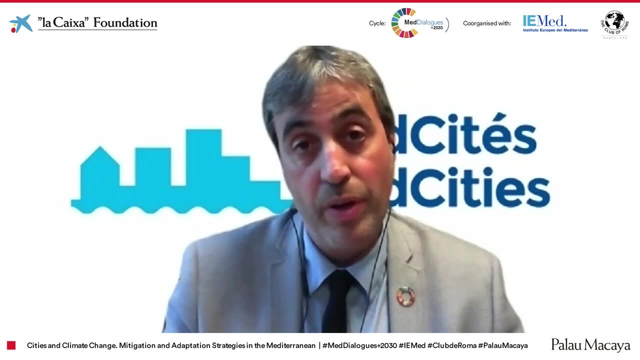 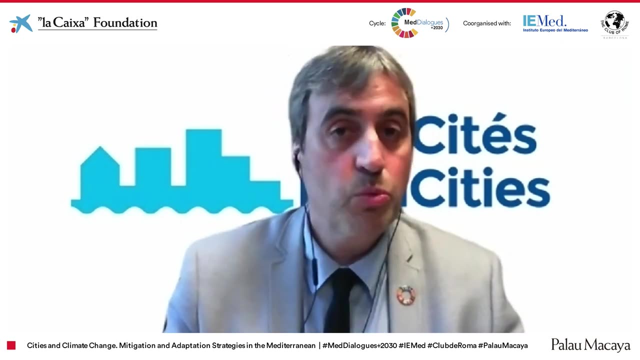 You know for sure, is the mobility, the urban, the air pollution, the noise pollution, As I said, the use of land without planning. many times There is the fragmentation of biodiversity. many times Many cities with great values in biodiversity then has been affected. 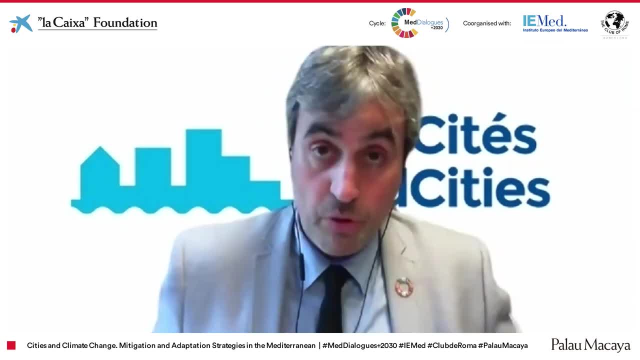 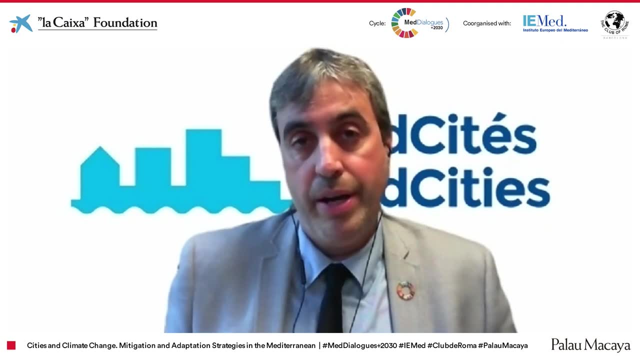 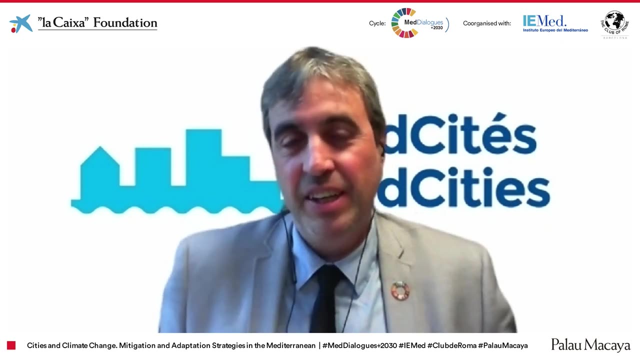 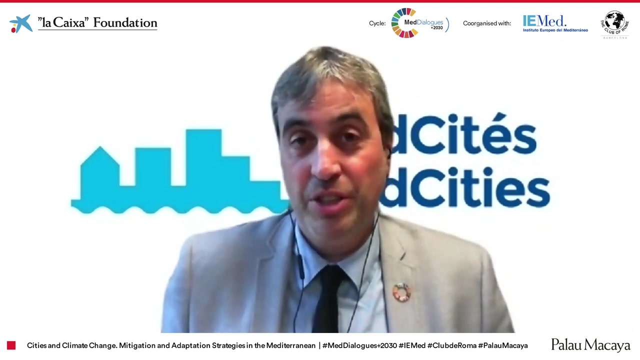 They have been losing this great heritage that is biodiversity. All of these challenges are faced by cities, And cities suffer, on the other hand, the lack- you know, many of you- the lack of competencies. I've been a mayor myself and I know how mayors suffer because they have the problems there. 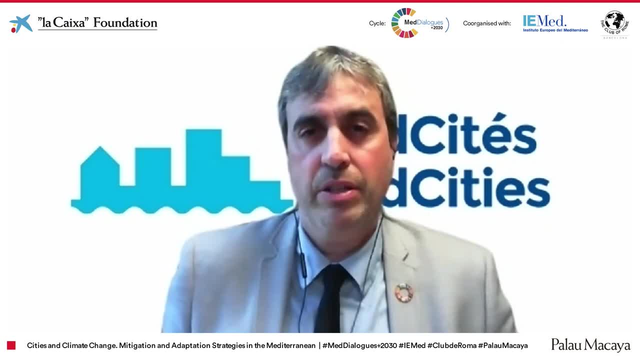 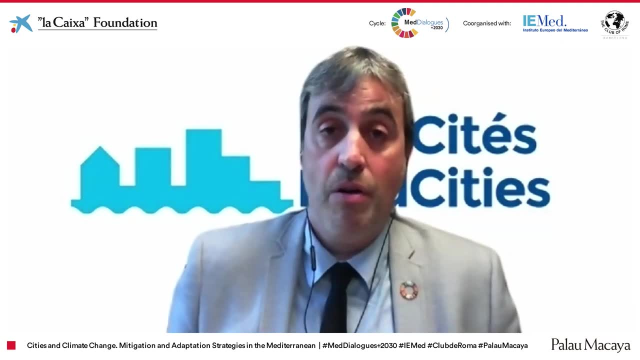 They have the people to attend, The people to do the work, The people to give them services, But the lack of competencies, the lack of resources, The lack of all the needs: the human resources, the financial resources, and the power, the competencies. 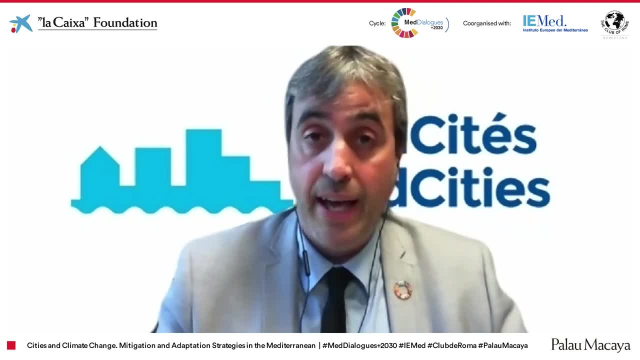 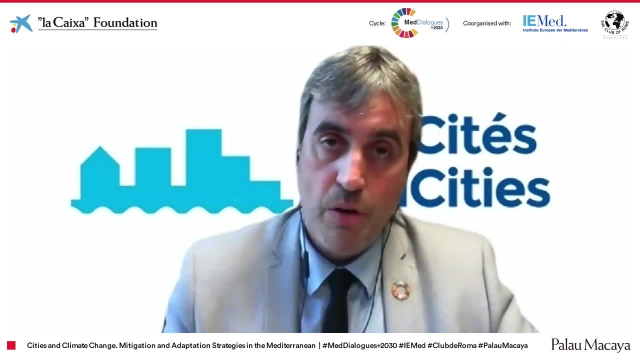 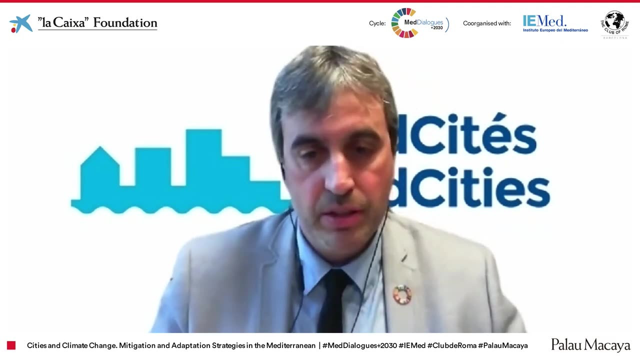 which, in many ways, in many cases, are held by states or, in some cases, by regions. So this is an added difficulty for these cities. Let me introduce briefly Why we are here on behalf of mid cities. Why, What is mid cities? 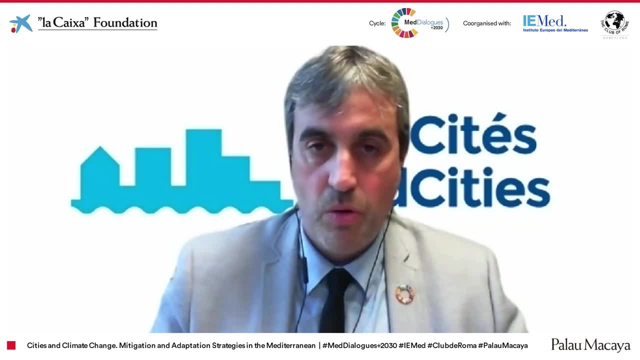 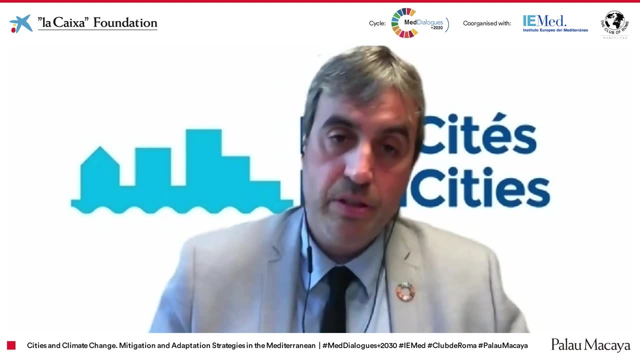 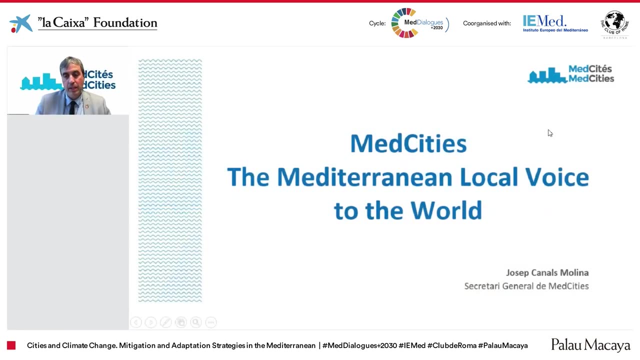 I will share with you, Hopefully this is going properly. So, mid cities, we like to say, maybe not so humbly, but we like to say that we are the Mediterranean local voice to the world. We are a network of 63 municipalities. 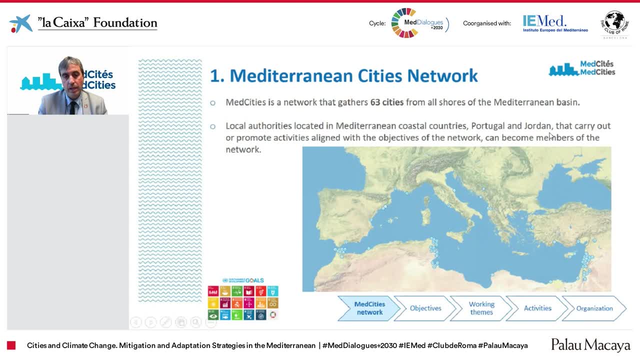 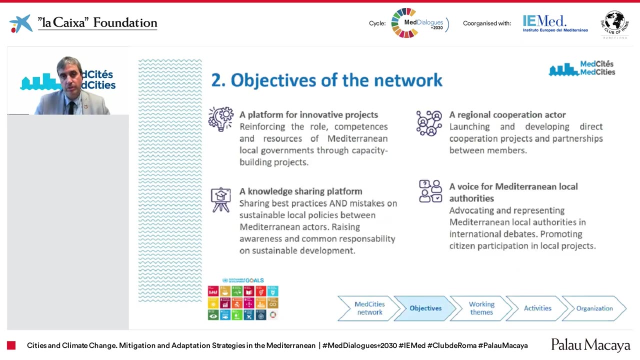 We are a union of municipalities from all shores of the Mediterranean Basin, All of them from states that has coastal site with the Mediterranean Sea, plus Portugal and Jordan. So what do we do? We work together, We share experiences. We, as association, give services to our member cities, to our local authorities. 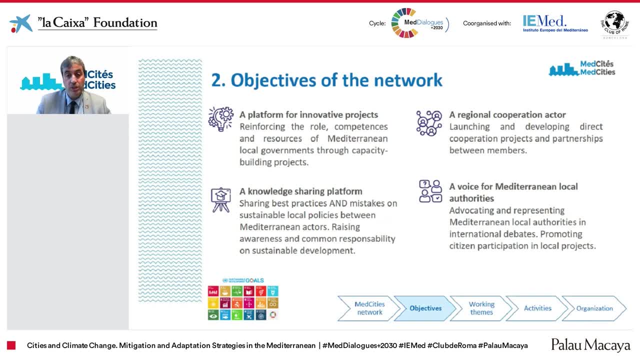 We are a platform of innovative projects. We try to reinforce the competencies and the capacity building of our local authorities, either representatives or technical staff. We launch and develop direct cooperation projects and partnerships between members and with other partners, with other stakeholders of the region. 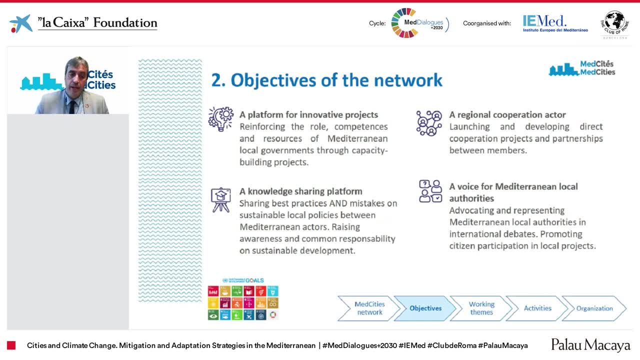 For example, we are conducting four interactive projects. We are knowledge sharing platform. We try to boost, to share all the good practices and the mistakes also among our member cities, to not to try to invent the wheel every time, So to see what other members are doing and how we can and they can learn from each other. 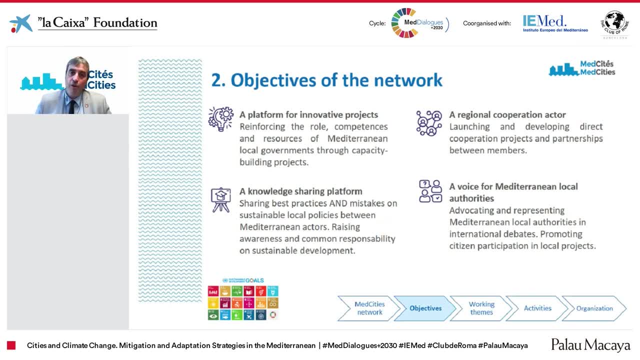 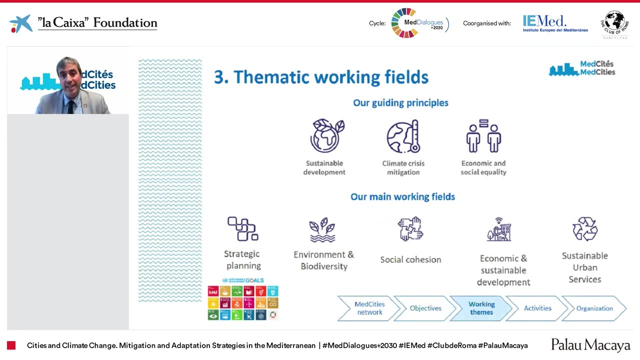 And we also try, from this accumulating of project of knowledge, We also try to project and to be a political voice with all the Mediterranean. We are working with local authorities, local authorities in the region, promoting and giving voice to them and representing them in other arenas, in other agoras, with the states, with regions. 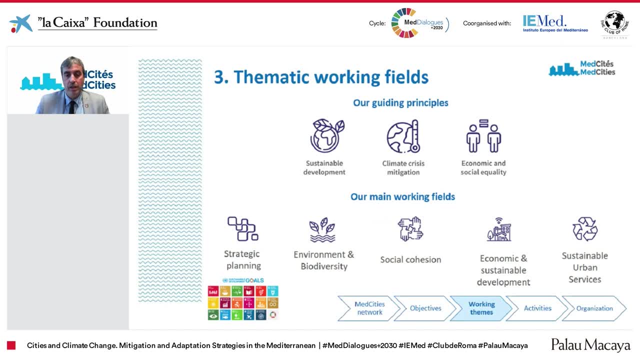 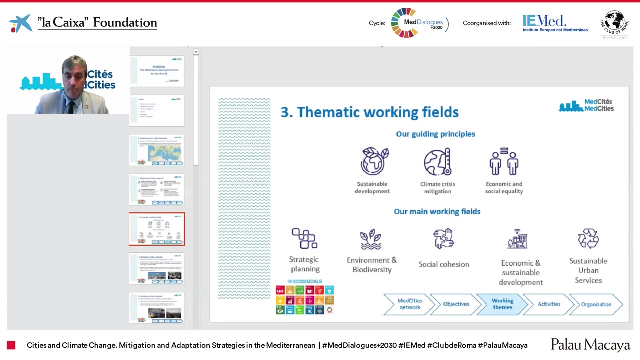 We work in this thematic working fields: strategic planning, environment and biodiversity, more and more social cohesion, economic sustainable development and urban services. These are our principles: Sustainable development, Development, Climate crisis mitigation And economic development with a sustainable perspective. Let me stop here. 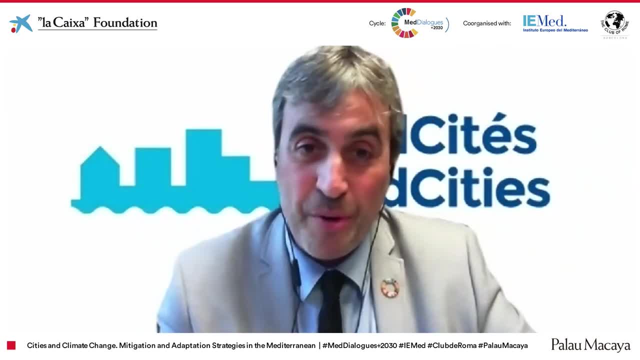 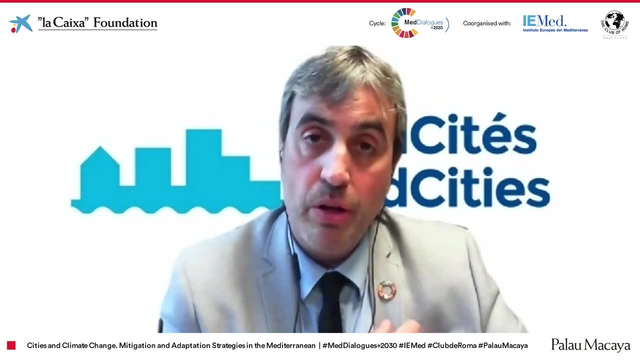 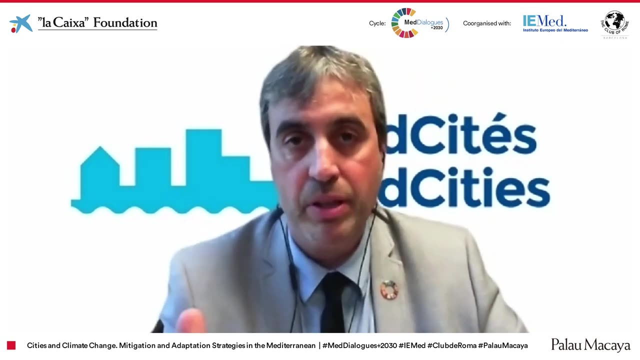 And just to this is why we are here, why we have been invited, and we are thankful for that And all those characteristics that I shared with you and you know a lot, which is all the impacts, All the impacts and the challenges that cities are facing. 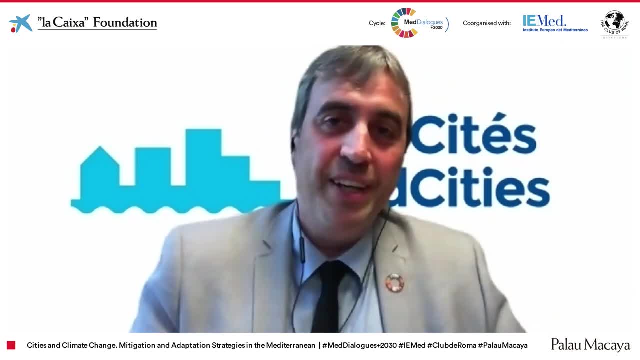 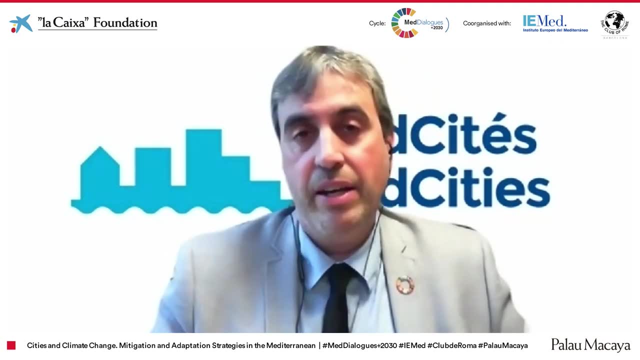 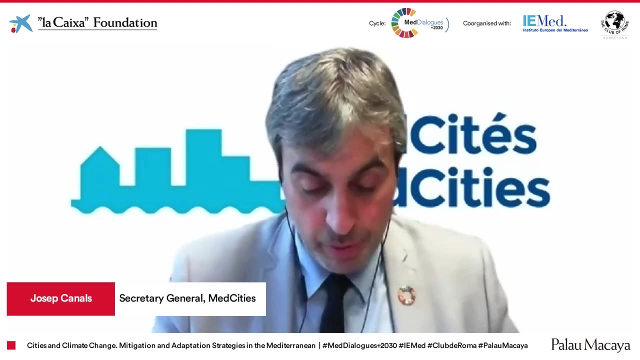 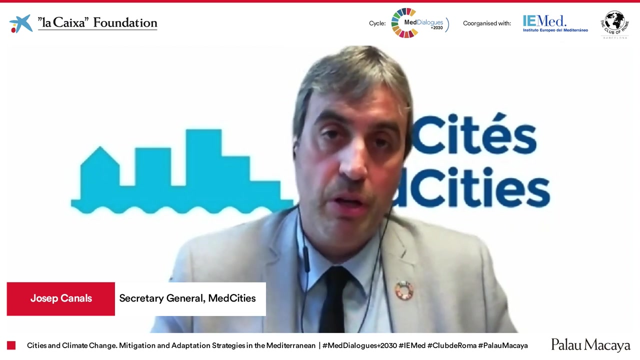 The local authorities. in fact, we speak about cities by our local authorities and our people that are living there, and with hopes and expectations- also Expectations, excuse me. So I would like to bring some to pose some questions: How local authorities can tackle to these challenges. 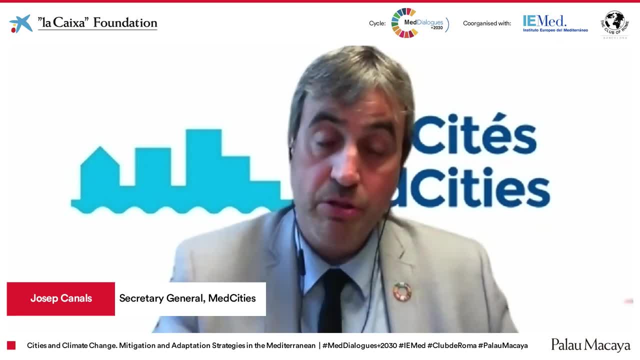 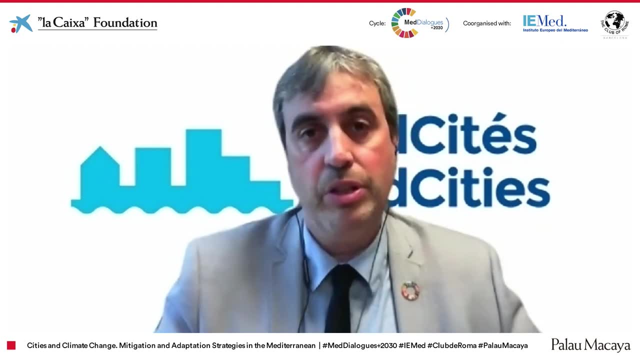 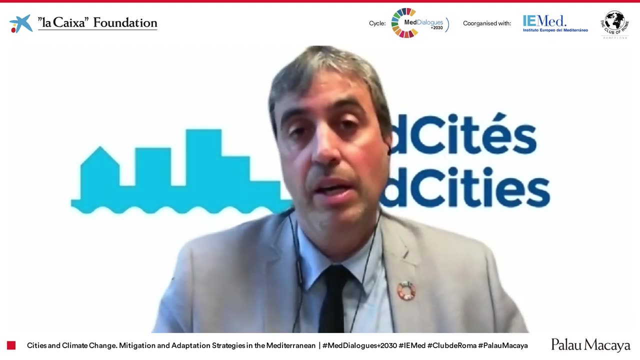 How they can relate with states, Because states are formulating the agendas. Agenda 2030, the new urban agenda, the European Green Deal are done, are conducted by states, But sometimes I have to say maybe not counting on cities. 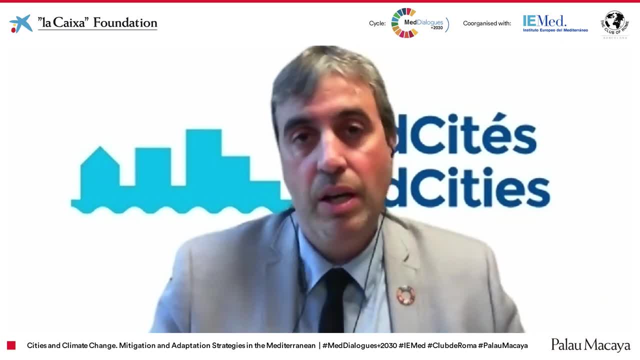 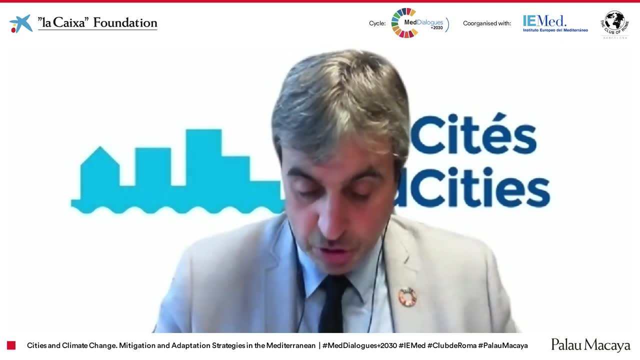 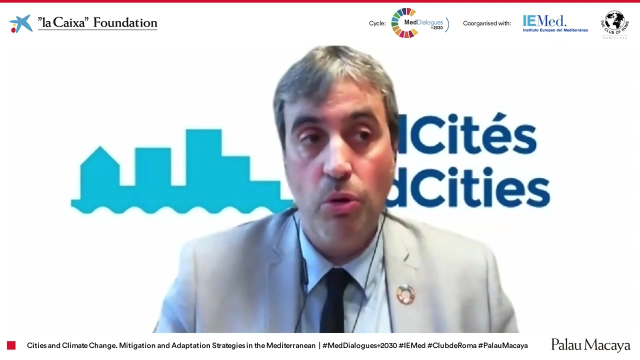 Which are, As I said, and you know, and they host the majority of the population of the world and in our region. So how we can help cities and local authorities to tackle that, How they can improve their capacities, Which is the space of cities to resolve, to solve these problems. 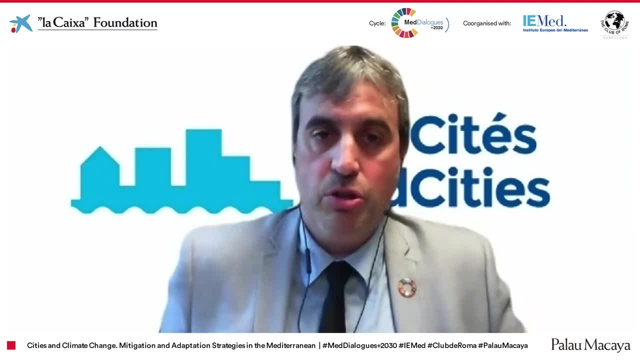 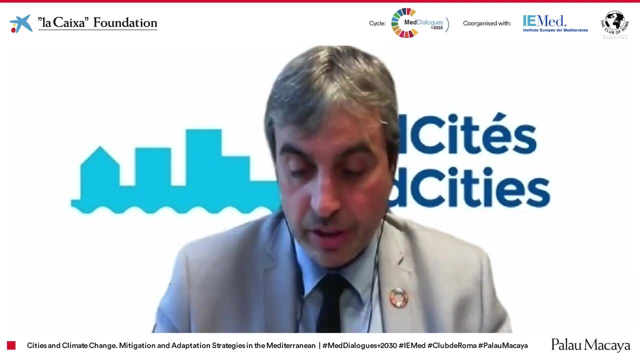 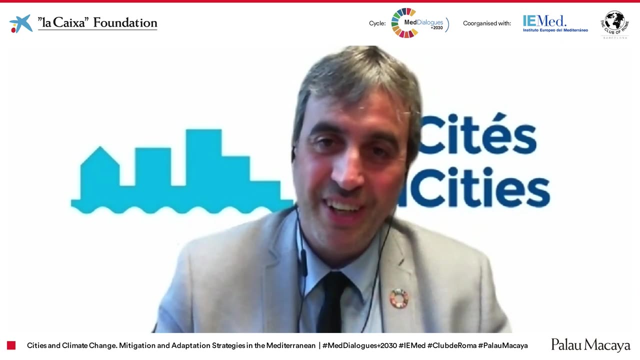 And how cities can improve, as I said, their capacities. This is something that we are doing in mid-cities, But these questions are on the table. We are wondering these questions, So maybe, maybe Mrs Hannah Alamuddin can put some light on these questions. 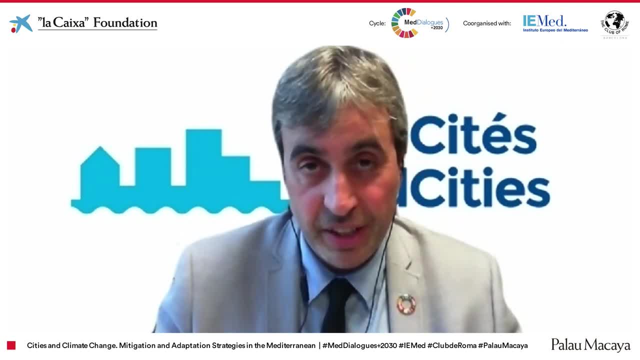 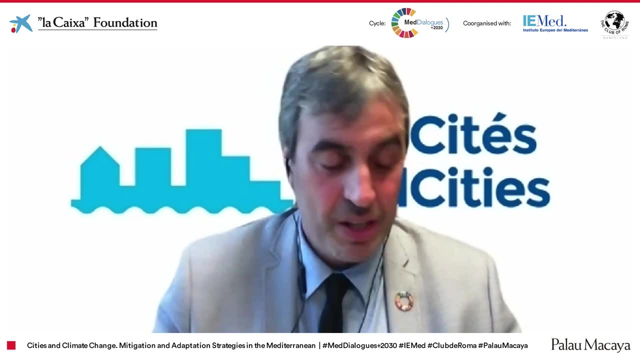 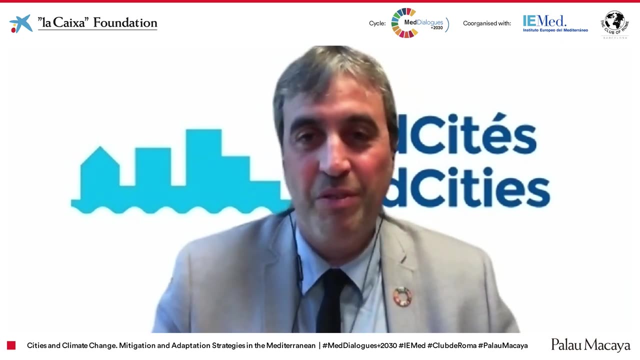 And on these maybe she can provide some answers to this. Of course, she has her own reflections That we are willing to hear, But we, as a network of cities, we need a lot of reflections. We need a lot of light also on how we can improve as a network. 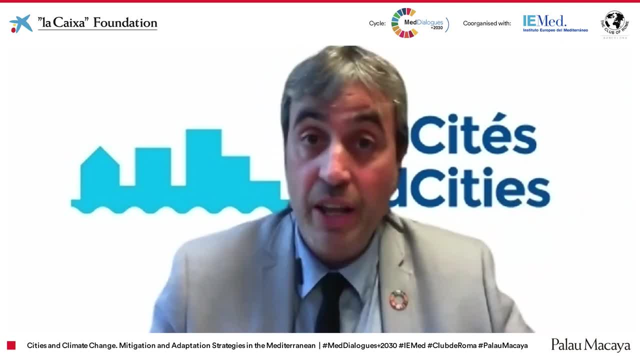 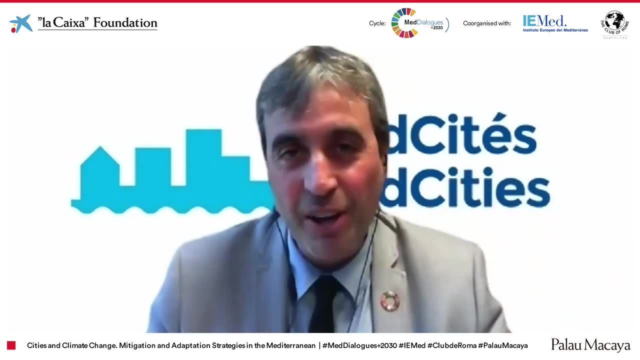 And one network that is also working with other networks. For example, in the Mediterranean Cooperation Alliance we are working with other networks, A network of networks. So we like a lot to cooperate, to share experiences. How Mrs Hannah Alamuddin can reflect on that? 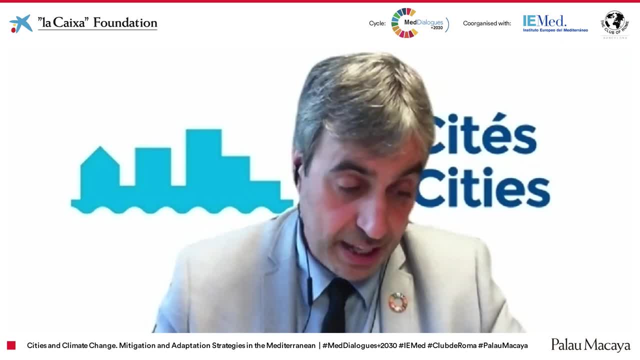 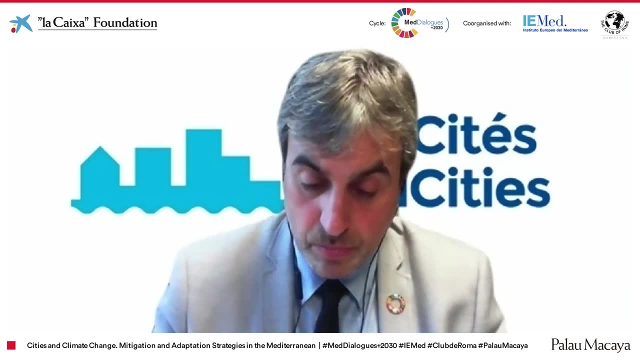 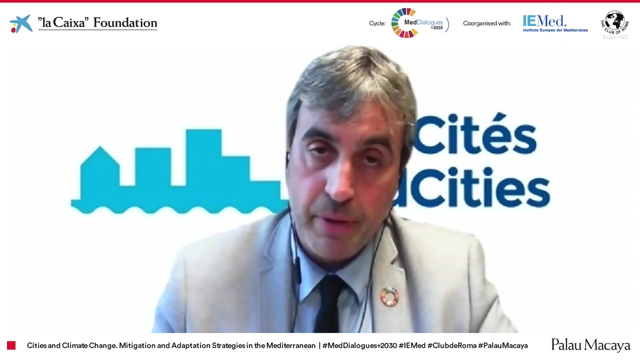 Mrs Hannah Alamuddin is a LEED accredited professional in sustainable neighborhood design. She has graduated from Greenwich University in the UK. She then went on to her Master of Science in Architectural Studies, In designing for Islamic societies, Which I think is a very differentiating approach. 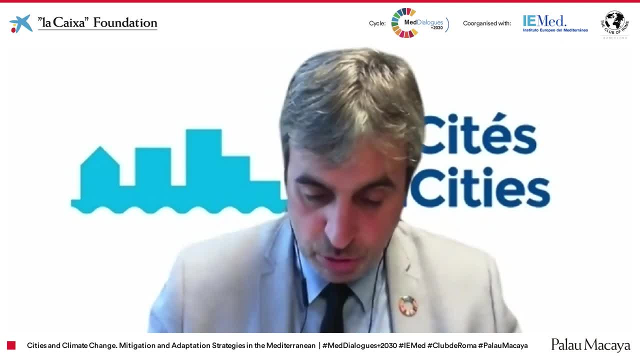 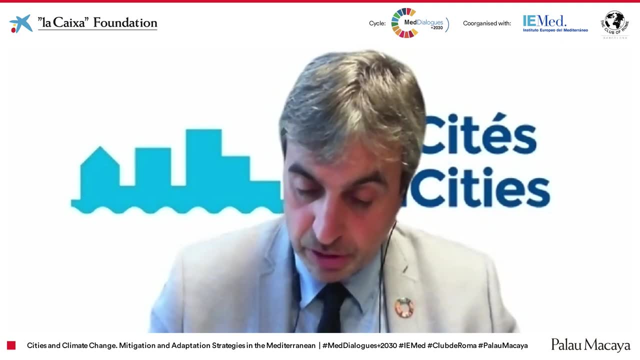 To what must be done to tackle these challenges. She started her practice in Lebanon And the practice Almi Maria Architects and Designers for Sustainable Development Works in architectural, urban design and landscape projects Within the perimeters of sustainable development. 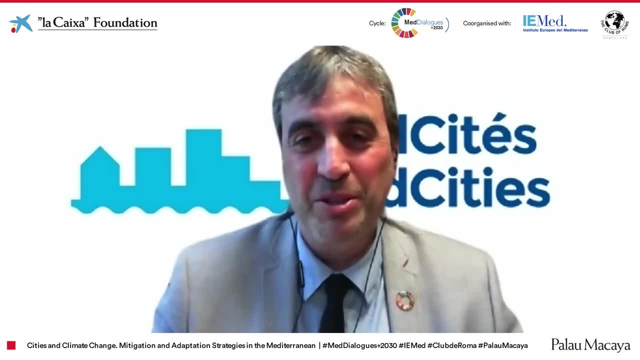 Which is celebrated a lot, I told you, Because me as a biologist And then I specialized as urban planner. I often witnessed biologists, often witnessed and stared at architects As someone that didn't like too much to protect the environment- But hopefully we have here a green architect- 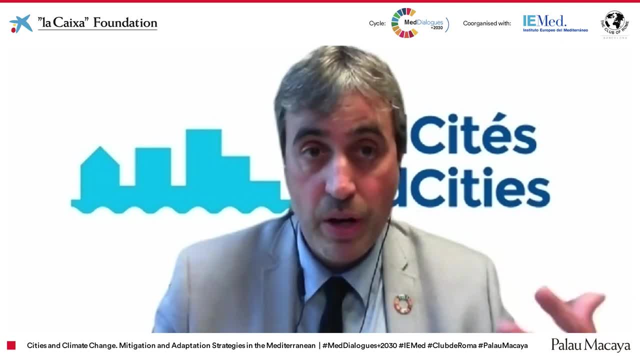 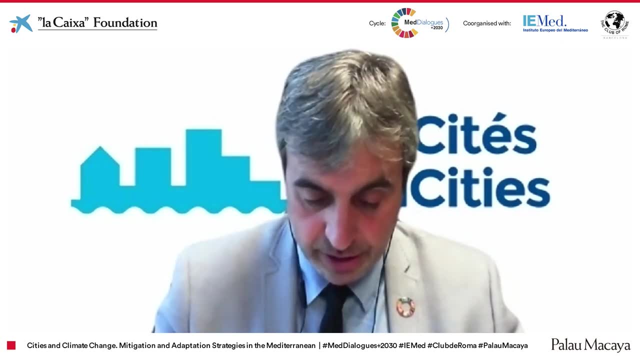 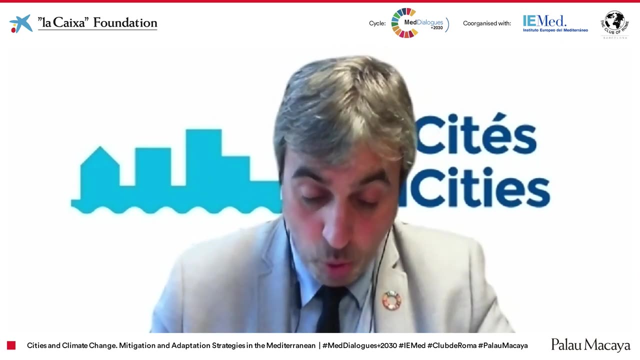 And a specialist with this vision, This vision of how developed cities and buildings With an ecosystemic approach, Which I personally celebrate. Mrs Alamuddin is also senior lecturer at the American University of Beirut And a board member of the Lebanon Green Building Council. 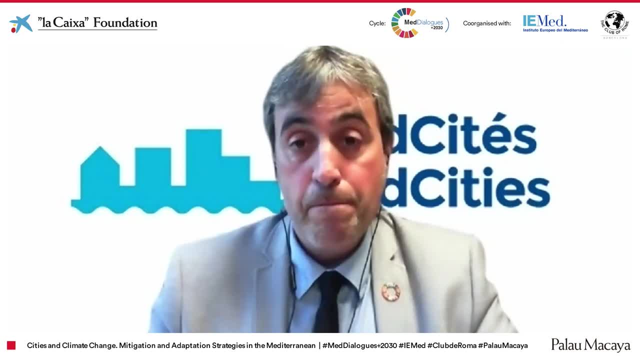 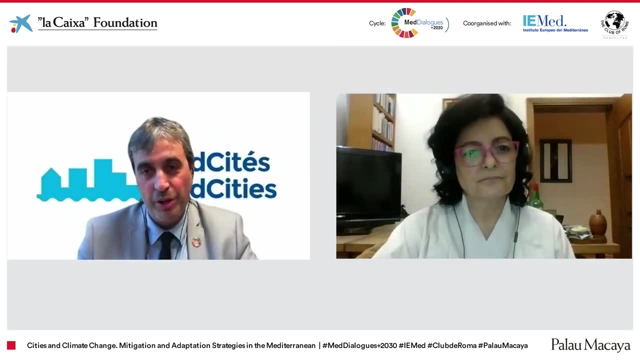 Which I also highlight a lot. Please, Hanna Alamuddin. Mrs Alamuddin, The floor is yours for 30 minutes. We are willing to hear you a lot. Thank you very much. Thank you very much for your invitation. 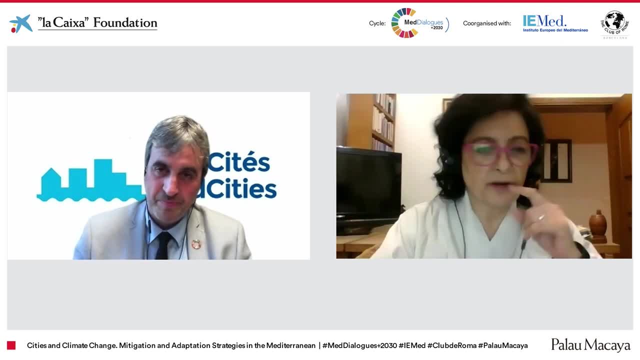 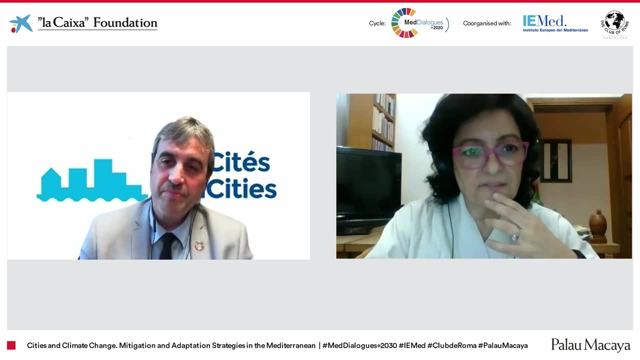 And the presentation. I just want to clarify a point. We in the 80s, when we did- when I did my masters at MIT- In designing for Islamic societies- It was the word sustainability was not there, So in a way it was really about being aware of the locality. 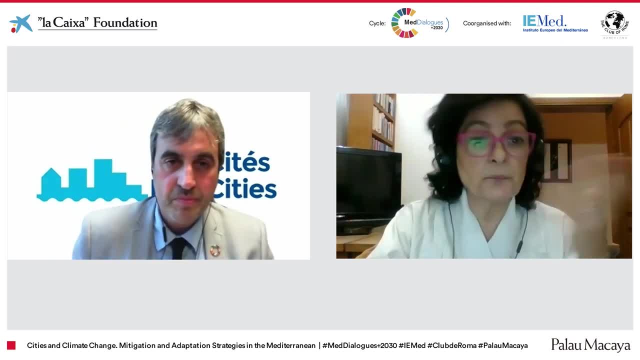 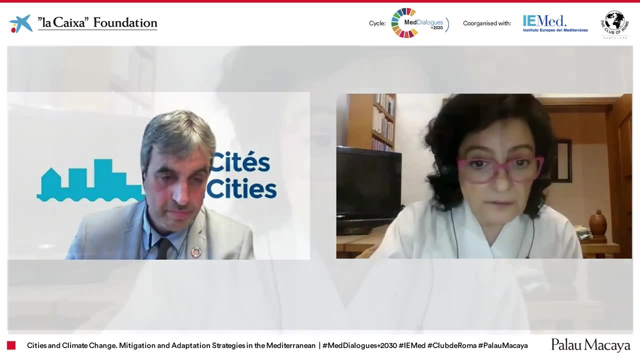 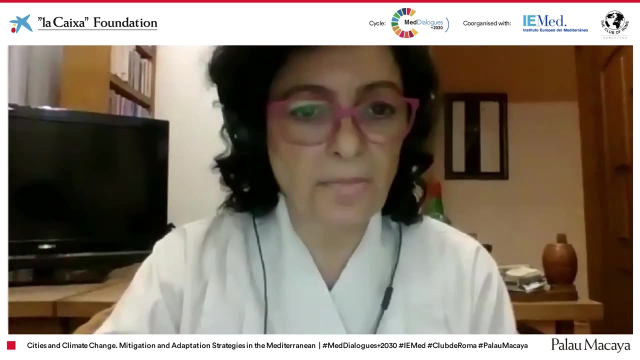 The context of the culture That is different from the European culture And architecture and development, Anyway, So I will share my screen now, Okay, Okay, Can you all see my screen? Yes, Yes, we can see it Okay. 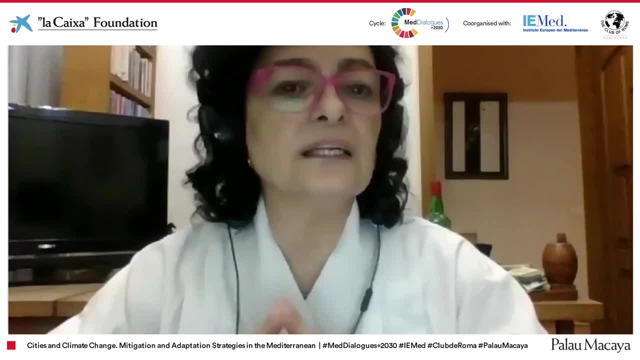 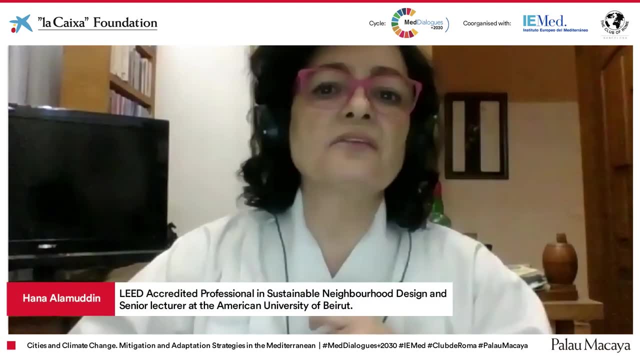 Good, Okay, Well, I wanted to start really from the basics And really look at what it is that we mean by strategic urban planning And, according to UN Habitat, It is a management tool that determines the direction in which an organization is moving. 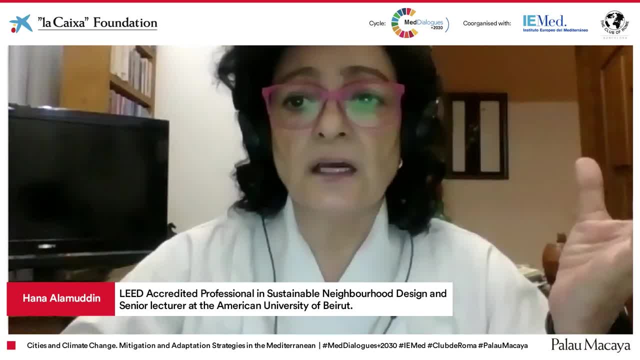 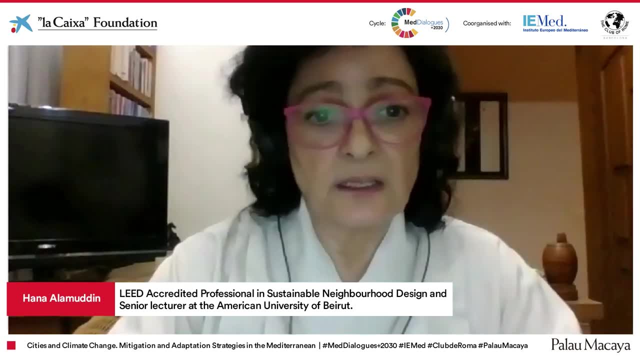 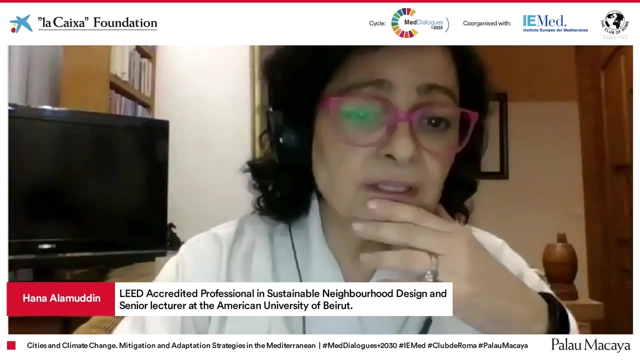 And how it will get there. The urban strategic And how it can get there. The urban strategic planning determines the direction of development Of a city Urban area In the context of its current profile And SWT SWOT analysis. It is oriented towards the future. 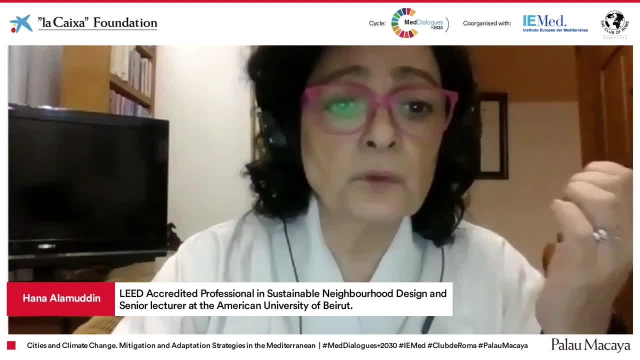 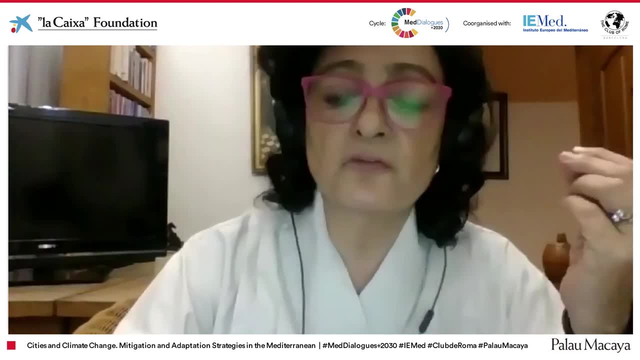 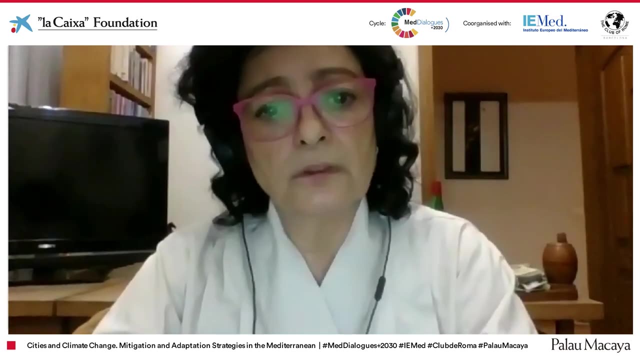 And this is quite important- Attempts to foresee how the world would be different five to ten years from now. It is aimed at setting the city's development direction based on what this future will look like, And here I would like to highlight a very important point. 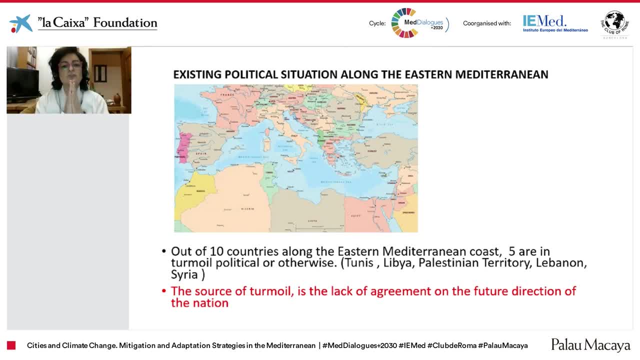 Which is the existing political situation in the eastern Mediterranean, which is where we are, Well, where I am. If we look at the countries on the eastern Mediterranean, which are about ten, Five of them are not Four for sure, But five are in turmoil. 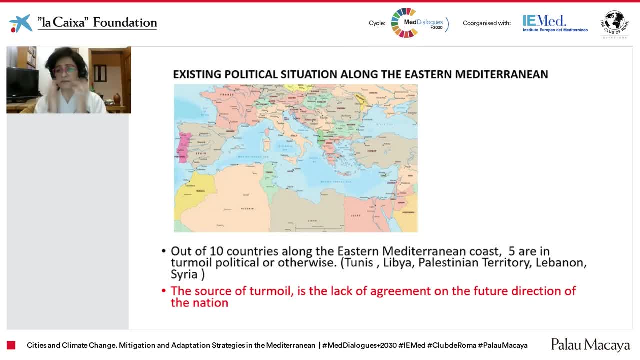 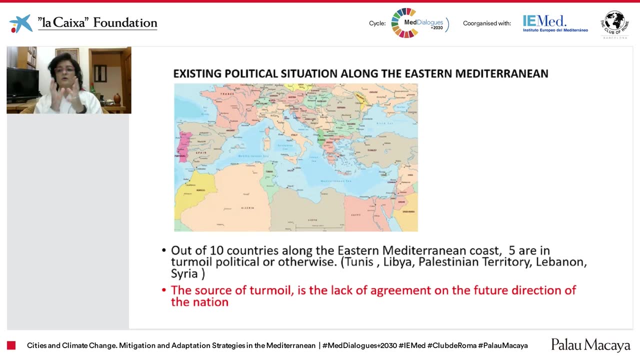 Whether it is wars, Whether it is political unrest, Economic unrest, Etc. Now one could argue that the source of this turmoil is actually the lack of agreement on the future direction of the nation. So this is where this issue needs to be thought about. 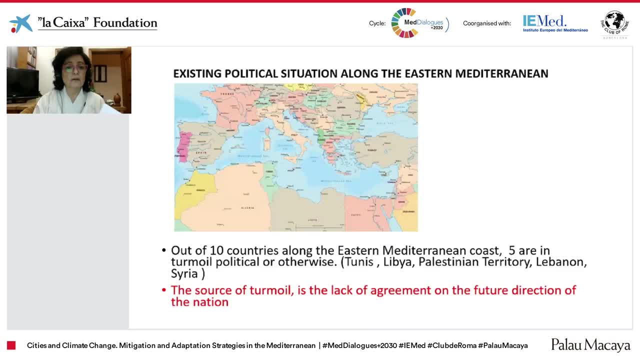 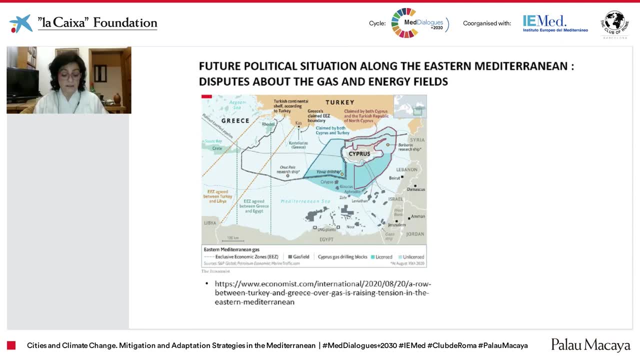 Within this context. Now, unfortunately, if we look at the future, then again, the prospect of peace in the region is also under question, with the discovery of gas fields and the rising tensions and disputes about this issue. The point here is that, in conditions of turmoil, government concerns are related to survival, safety and security. 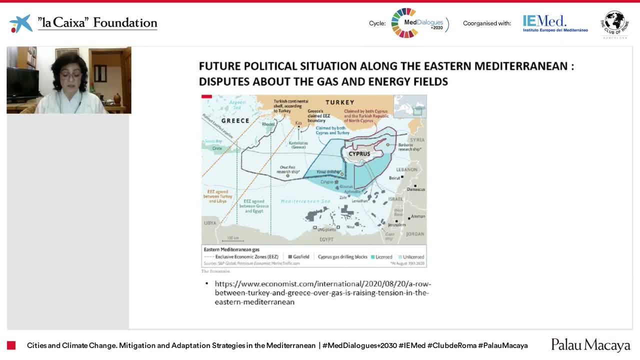 Moreover, conflicts result in the loss of expertise and know-how that leave the countries and government bodies understaffed and unable to function properly. My presentation will focus on Lebanon, Not just because I know it well, but because I believe that there is an interesting message to be heard. 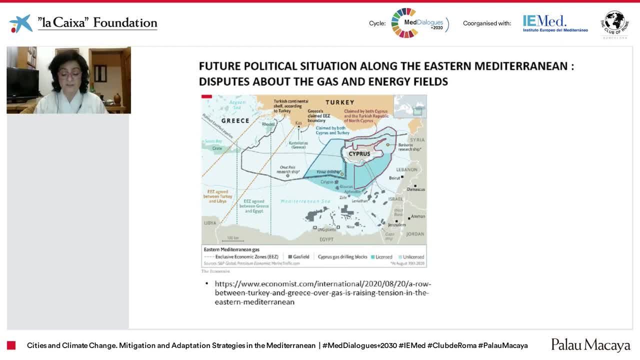 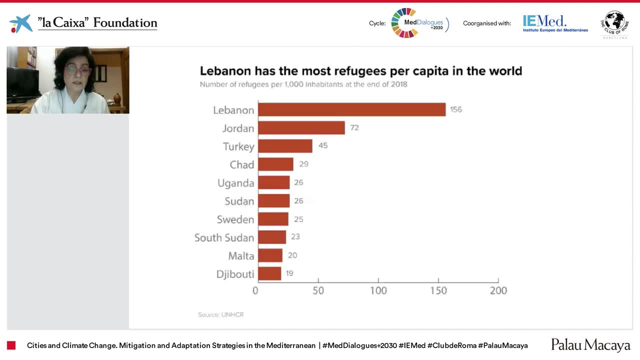 And as it is your worst nightmare scenario for litigations, And as it is your worst nightmare scenario for litigation, And as it is your worst nightmare scenario for litigation, And as it is your worst nightmare scenario for litigation. So today we are going to be talking about the 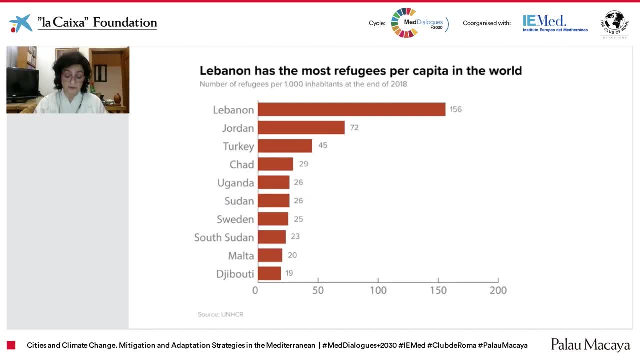 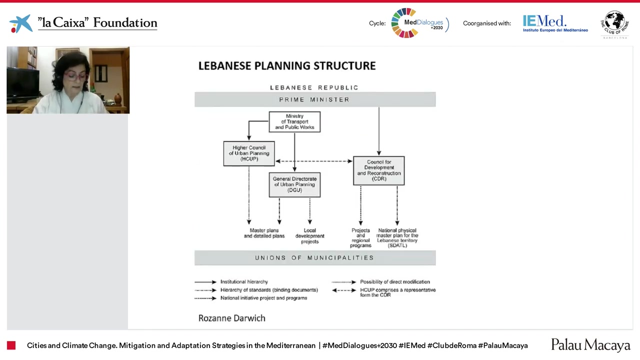 climate change. Now, according to the New And habitat, Lebanon is highly organized: an overall population of approximately 6.8, making it the country with the highest number of Syrian refugees per capita in the world. As for climate change, we know that the actual source of greenhouse emissions are energy. 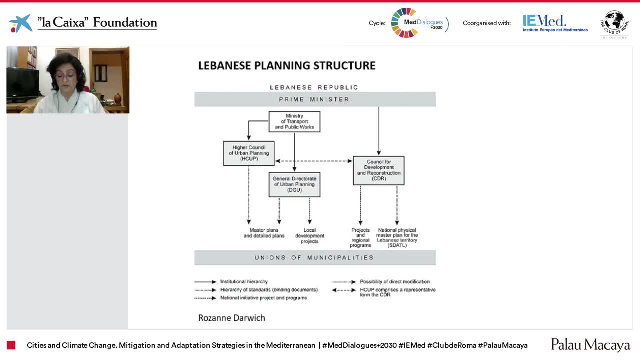 production, transport, waste, landfills, agriculture and deforestation- all sectors requiring a clear long-term vision roadmap and administrative tools and funding to be able to succeed. If we look at the planning structure in Lebanon, we find that, as far as the administrative 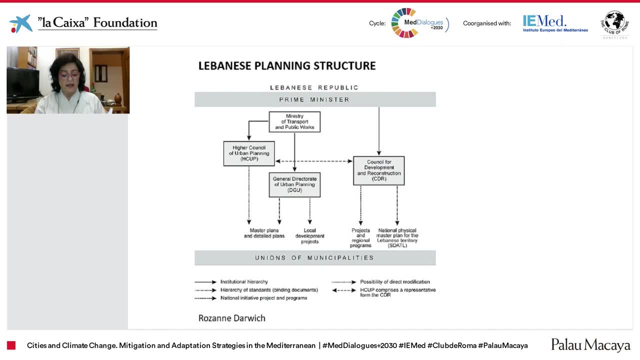 tools are concerned, planning is very centralized. It is dealt with at various levels by the following bodies. We look at the Higher Council of Urbanism. It is formed from different ministries and specialists and they are responsible for recommending and guiding the urban planning at the national scale. 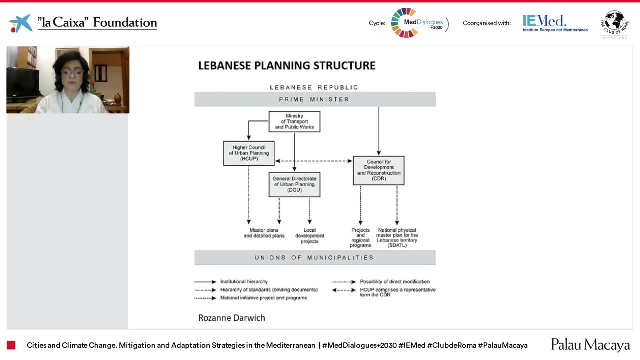 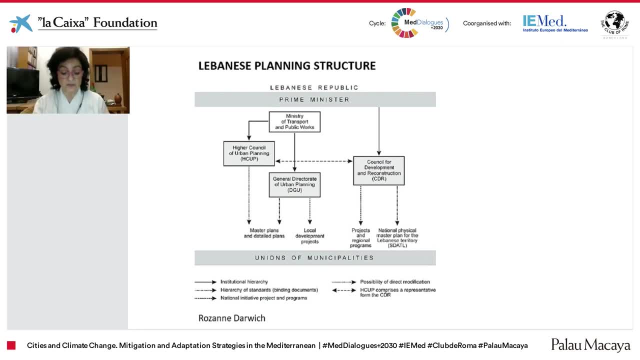 They are responsible for developing and reviewing master plans all over Lebanon. The CDR was created for the reconstruction of the country, separate from the ministries, and they regulate- supposed to regulate- urban growth through a national physical master plan, which is really just a guiding framework. 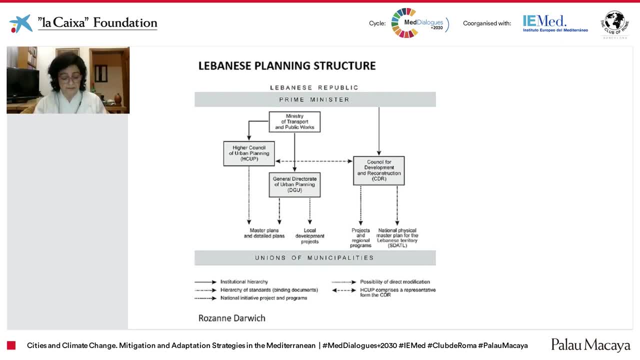 Now for the municipalities. municipalities in Lebanon number 1,038, and the majority of them have less than 4,000 residents. Now the municipalities have responsibility over planning, including water, wastewater, urban management, economic, social development and environmental protection. 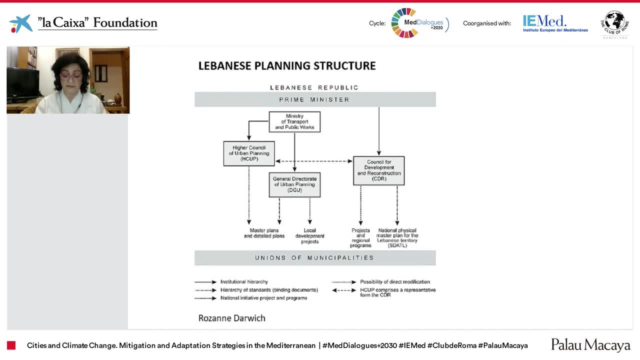 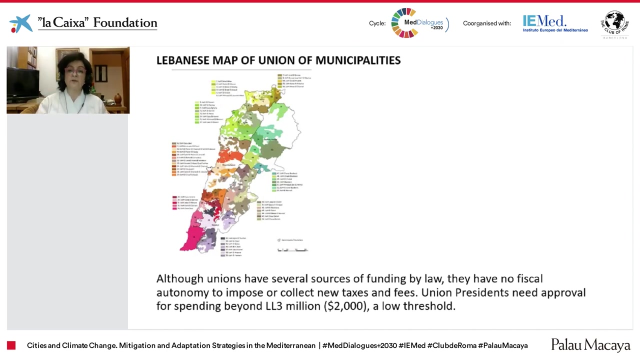 But the majority of municipalities lack the administrative and fiscal capacity to carry out the project. Furthermore, when we consider these sectors that we just mentioned, they tend to span much larger than municipal boundaries. Therefore, since the installment or the re-installment of municipal elections in 1998, there was a 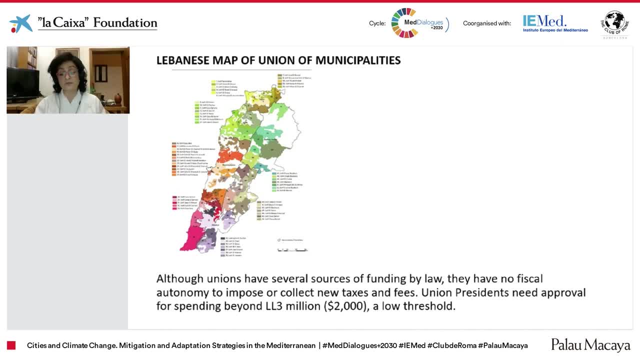 rise in the formulation of what we know as municipal unions. So from 1990, they were 13,. they rose up to 53 in 2016.. This is a very important shift. It allows the efficient planning as they can relate to the local communities but have 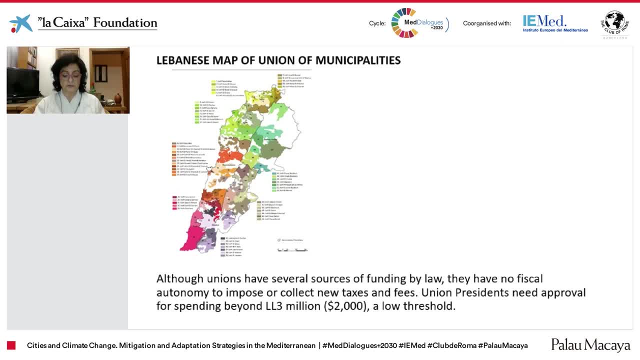 new tools and capabilities, such as observatories for strategic planning and access to donors. However, the union of municipalities still lack independence from the central government and ministries and they cannot access funds from the government And Um. Although they are a move in the right direction, they really need to be developed further. 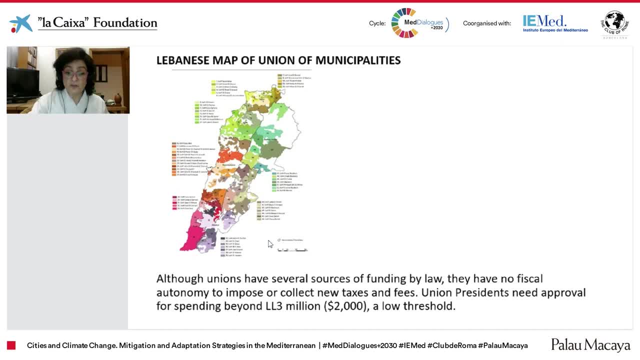 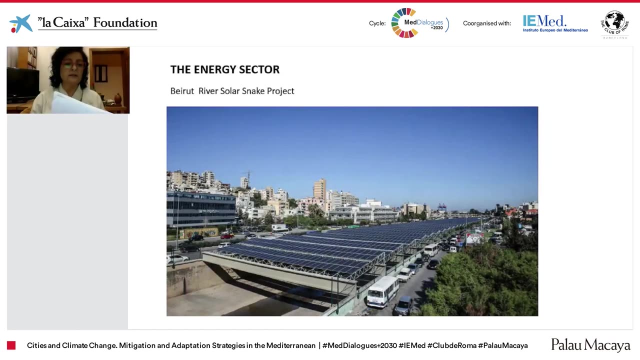 As you can see here, they have no fiscal autonomy to impose or collect new fees. Now, the second layer that I will be dealing with or looking at is really the energy sector. So we looked at the administration And we saw that the planning is moving sort of in the right direction, but it lacks autonomy. 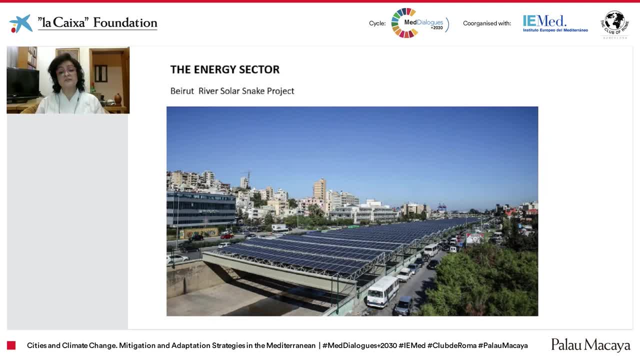 still Now. our next phase is the energy sector, And this is highly again centralized In 2009,. at the Conference of Parties to the United Nations Framework Convention on Climate Change, the Lebanese government committed to increase the share of renewables of the 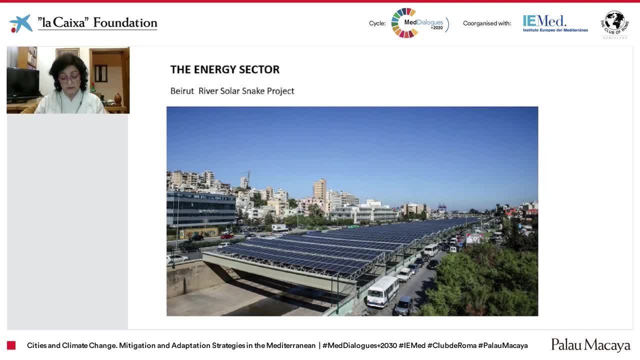 projected total electricity and heat demand in 2020 to 12%. What we see in front of us is the Beirut River solar snake project. This was the first step towards that goal, And a call for expressions of interest was launched in April 2013 by the Lebanese Ministry. 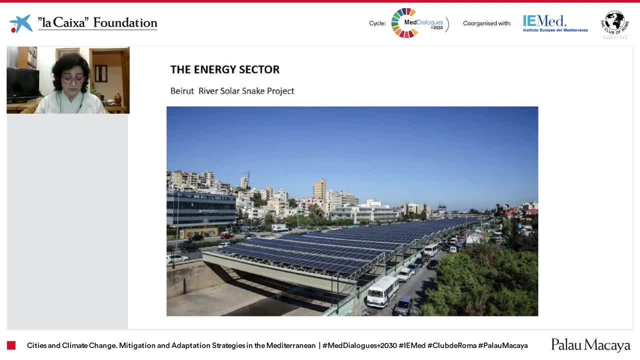 of Energy and Water. Now, the Beirut River was the largest body of water in the city. It originated in Mount Lebanon. Its waters were directed to the city via aqueducts and rivers. Since the time of the Romans, The river flourished as a riparian landscape and a social space for the city until 1968,. 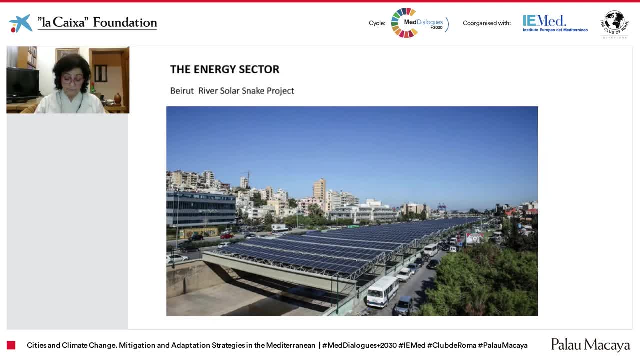 when it was transformed into a concrete canal to control its flooding of the neighborhoods that grew next to it due to urban growth. This transformed it into an industrial waste waterway and sewer, posing numerous health risks to the neighbors. The Beirut River solar snake made use of the space over the canal to install a photovoltaic. 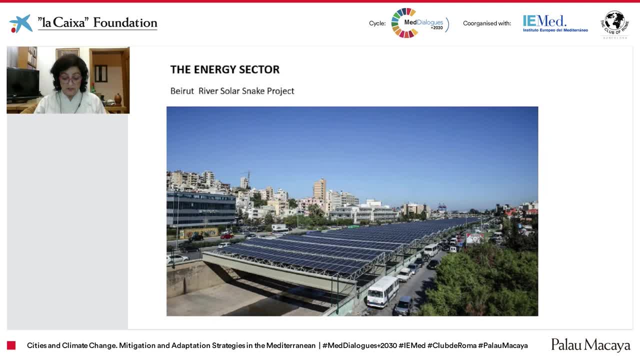 farm in the middle of the city. This ingenious idea provided clean energy to the main power company of the nation. Planned in several phases, the first phase of peak capacity of one megawatt was connected to the grid in September 2015.. Now the project consists of 3,600 polycrystalline PV panels of 300-watt peak tilt angle: 10%. 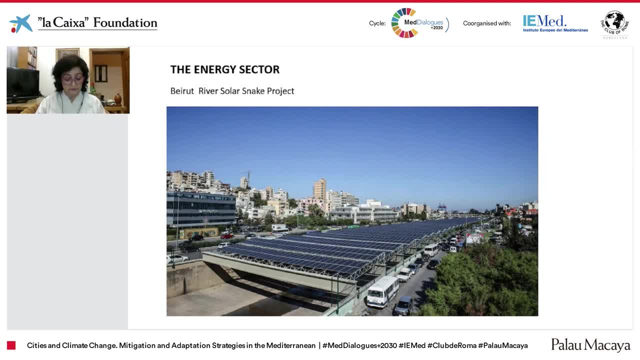 spanning 31 concrete beams above the Beirut River. It actually generated 5,427 megawatt-hours of electricity until June 2015.. The project further reduced around 4.5 kilotons of carbon dioxide, based on a grid emission factor of 0.56 kilotons, and saved about $900,000.. 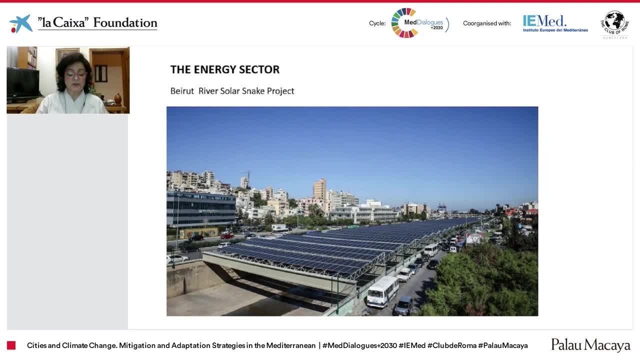 In 2019, this project won the prestigious Environmental Energy Global Award under the National Catechism, competing with more than 2,500 people. Moreover, this project played a very important role in raising awareness of clean energy and sources. Unfortunately, other projects planned by the Ministry of Energy and Water with a public-private 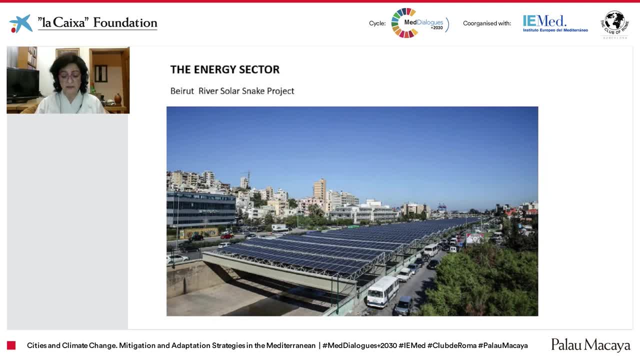 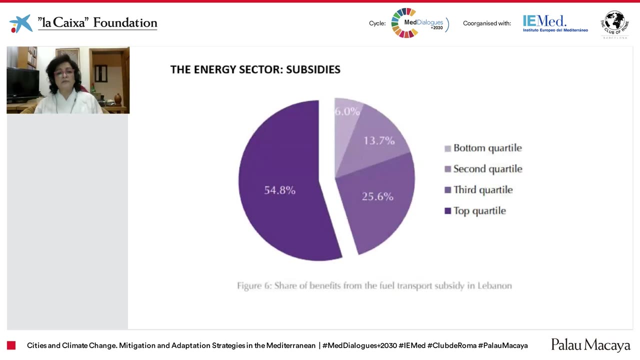 partnership, such as the solar farm in Zahrani, were implemented, But some unfortunately failed. They were not like the wind farm of Akkar, because of the economic meltdown. However, in a way, the economic meltdown was itself a mitigating factor for climate change. 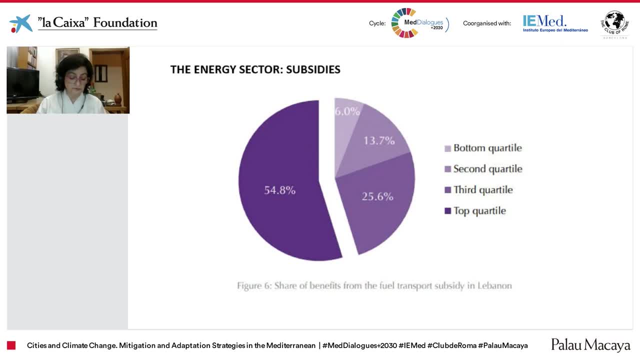 as the subsidies on fuel had to be lifted by the government due to the sharp depreciation of the local currency versus the dollar, And according to a study by the Ministry of the Environment and the UNDP in 2013,, the fuel subsidies were found to be $3.1 billion, ie 7% of the country's GDP. 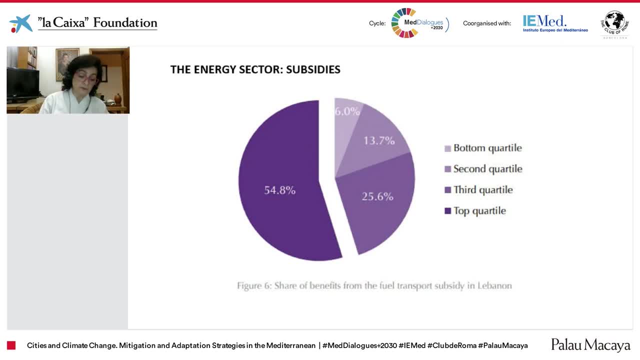 Now, while aimed to help the poorer section of the population, we can see that it was found to benefit higher-income households and actually increased energy consumption and enhanced global warming. Furthermore, the lack of central electricity and the lack of energy consumption was a 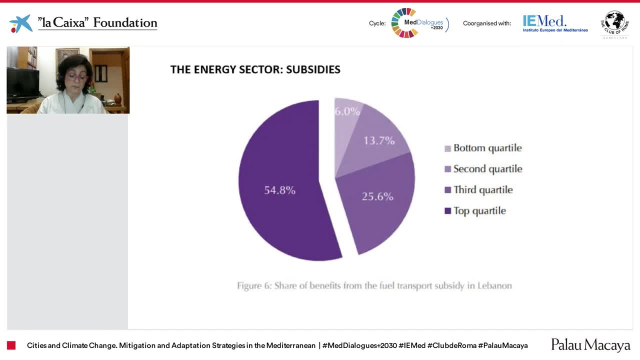 key factor in the development of electricity. The lack of central electricity meant that neighborhood generators installed as a backup for the central electricity have become the main source of energy for households today, with their owners applying higher and higher tariffs and virtually no control over the air pollution. 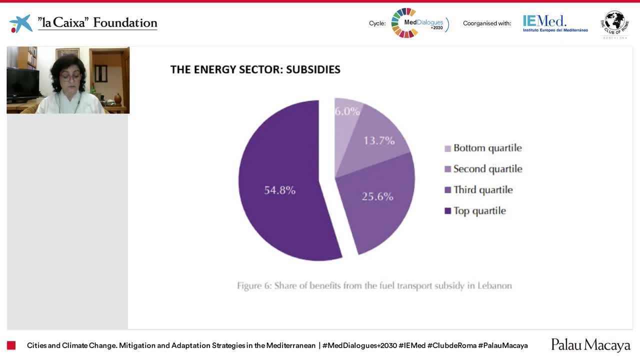 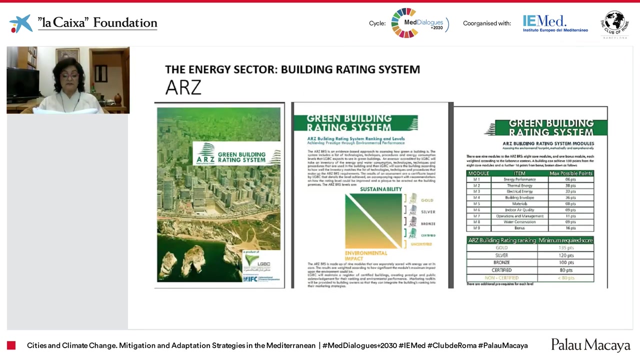 This has also brought to light the issue of energy consumption, with an increase in the installation of photovoltaic solar panels on roofs, especially for institutional use. So, in a way, the economic meltdown raised a lot of issues and questions. Another mitigating global warming factor is through green buildings. 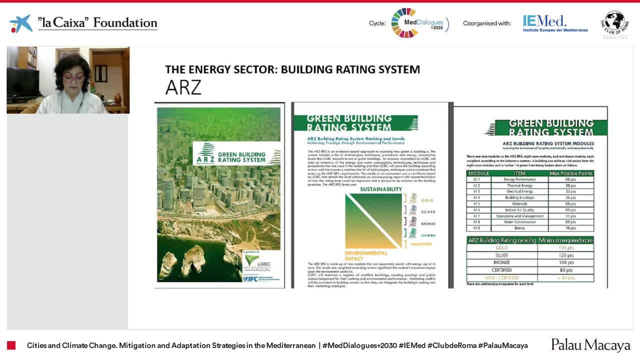 However, Lebanon, like other southern countries, the criteria used by international bodies like LEED and BREEAM and others tend to be difficult to comply with. the criteria used by international bodies like LEED and BREEAM and others tend to be difficult to comply. 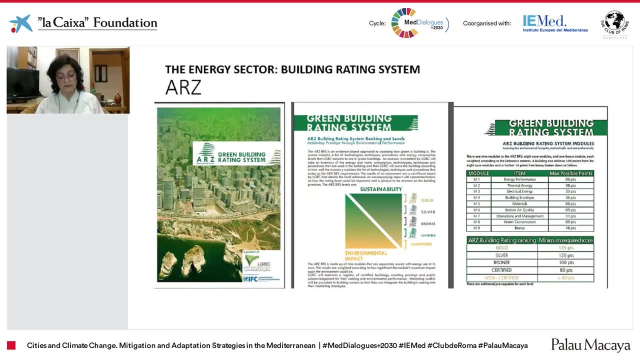 by international bodies like LEED and BREEAM and others tend to be difficult to comply with, related to existing commercial properties. The rating system is designed to measure the extent to which existing commercial buildings in Lebanon are healthy, comfortable places for working, consuming the right amount of energy and water, while having a low impact upon the natural. 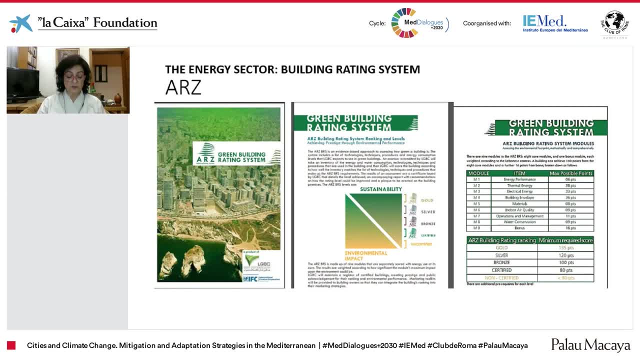 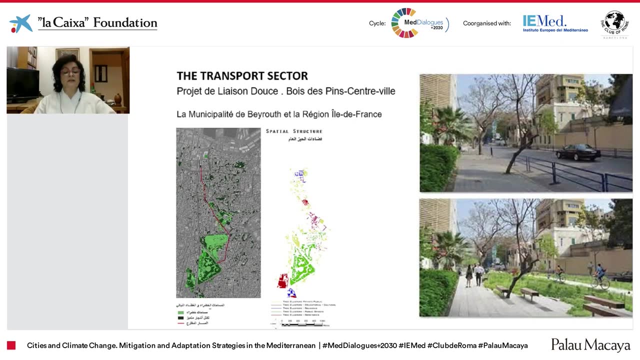 environment. Today, we have five projects that have been certified, with three in the pipeline Now. another main source of greenhouse gas emissions is, of course, transport. Now, although Lebanon was one of the first countries in the region to have a railway, 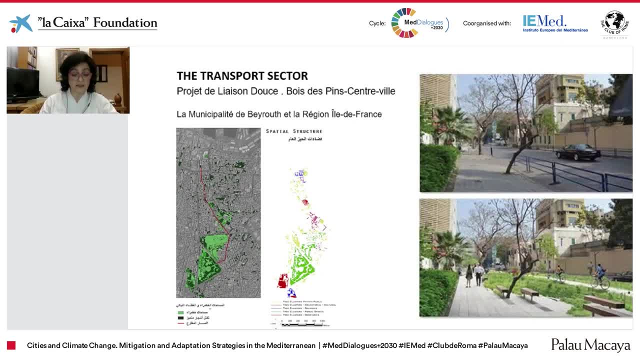 built in 1895 with a network of 40 stations connecting 200 kilometers. the system was badly damaged during the civil war and has not been reinstated since. Meanwhile, the average gas emissions in Lebanon are about 1.5 billion. The average gas emissions in Lebanon are about 1.5 billion. 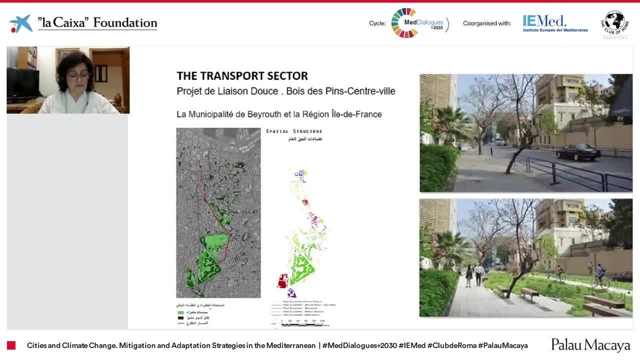 The average time the Lebanese spends commuting across the city is three hours per day. This means that 16% of a person's production time is spent commuting, at the cost of $2 billion each year. The main cause for this loss is related to the lack of organized public transport. 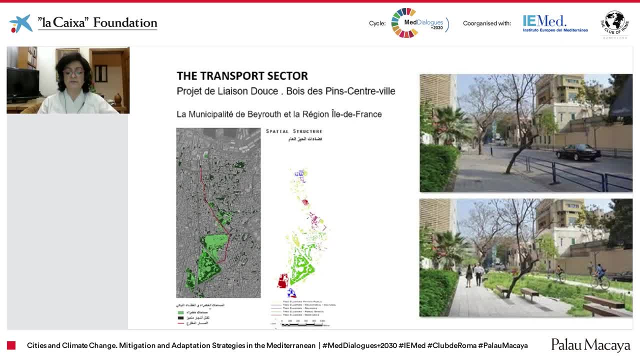 the bad condition of the roads and the rise in the number of privately owned cars. The rise averaged a yearly increase of 13% between 2007 and 2016.. Now, over the years, many proposals and studies were done. looking at a metro station which is 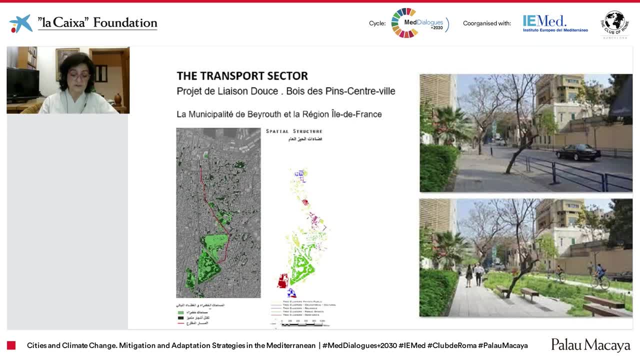 problematic in Beirut because of the archaeology of the city, the re-instatement of the train, tramways, bus system, etc. including a master plan by the Ministry of Public Works and Transport and transport. However, this plan was deemed not economically viable in the short term. 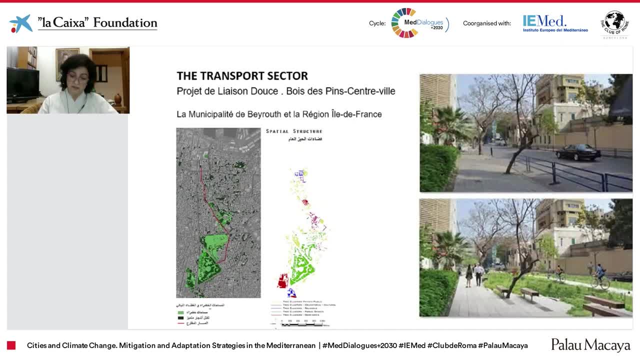 because of several obstacles facing the government, such as political tension, social unrest and the refugee crisis. It is estimated that 70 percent of cars in the city come from outside. Therefore, the most feasible plan was for a rapid bus transport link, presented in 2018. 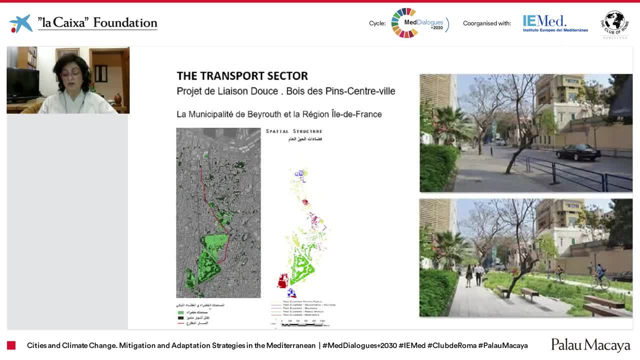 and accepted for funding by the World Bank at the cost of 295 million dollars. However, here again, the Lebanese government requested that the money be relocated to finance the cash subsidy cards to accompany the lifting of subsidies, And it looks as if the World Bank is willing to consider the redirection of the loan. 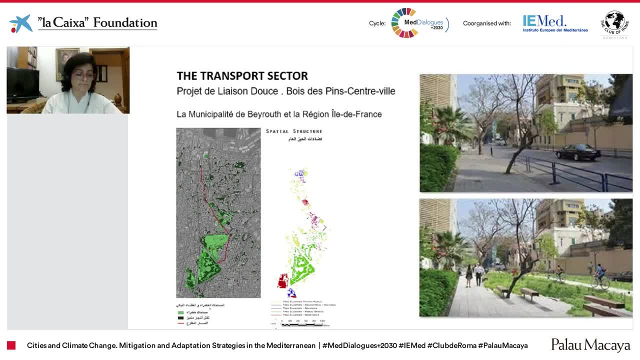 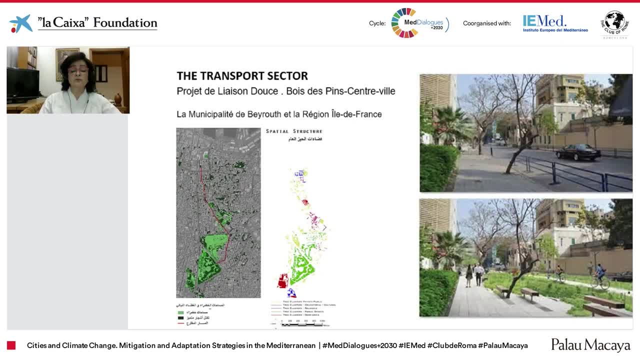 the World Bank. It was funded by the World Bank. It was funded by the World Bank, It was funded by the Ile-de-France and it's called the Liaison Douce project. The idea behind the project is to provide the citizens of the city with a green corridor of public space, pedestrian and cycling. 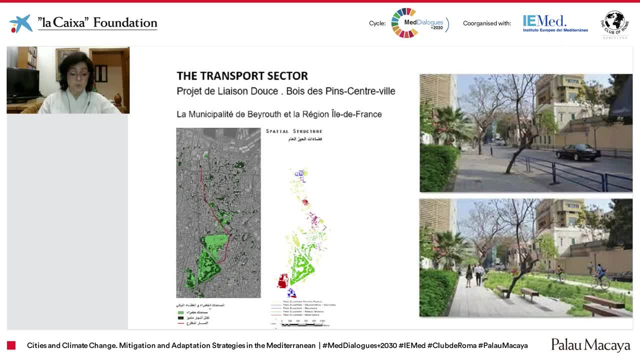 paths linking two iconic sites: the Voile du Thin fine forest of Beirut and the center of the city along the Damascus road. The study was designed by planner Habib Debbis and preserved with Haber Nadj. just a high-quality linear urban park, but a provision for alternative means of transport. 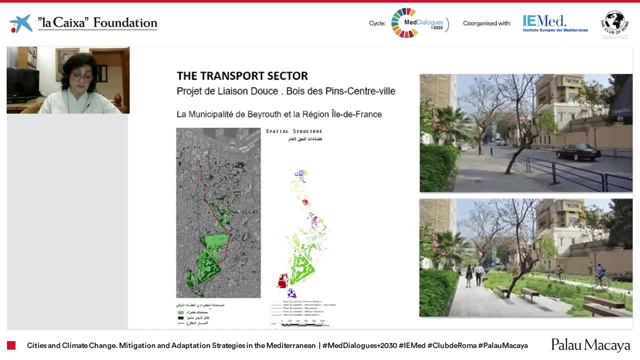 cycling and walking. The added value of the project is that it follows the Green Line, which is the zone that separated east from west Beirut during the civil war. Thus, the project will also act as a link between the communities on either side of the Green. 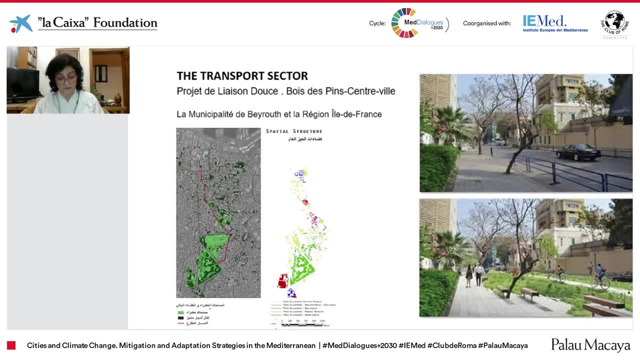 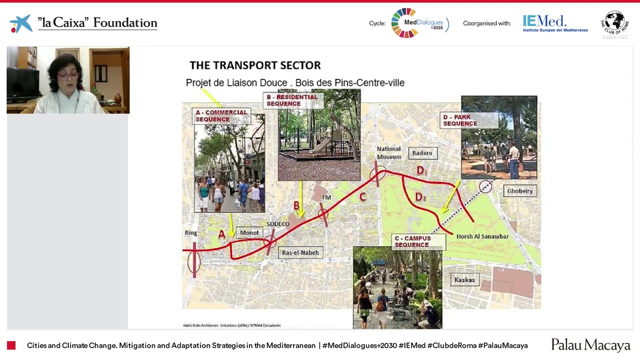 Line and link the heart of the city to the edges. The study was done and submitted to the municipality in 2011 and has since stayed in the drawers When the president of the Ile-de-France- you can see here the different public spaces that it provided- but the president of the Ile-de-France. 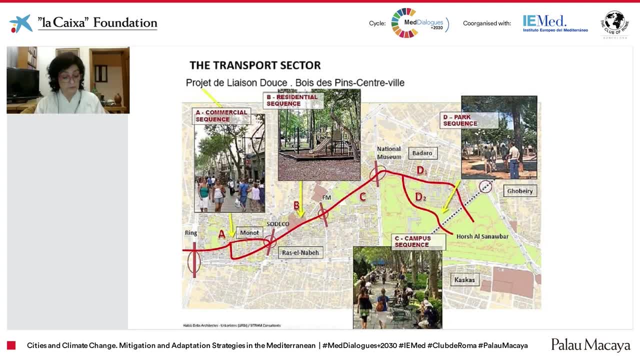 Madame Valérie Descrez visited Beirut. She welcomed the invitation of the President of the Ile-de-France visited Beirut and inquired about the study and why it did not get implemented by the municipality as originally agreed. She was informed that the study requires approval. 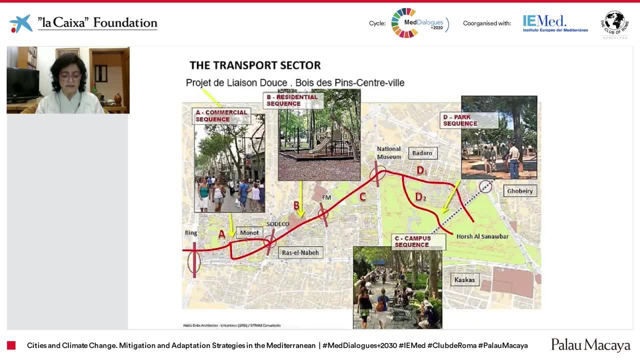 from various ministries and is stuck in the bureaucracy of the system. As far as Habib Dibs is concerned, he says public projects in Lebanon are not for the public good but for the authorities to make money, And this project obviously was not financially of use to them. 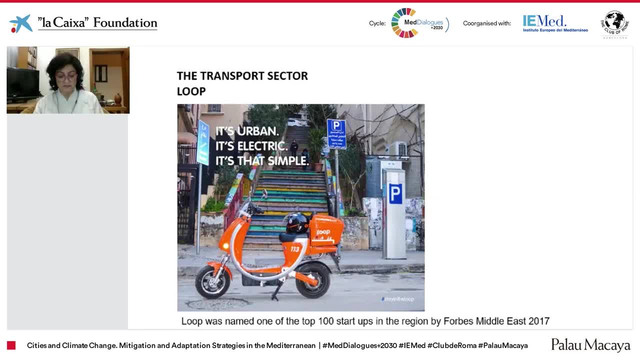 On the other hand, a private venture startup of smart electric scooters was started in 2016 in Beirut. Loop was set up by a group of highly skilled professionals in telematics, fleet management, logistics and market development to offer the service for the first time. 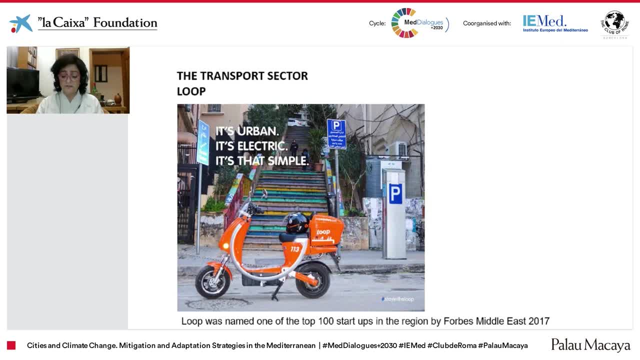 in the Middle East, starting with Lebanon. This app-based service operates a fleet of smart electric scooters and charging stations, making commuting in the congested city efficient and clean. The philosophy of the firm is: as part of the sharing economy, we believe that the future of transport 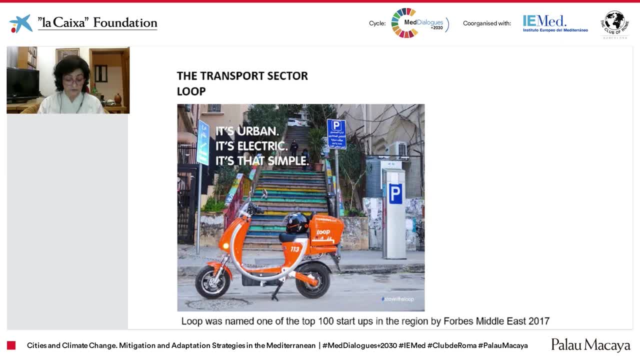 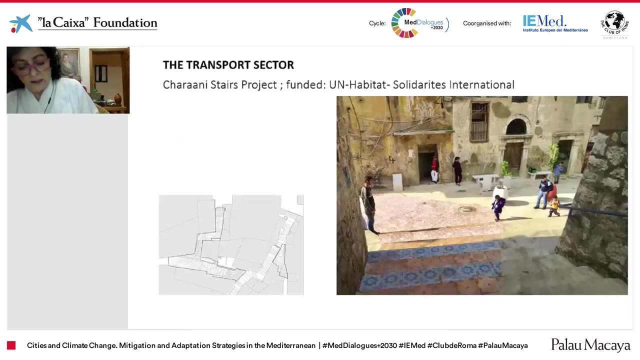 is based on access instead of ownership. Loop was named one of the top 100 startups in the region by Forbes Middle East 2017.. Another small-scale project which is very interesting is the rehabilitation of the Shaharani Stairs in Tripoli. 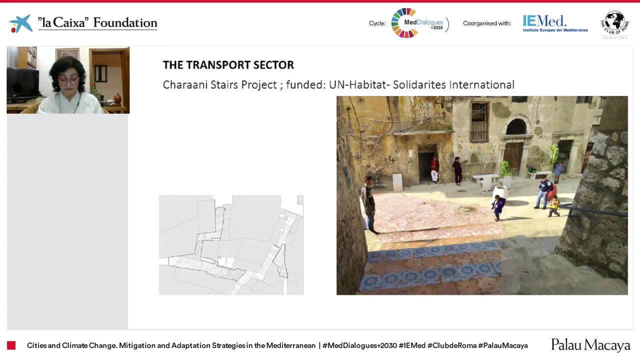 The project was funded by UN, Habitat and Solidarites International and was designed by Emergent, the National Architecture Ava Studio. The rehabilitation of the Shaharani Stairs is a project that is about public space and located in Tadbe, a low-income neighborhood in Tripoli. 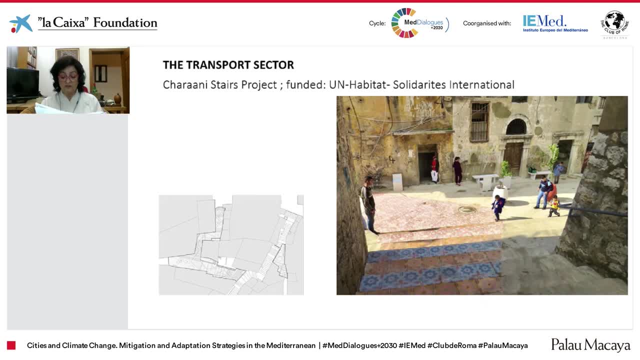 The project was about rehabilitating the stairs, as they are vulnerable to flooding and other issues, but are also the main access of the neighborhood to the historic center of Tripoli and its souks. The project is also about social integration, as 15% of the community are senior refugees. 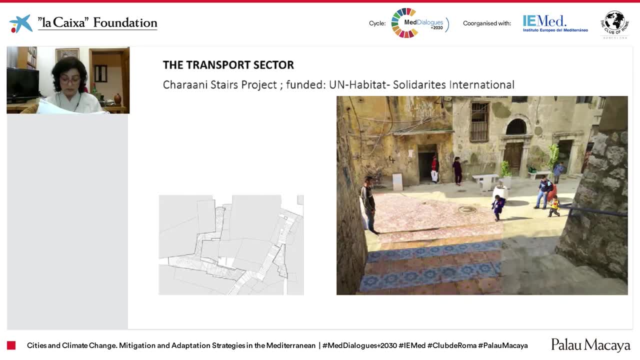 and it's about post-conflict recovery, as the stairs are located near an area that so clashes between two neighborhoods of different sectarian profiles: Jabal Mohsen and Tadbe. Focus groups were formed to engage the communities and to hear their concerns and needs. 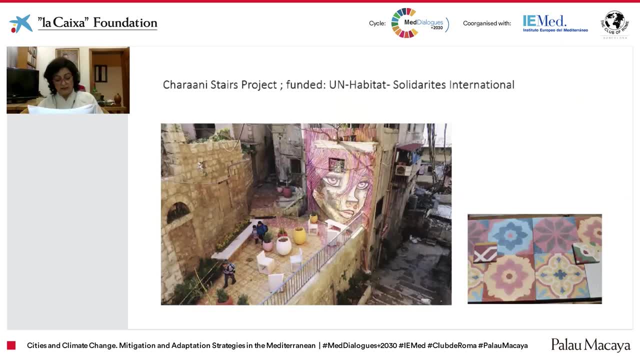 and, And we see that the material used for the stairs were locally manufactured acoustic tiles and the mural that we see was designed in collaboration with the local artist, Alfred Badr, and represents a local girl that was killed at 11.. Of course, all this was done after fully coordinating. 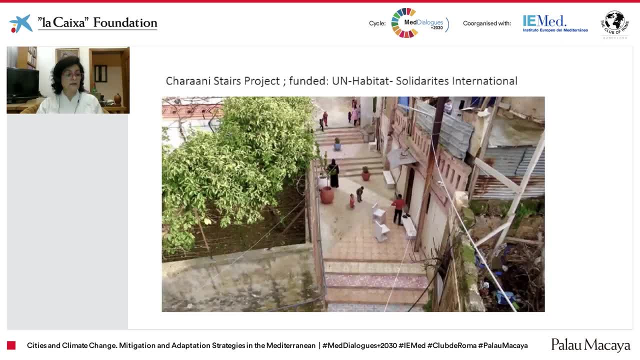 with her family. Now both the tile work and the mural were appreciated by the community and the space is now being used as morning gathering spaces and routes to the city. The inclusion of lemon trees refer to the city's historic citrus industry. That is common. 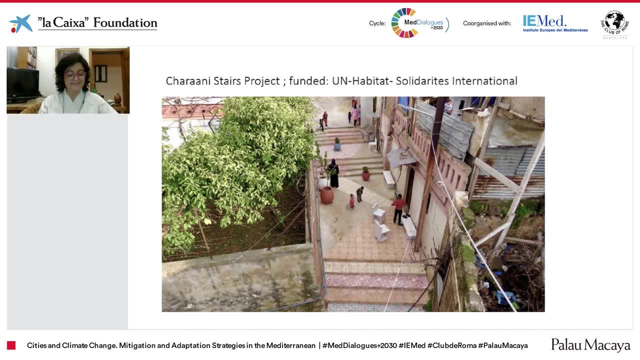 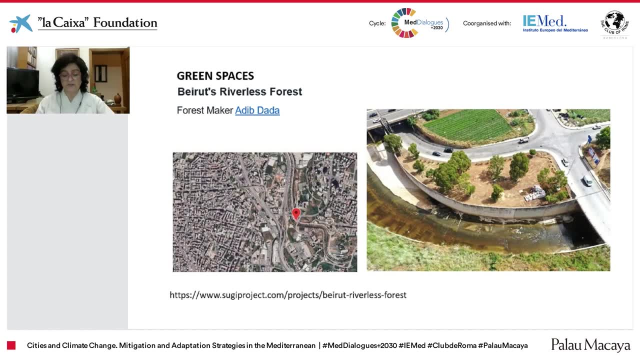 You can see them. They're very small, unfortunately, in this slide Now. a good tool for mitigating climate change is green space. I think we all agree Now. Beirut has 0.8 square meters of green space per capita. 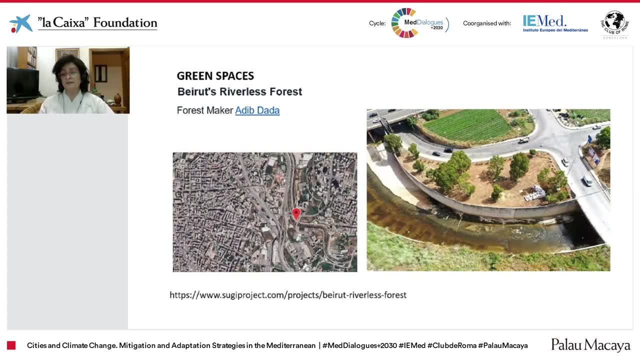 versus the nine square meters per capita recommended by the WHO. Now, going back to the Beirut River, an initiative by the firm The Other Dada, who are a regenerative architecture and consultancy firm led by Adib Dada, had been conducting extensive research on the Beirut River. 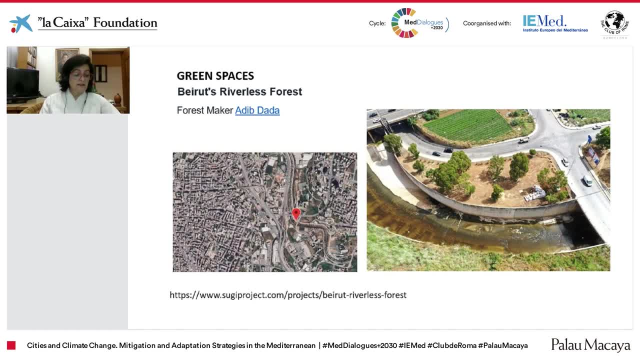 and its neighboring areas. As we said, the area was a rich riparian environment and was a backdrop of many cultural events, such as the Armenian Water Festival, Vardabar and the Muslim Heath, Now, unfortunately, faced with complete disinterest. 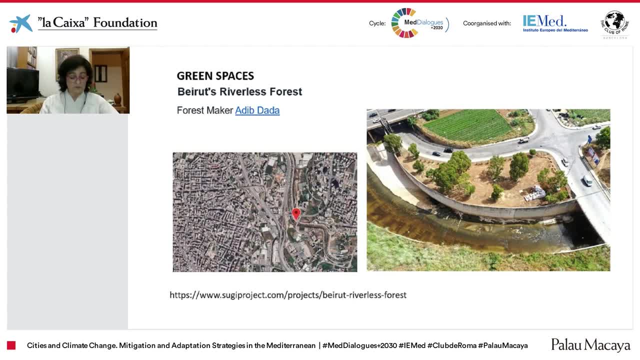 for ministries and institutions responsible for the Beirut River. The consultant decided to go to a more concrete, simpler project: Emiyaki Forest. Emiyawaki Forest, the first in Lebanon. With this, he approached the mayor of Saint Delphine. 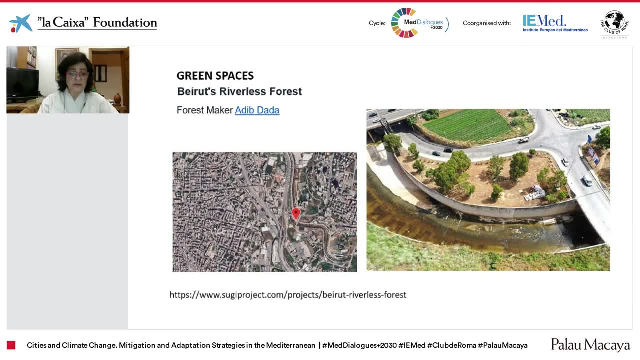 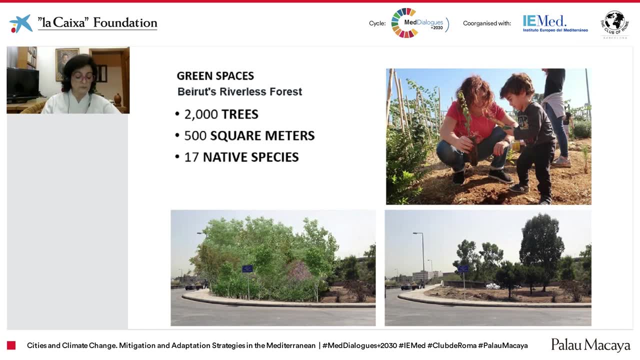 to gain access to the land. Funnily enough, funding was easily collected using the SUGI app, the Sustainable Urbanization Global Initiative app, and a forest which is a service provider for creating natural, wild, maintenance-free native forests. Emiyawaki forests are dense, multi-layered forests. 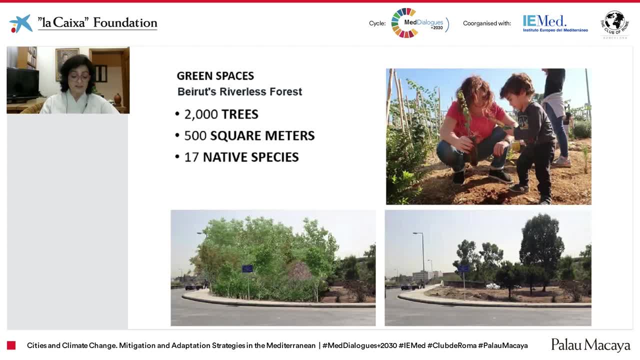 30 times denser than other man-made forests. that's capturing 30 times more CO2 and 30 times more pollution. They are 10 times faster growing and they restore soil, health and biodiversity. in degraded sites They become completely self-sufficient. 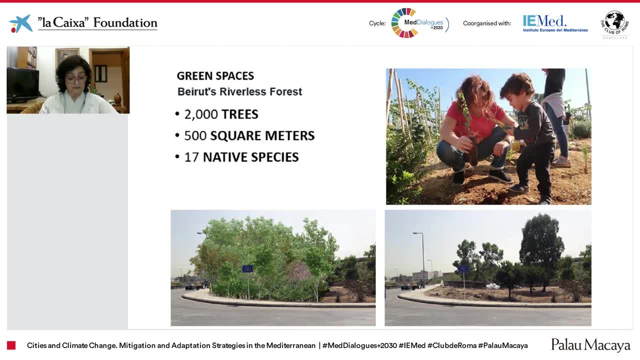 after three years, Emiyawaki forests require no watering or maintenance. In May 2019, the other Dada planted Lebanon's first native urban forest called Beirut's Riverless Forest. The municipality was required to take care of the watering for two years, while the consultants provide. 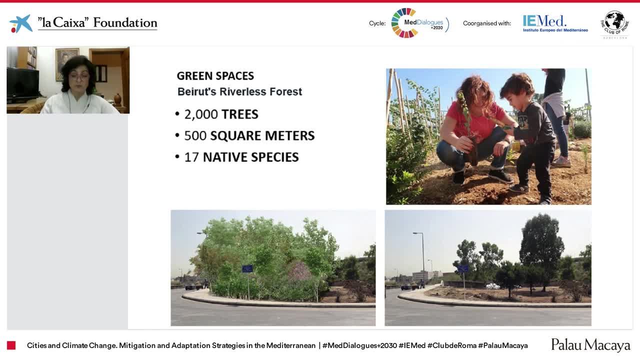 all the fundraising, site work and two years of maintenance. with the help of volunteers, Volunteers from various backgrounds joined the project and helped implant and maintain the project. and the project restored not just the first forest ecosystem but brought communities together. The second part of the planting is completed. 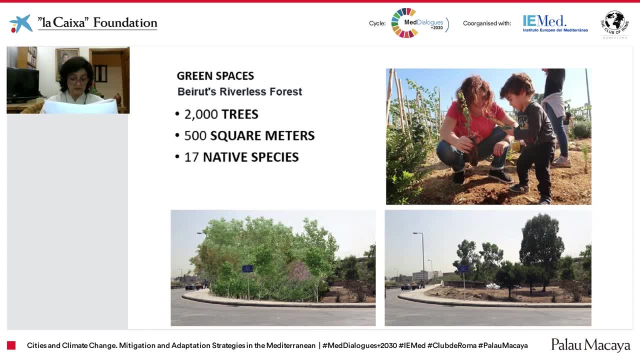 in November 2019, amounting to 2,000 native trees and shrubs and restored land by the capital's polluted river. Beirut Riverless Forest earned the D&AD Future Impact Award in 2019, and I have social media accounts so you can check it out. 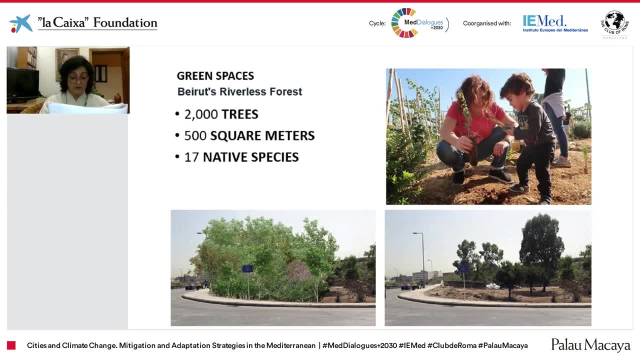 Beirut Riverless Forest earned the D&AD Future Impact Award in 2019, and I have social media accounts so you can check it out. The second part of the planting is completed in November 2019, amounting to 2,000 native trees and shrubs. 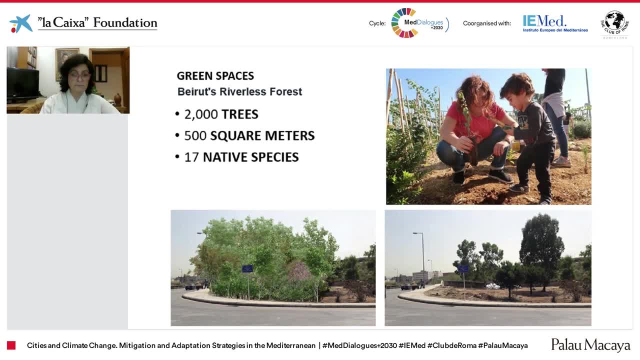 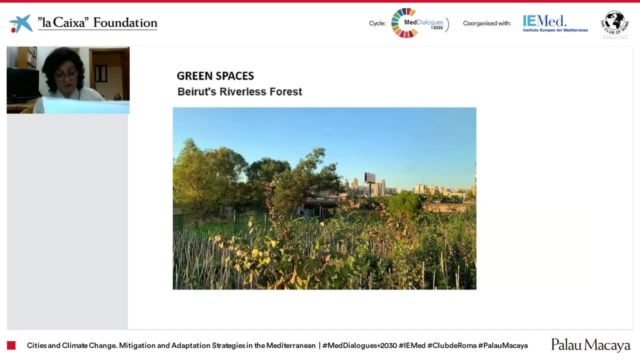 and restored land by the capital's polluted river And the first. The project, therefore, has achieved a lot, from being the first Miyawaki forest in Lebanon to a successful and replicable pilot project for suitations in Lebanon and beyond. We are expanding Beirut's Riverless Forest. in Senn-Nel-Feim in November and we will be planting. We are also planting another 3,200 saplings there, also integrating pathways and central public space. We are also planting a linear forest inside the Shiyah Municipal Park in two weeks. 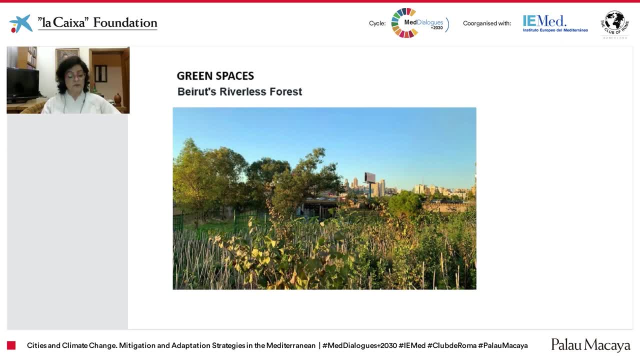 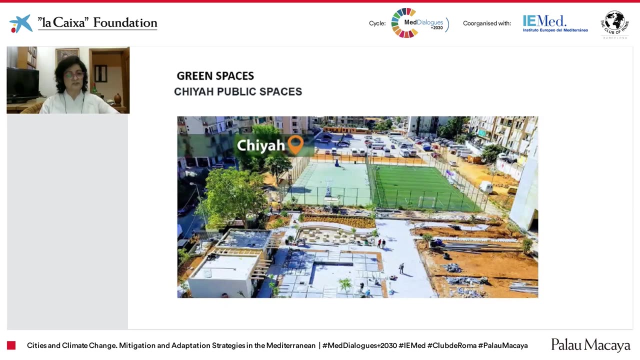 That's 800 saplings, and are negotiating with the Zouk Lesbah municipality for a similar project. I was told by Eddie Dada, the designer behind this project. This brings me, as we mentioned Shiyah, to another project, which is the Shiyah Garden Public Spaces. 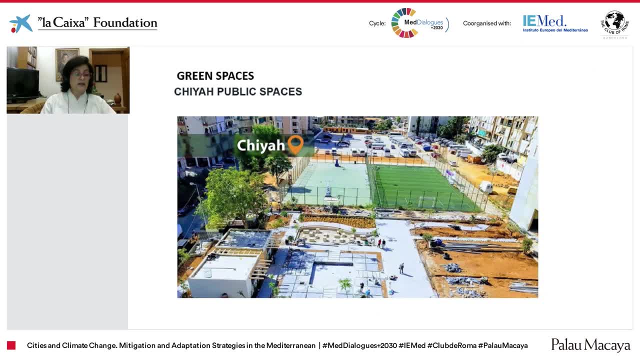 Now, in a way, this is a success story at municipal level, as Shiyah was one of the most affected suburbs of Beirut during the civil war. Many buildings still bore the scars of the war, as it was on the demarcation line. 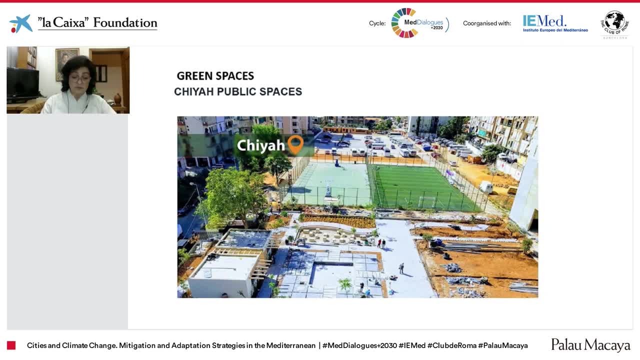 Highly populated area. the municipality, led by its president, agreed on the strategy to change the perception of the area to attract businesses through green public spaces, Working with various stakeholders of the area, from family groups to parishes, local businesses. the municipality's strategy was in three parts. 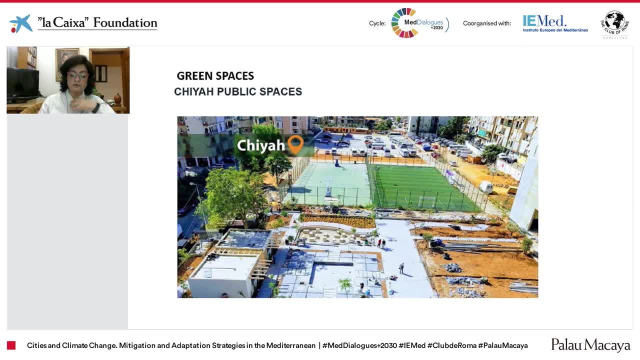 The municipality allowed temporary use of unbuilt lots in the area as gardens and play areas. They also set up the garden and community space which you can see here and brought in others to invest in the natural environment. This was done with additional space and services, such as gardens, host facilities, coffee shops, etc. 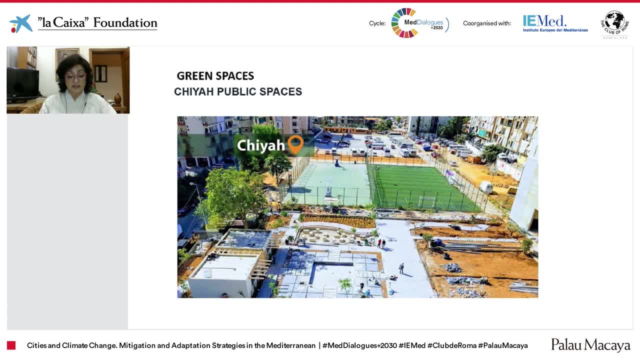 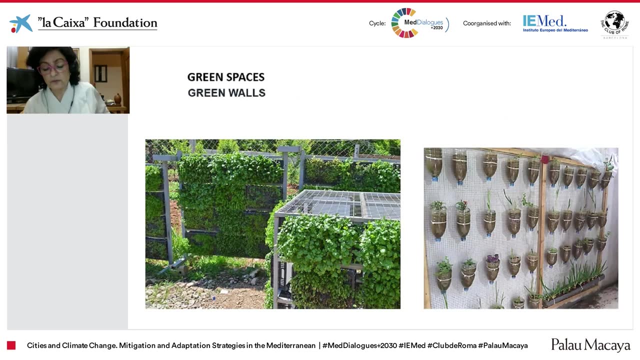 to enliven the municipal spaces. The project has proven a great success as it gave access of the residents to open spaces to enjoy. Now, green spaces can also be used for economic support. This is the garden wall project. It's a micro gardening project. 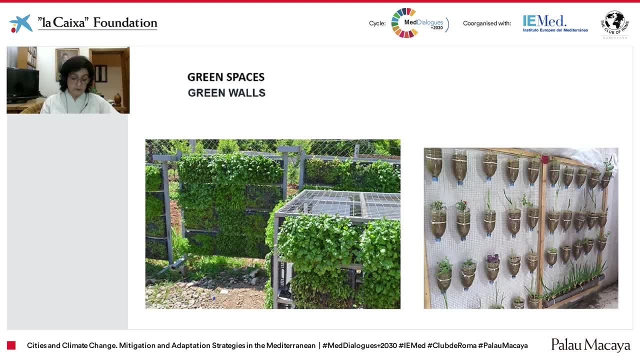 Implemented by the FAO and funded by OKA, managed by Lebanon Humanitarian Fund. Syrian refugees and host communities in Lebanon are improving their nutrition thanks to FAO. The initiative is helping households build vertical micro gardens out of recycled material. Each crate can be used to plant two consecutive vegetable crops per year. 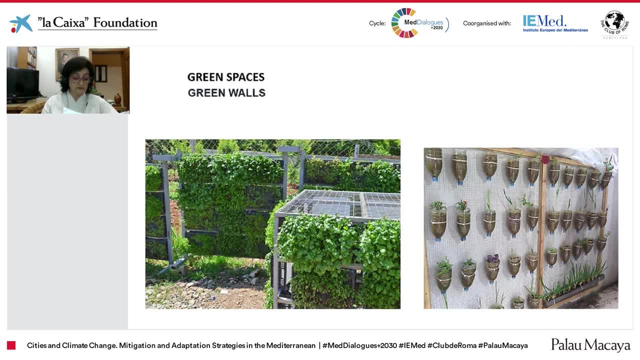 and can be used to grow a wide range of summer and winter vegetables That can be harnessed throughout the year without using arable land. The project primarily targets women-headed households and those with a large number of children, And the beneficiaries until today are 30 vulnerable Lebanese households and 120 Syrian households. 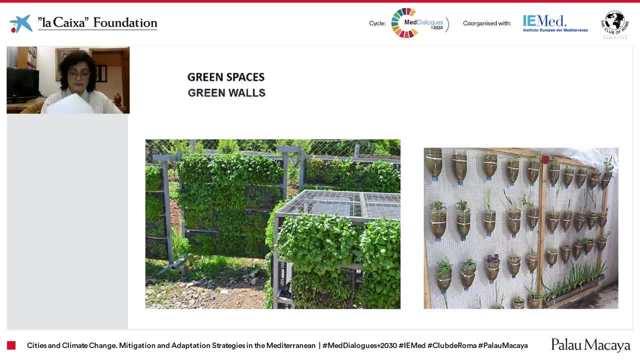 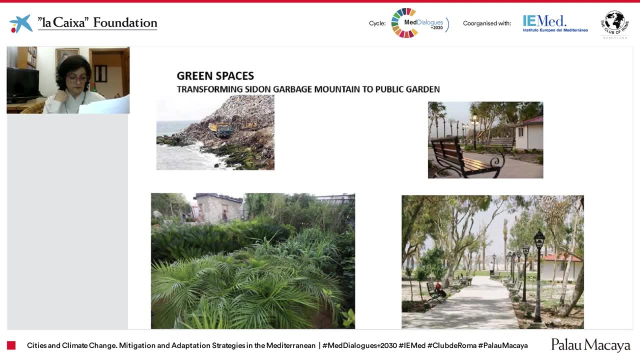 Now, speaking of waste, this is a project that is very interesting. It is the Saida Garbage Mountain project, The Saida Garbage Mountain. the Saida Garbage Mountain, yes, became a symbol of the garbage crisis we suffered in the country. 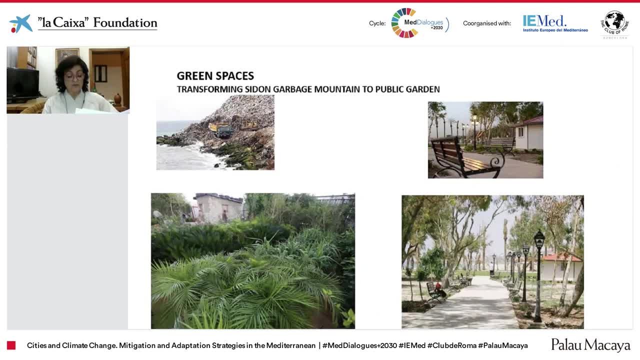 It was set up in 1982. It received 300 tons of solid waste And, as it received waste from 250 people living in 15 municipalities around Saida, the waste mountain stretched 55 meters high from the surrounding terrain and covered an area of 60,000 square meters. 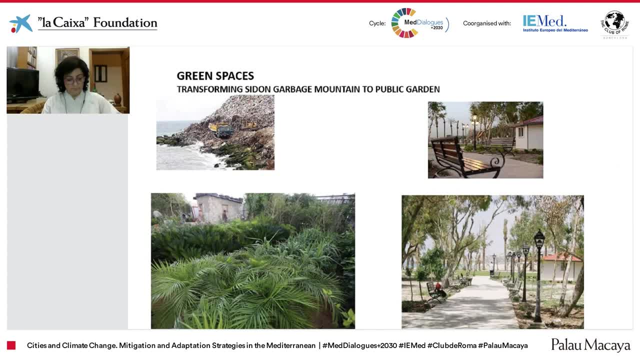 Located on the southern edge of the city, no more than 200 meters away from the residents. the garbage mountain was a threat to the health of the residents And, since it did not have a proper base, the garbage leaked out into the ocean frequently. 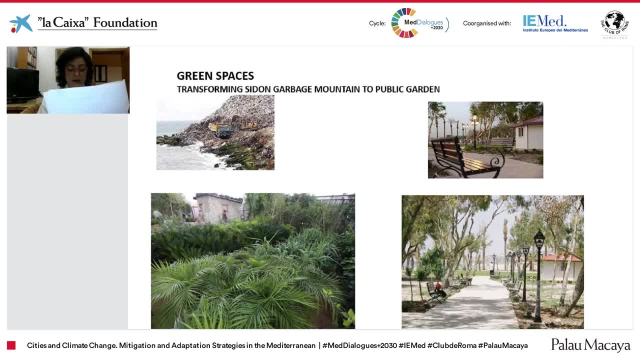 In 2016,, the US DP and the Ministry of Environment and the Municipality of Saida inaugurated the garden project which replaced the garbage mountain. It was funded by the Lebanese government and implemented through the Ministry of Environment and the UN DP. 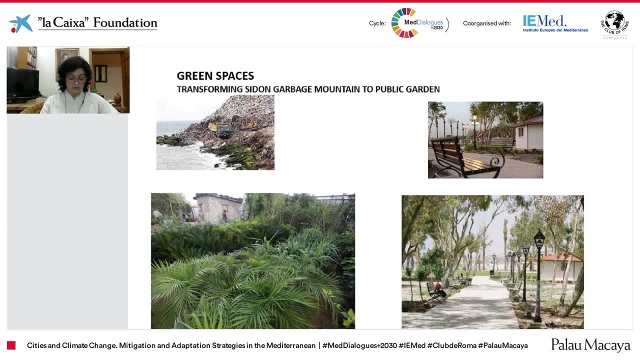 During the event, a documentary went through the process of rehabilitation of the site, from degasification to sorting waste from rocks to plastics, etc. And finally landfilling by burying organic waste. The result was 33,000 square meters of garden, with more than 10,000 trees, backgrounds and theaters. 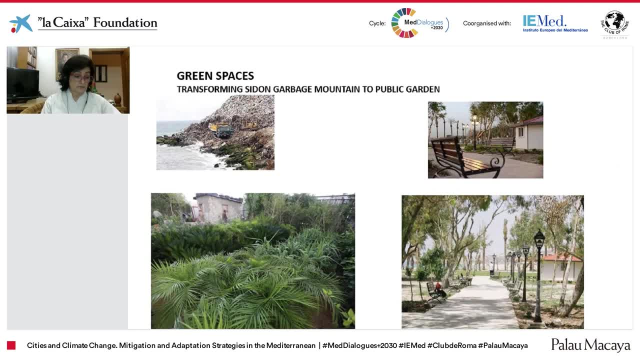 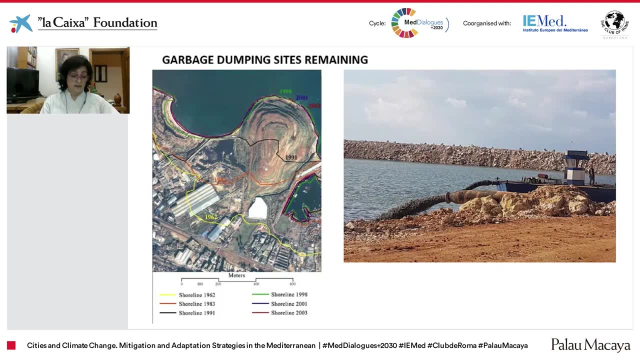 However, this is one garbage dump on the Mediterranean that has been successfully dealt with. The government still lacks a comprehensive plan to deal with the garbage disposal, As the average resident in Lebanon produces up to 3,000 tons of garbage, which is 1.2 kilometers of solid waste each day. 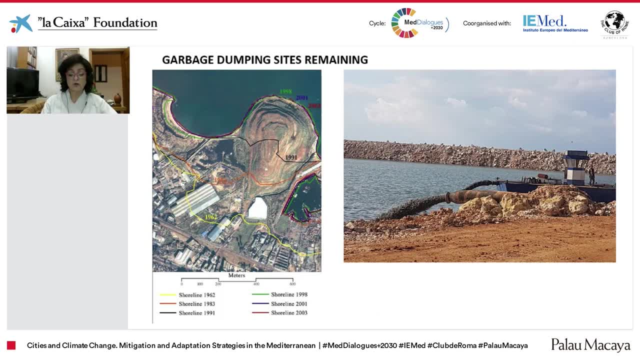 with more than three-quarters of it destined for landfill or an open dump site. At least two garbage dumps are still being used along the Mediterranean in Lebanon: The Costa Brava, which we see on the right, and the Birsh Hammoud dump, which we see on the left. 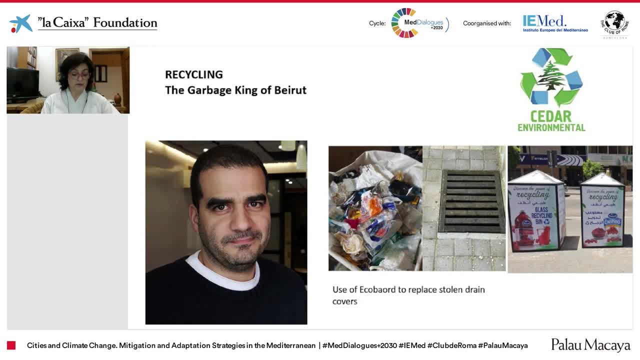 One individual who probably has done more for waste recycling than any other entity in Lebanon is known as the Garbage King of Beirut. engineer, Ziad Abishaker, He launched Cedar Environmental as a salt and composting company in 1999, after he returned from the USA. 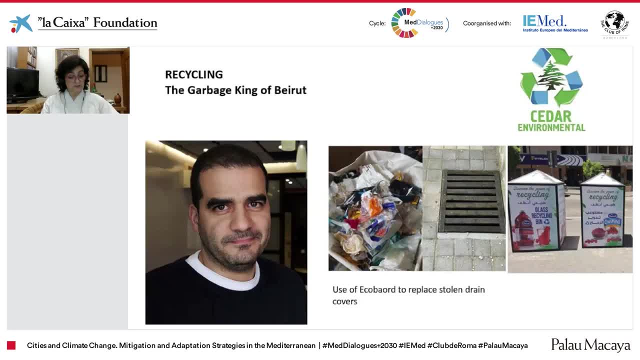 He was soon faced with corruption when dealing with large municipalities and other government bodies. Abishaker's main aim was to build smaller-scale recycling plants to deal with garbage for smaller towns, and it took him 10 years to set up 12 recycling plants. 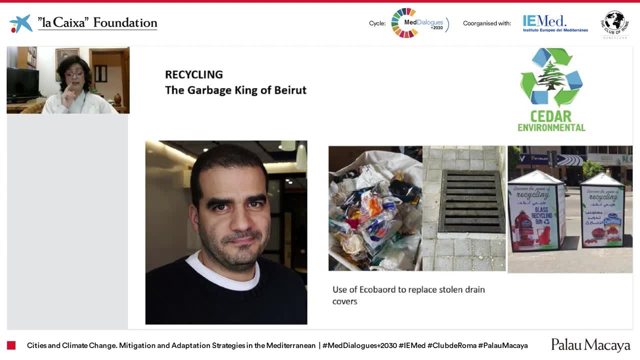 Abishaker then went on to innovate and came up with a patent technology that produced what they call ecoboards Made from recycled bags. ecoboards are highly durable and successful for small construction, like the recycling bins found in Beirut, soon to number 150.. 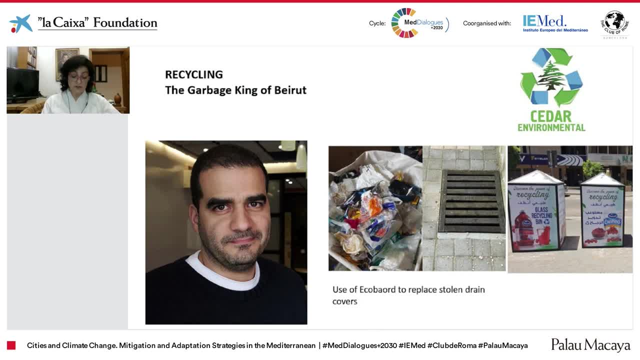 Ecoboards were also used to make vertical planting structures, and we can see them here. They were used to make the drain covers, because, during the economic crisis, anything metal was actually stolen and sold for money. Now, with an experiment, Abishaker was able to use the ecoboards as planters. 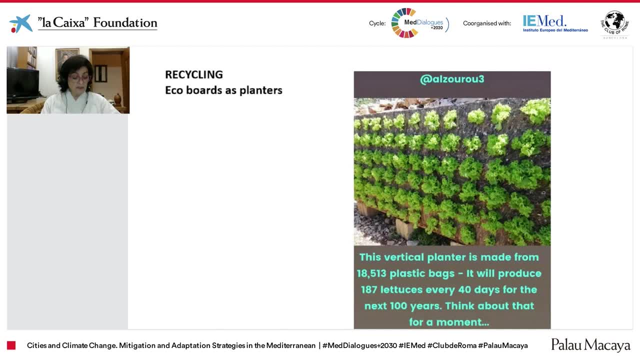 The 12 planters, made from 10,000 plastic bags, were planted and within 41 days produced 2,000 heads of lettuce. Now this is part of a project to promote roof gardens in the city and help bring back the birds back into the heart of the city. 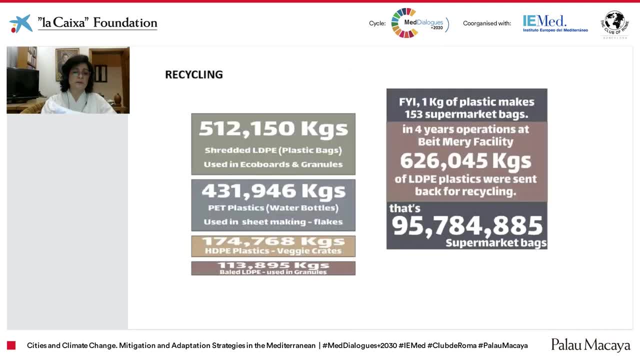 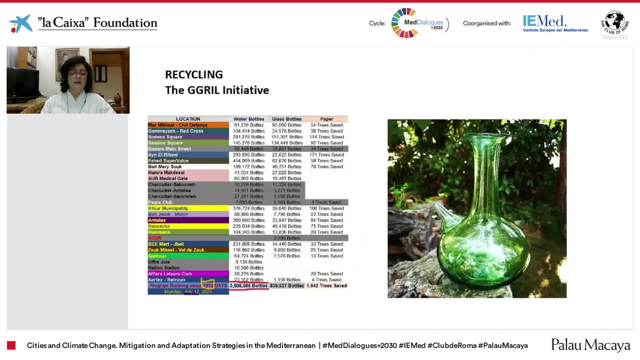 His next and this is some information about the recycling. this is from his late Mary facility. Now the next and very important innovation was linking glass recycling with the old, traditional Lebanese craft of blown glass. The Green Glass Recycling Initiative started in 2013. 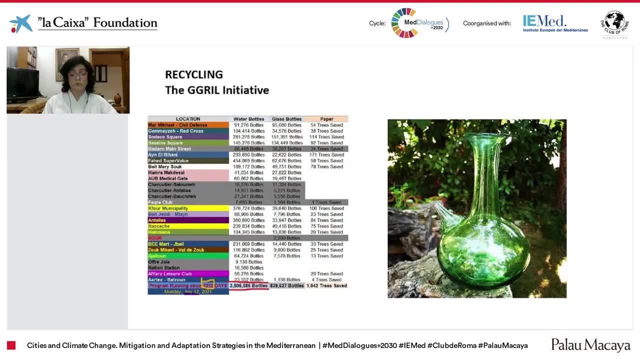 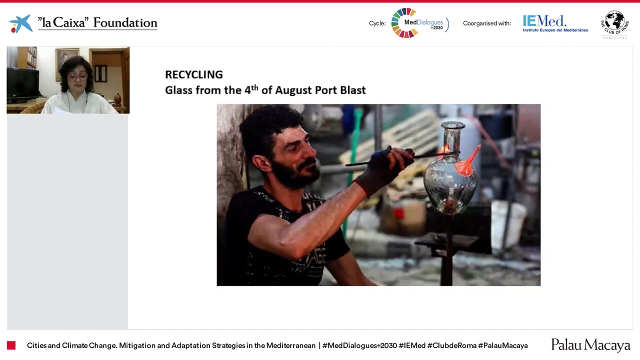 after Lebanon's only recycling glass factory was bombed in 2006.. The collaboration with six remaining glass flowers in the country was to produce beautiful multicolored glass items and after the August 4th port blast, Abishaker transported eight tons of shafted glass to be recycled. 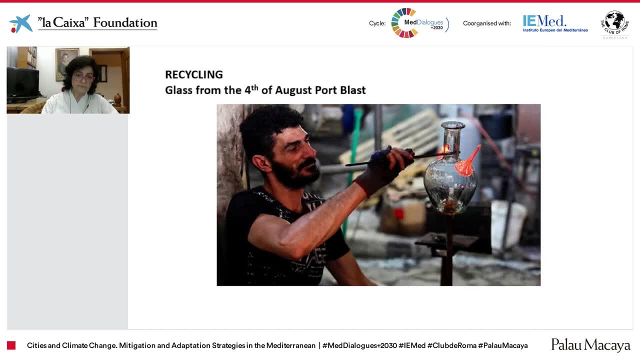 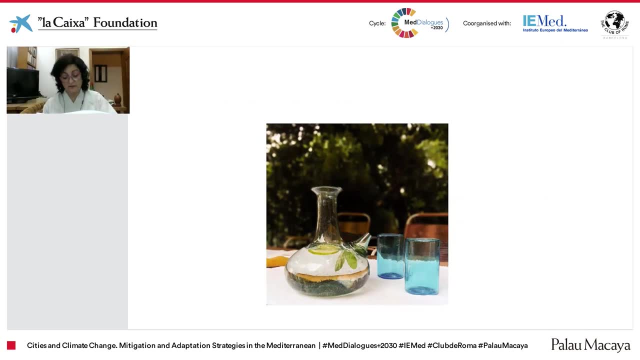 and this is one of the projects. Finally, to conclude, it is clear that the precarious situation in Lebanon has rendered central government and ministries unable to fulfill the many recommendations and studies and reports made by donor agencies on climate change mitigation, One small positive aspect of the tragic economic meltdown in the country. 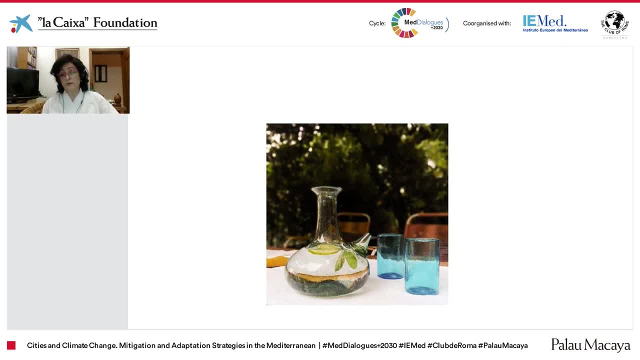 has been the lifting of subsidies which has been an eye-opener for the citizens. We have seen how citizens of the country have driven very valuable and important initiatives to help reduce environmental damage and global climate change. But, valuable as they are, issues like monitoring global warming need an overall structure. 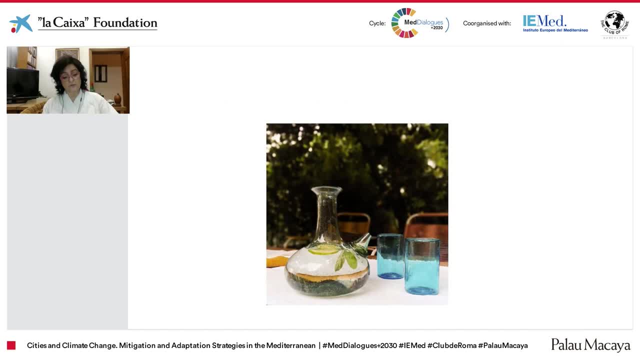 that plans, coordinates and follows through on these initiatives. Climate change is a global matter and governments need to be held accountable, And here I'm referring to the dump sites on the coast of Lebanon. Coordination is required between international agencies and donors, with clear mechanisms of follow-up and retribution. 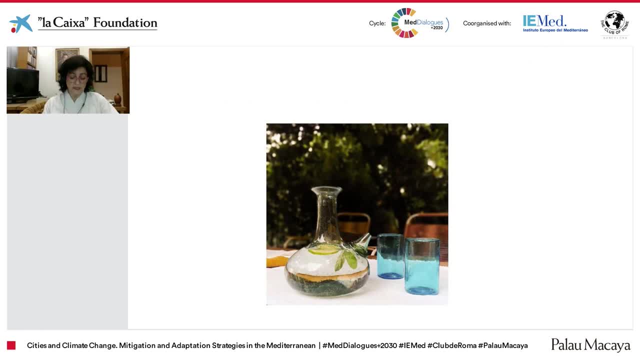 But at the end of the day, though, the people of Lebanon and the government know what is needed to be done, but the threat of conflict and political instability in the region. their priorities are, unfortunately elsewhere. Thank you, Thank you. 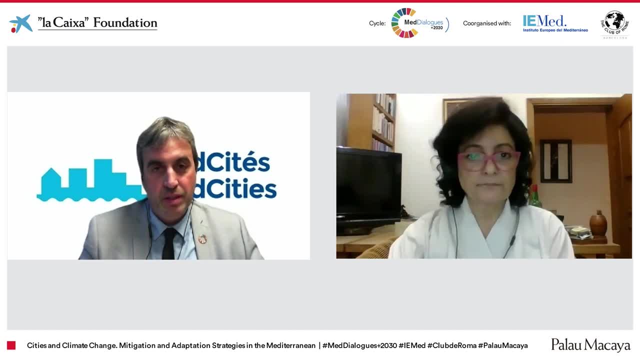 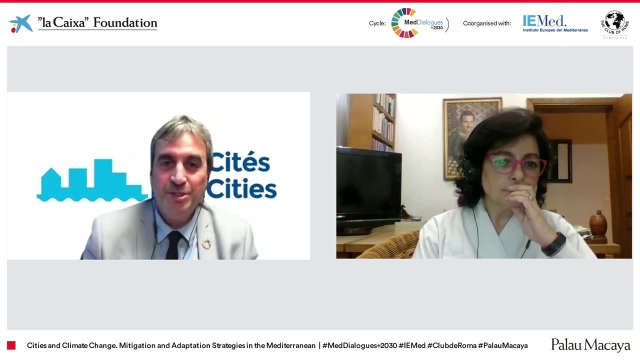 Thank you very much. This is, Mrs Alamuddin, Very inspiring examples of the work that's been done in Lebanon. That makes me reflect on something, but first let me recognize not only the European Institute of Mediterranean, but also the Club of Rome for organizing this event. 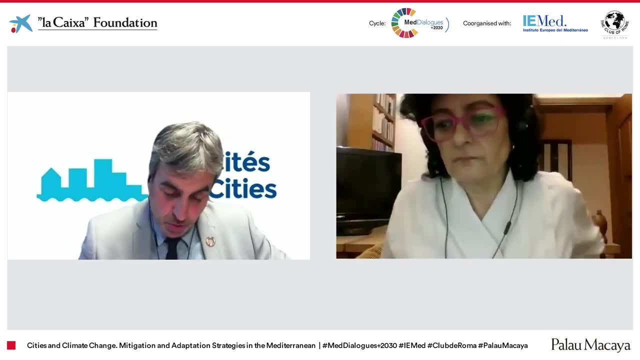 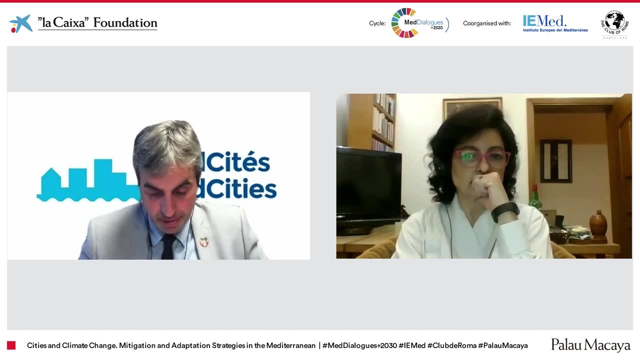 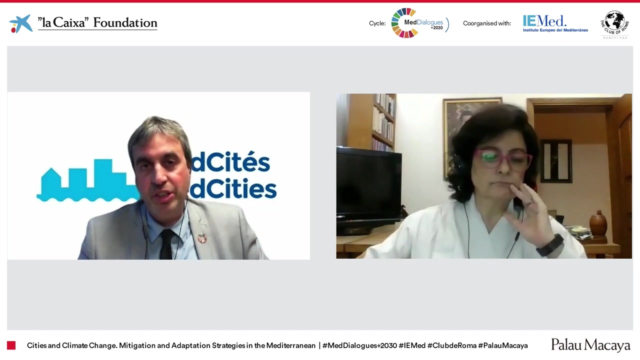 And what you said. I would like to highlight some of the ideas that were just said and impose some reflections. some more reflections on my behalf. Firstly, I think that the need of working together- you express this- is much needed for the small municipalities. 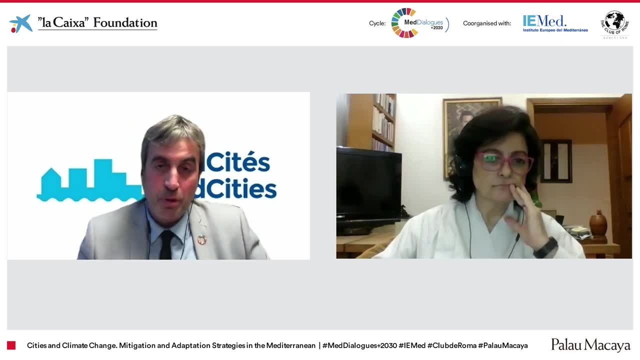 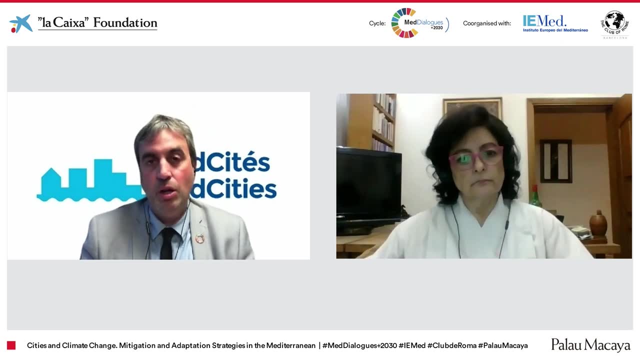 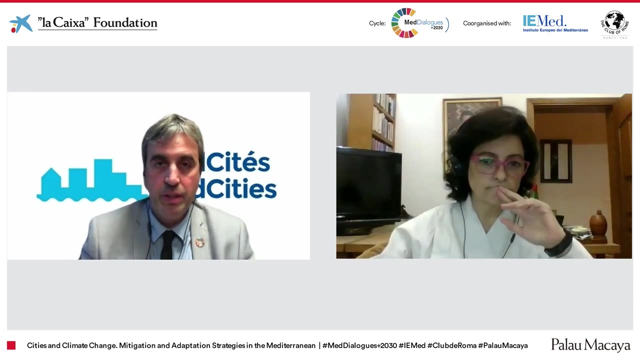 So cooperation and, if it's possible, institutionalized cooperation like that we have here. for example, where I'm right now, MedCities is hosted by the Barcelona Metropolitan Area, which is an institution of 36 municipalities that work together, that share competencies on waste management, on water cycle, on energy, on mobility. 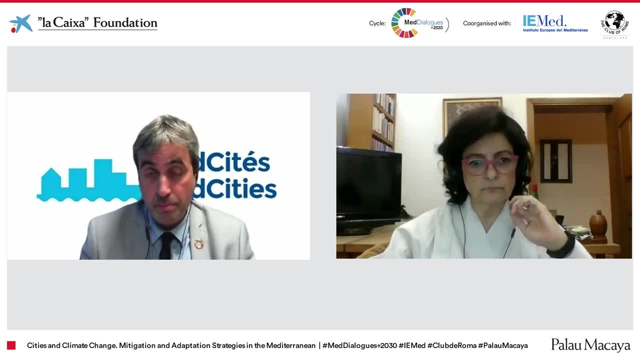 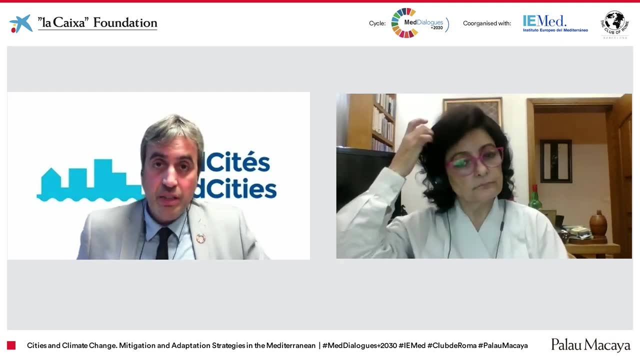 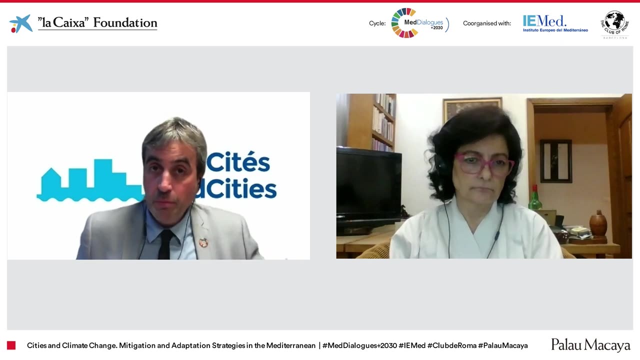 The Metro of Barcelona, in fact, is managed by the metropolitan authority, not by the municipality, For example. so it's very needed to tackle climate change, to work together and give bigger scales, most of all for the small municipalities, because they don't have resources. They have fewer resources. 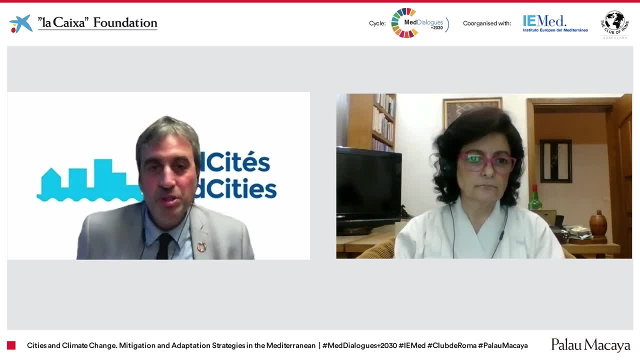 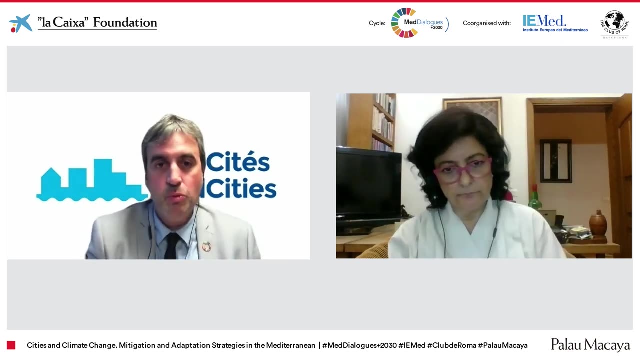 In many cases, in very small municipalities, the only person who is dedicated to this function is only the mayor, for example, or one engineer, or only or only one architect, so they don't have specialists, experts in waste management, experts in mobility, experts in public spaces. 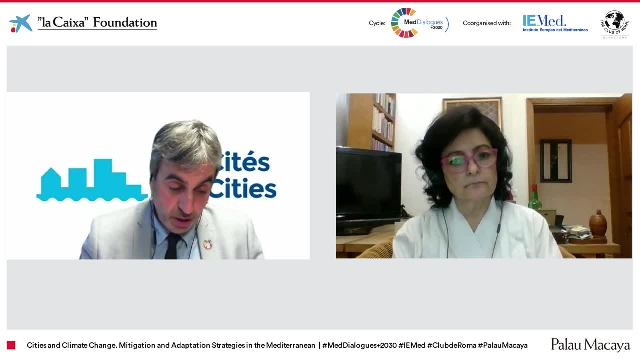 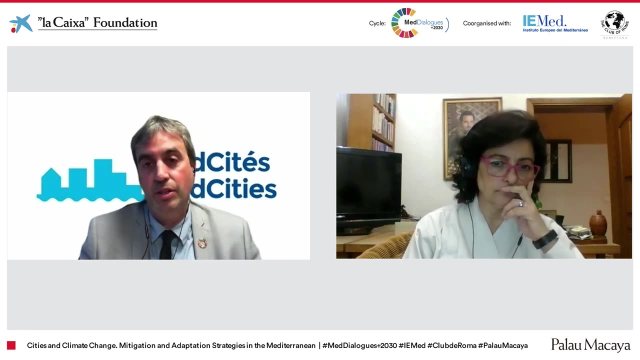 So it's very important. Another thing that I would like to highlight from your words is the need of political stability, of course, for doing great infrastructures, For example, the recovery of a river, a metro, a sub-railway, as you expressed. 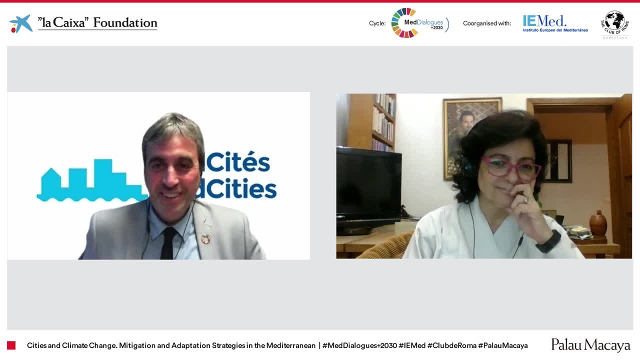 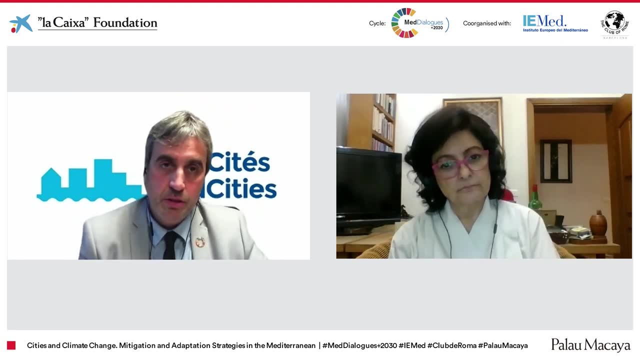 It's very important. It's very sad to see that sometimes the money that is providing international funders is not going to the right places or not going to the final objective that was aimed. So it is very important to have political stability and strategic planning, strategic planning and urban planning. 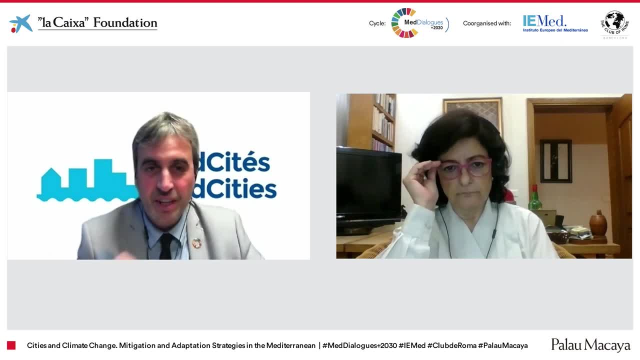 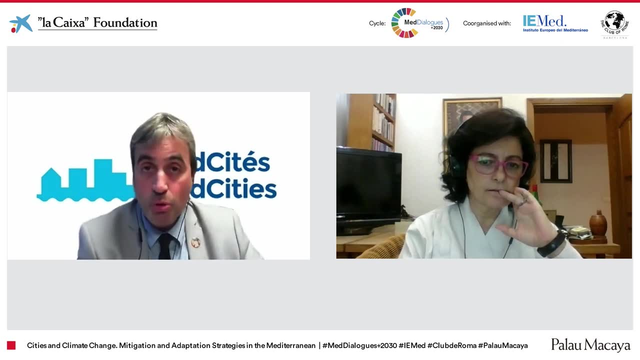 Not everyone is doing strategic planning. Let me say the met cities has done, has conducted some strategic planning, Some strategic planning across the Mediterranean region for some, for some cities. from that, from those works are becoming in specific actions, planning actions during the last 10 years. 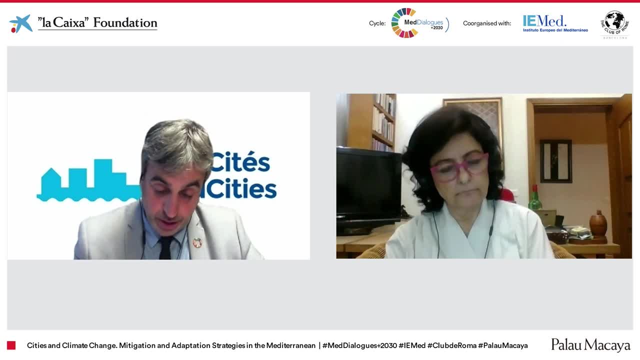 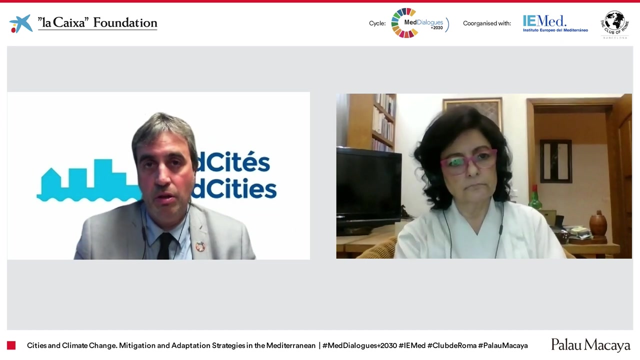 So it is very important to to, to, to planning, to know what you are willing to do, surpassing the mandates, surpassing the political orientations- maybe in some aspects There- of course there are- There has to be different political orientations, but there are main, main issues that have to be. a general consensus is, I think, one of the main aspects that I also obtained from your words that we need consensus to do the great works: the transformation of the city, the planning, green spaces, planning, metro planning, the recovery, for example, of rivers, planning, the extension of renewable energies. 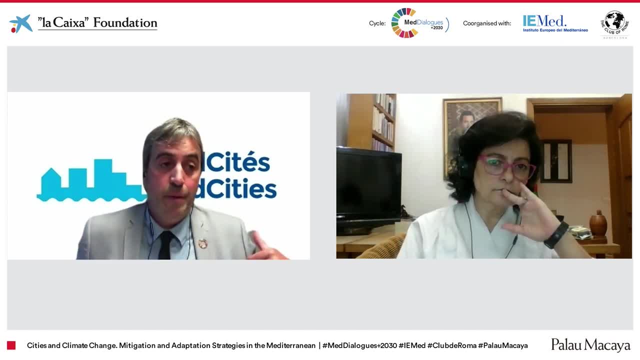 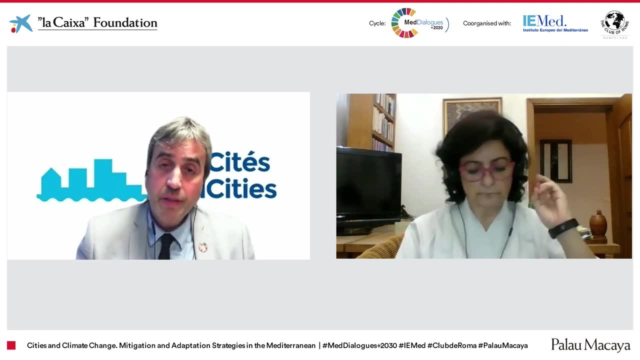 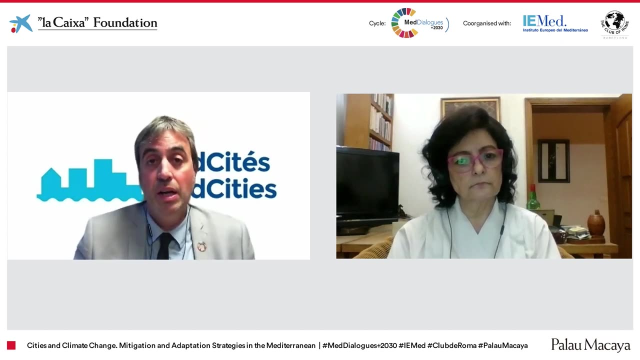 Isn't it? I think it's very important to have consensus, because these projects, uh, last more than one mandate, one political mandate. So for me it's very important. Another thing that I it's important for me from your words, in in some of the cases you express, is the appropriation of the measures. that must be done by people. 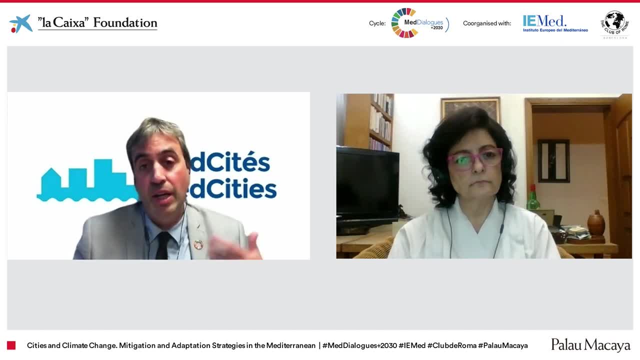 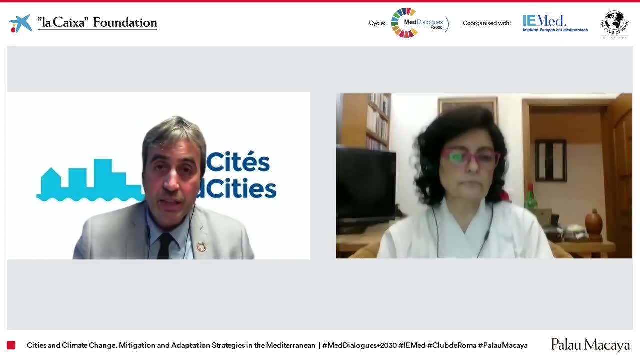 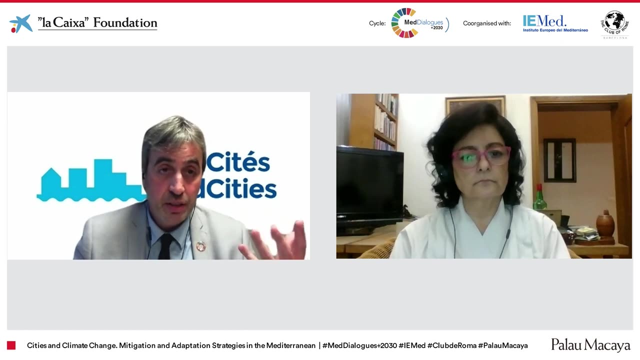 And you can co-construct with people the case of the of the stairs, uh, the tiles, uh, some of the things must be done with people, with general public. We need to raise awareness And and and, because changing behaviors will also change the, the, the way of people demanding solutions for the representatives. 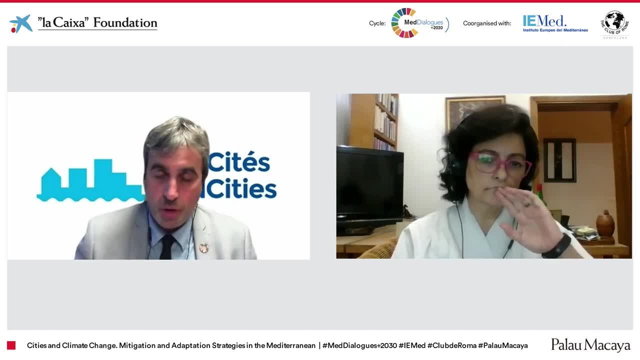 It's very important. It's sad to see, but it's so common to see uh dumping places like like garbage mountain uh, but they are frustrating. uh uh reasons, but you also provide a hope, Mm. 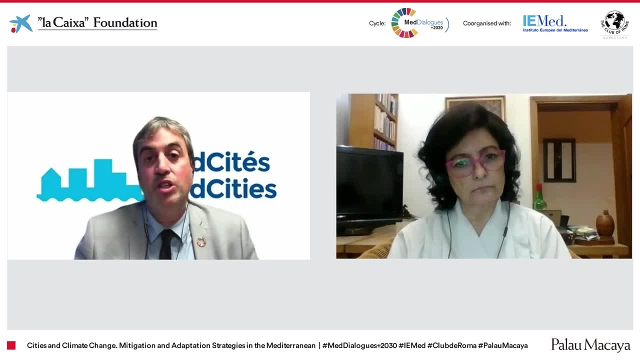 Mm, and good examples on how we can tackle, if there is political will, if there is popular will to uh, to press to the politicals also and to vote to the right direction. regarding, of course, we have to regard your own uh personal uh orientations, political orientation, but 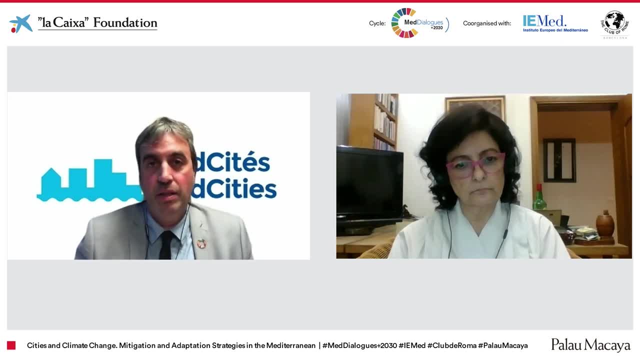 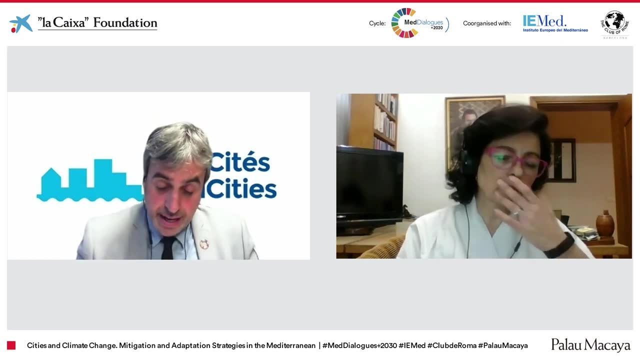 ask them to solve what the problems that, uh, that are there, regardless the political orientation. so it's very important to that and i like to highlight also, and, and and gives me a reflection on on the importance, in my opinion, of green public spaces- is is a good way to democratize. 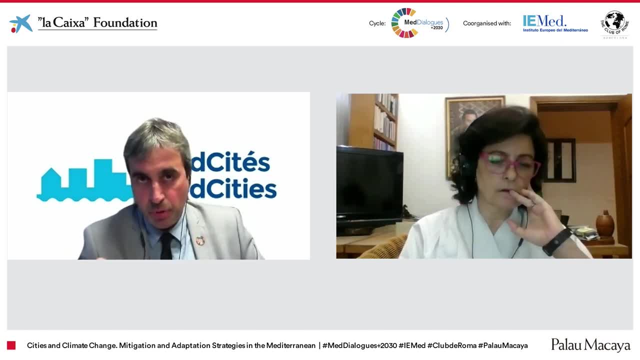 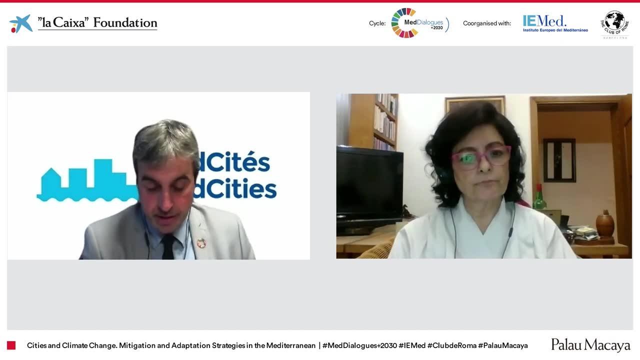 i call it, democratize the public spaces, the, the example and and of of the render and the actual situation in the present situation, for example, that the, the project is trying to to achieve. it's very important. we we could show many of of of aspects, uh, uh. 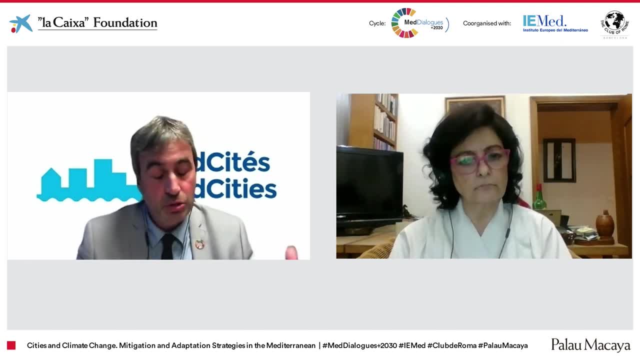 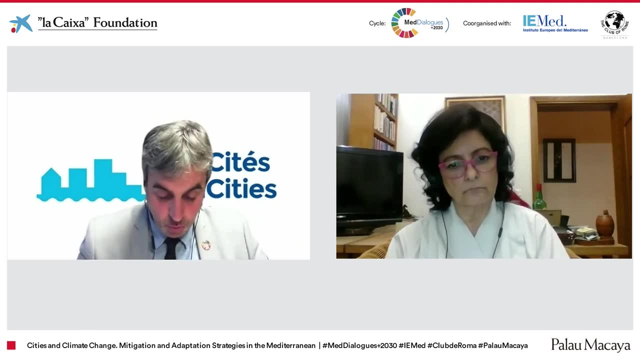 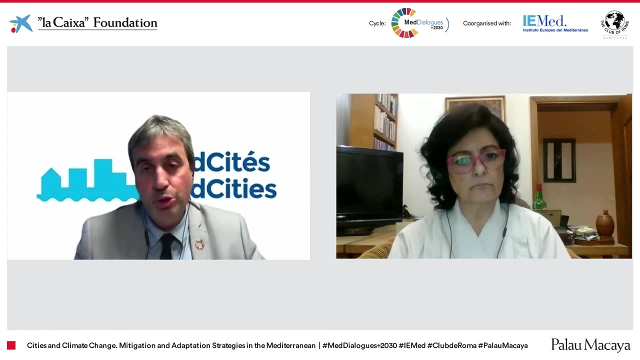 in the world transforming, uh, green space, uh sorry, gray spaces, into green spaces. so this is for me, it's democratized, so i is also a thing that i wanted to to highlight and the different scales and the, the ability of the restoration, as you showed, of one of the of the 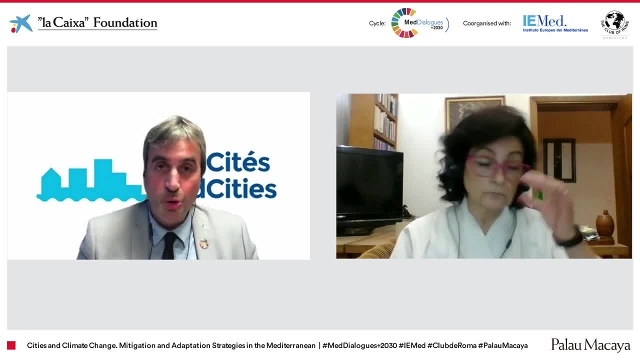 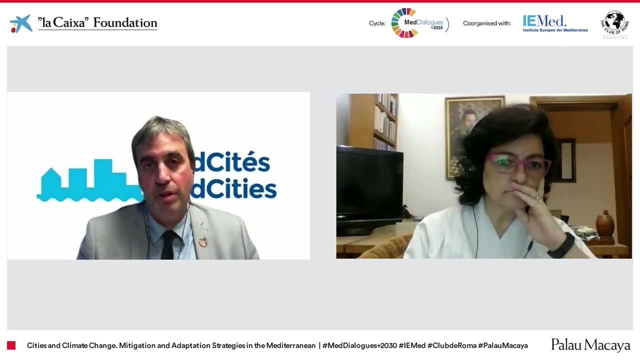 of the government, mountains. it's very important to see that there is hope, there is that you can turn things into, into- uh, there are good examples of turning things, bad examples, but also good examples that some things could be restored: rivers that must be, they can be restored. and just finally, and to put maybe, 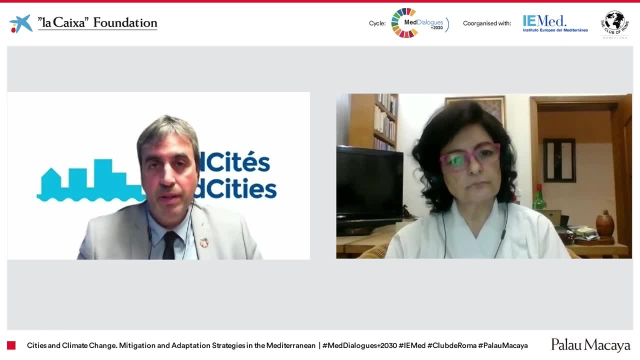 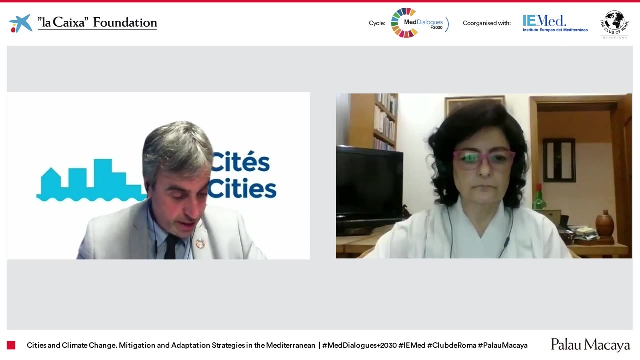 some for, for your reaction, or for the people, uh, all the public that are. we are the audience that we have today. please, uh, pose your questions, but i i like to pose one reflection and if you wanted, uh uh, mrs al-amuddin, to to react that, 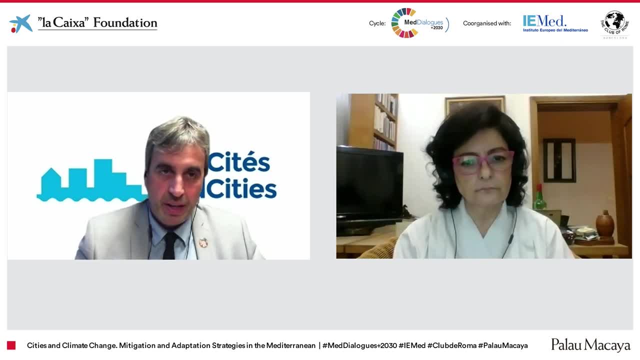 we see in the river the example of a damaged river which was paved in order to uh, safe from flooding. but uh, we know the ecologist it's. the best way of flooding is is have green spaces into the river, having the riverbed, having the, the green space into the riverbed and then the riverbed. 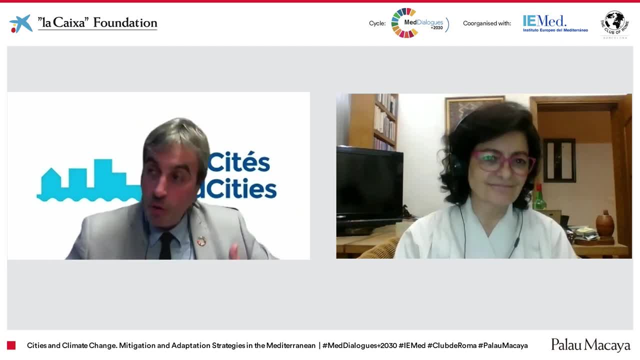 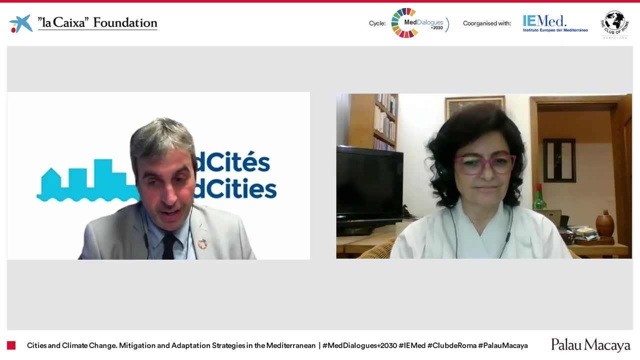 having all the meanders of the river, having all the spaces to flooding, And so they have not to be urbanized. So and we have an example in the river, in spite of debatement, the river taking advantage of the river by putting solar panels. 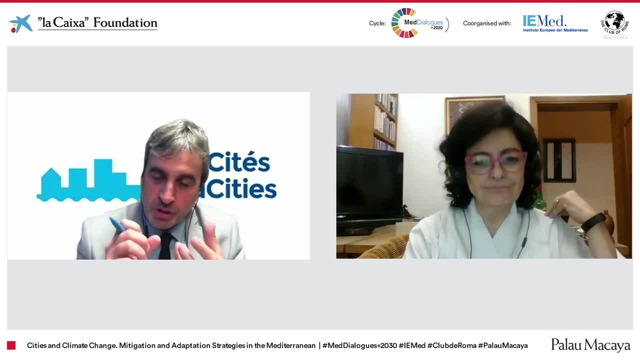 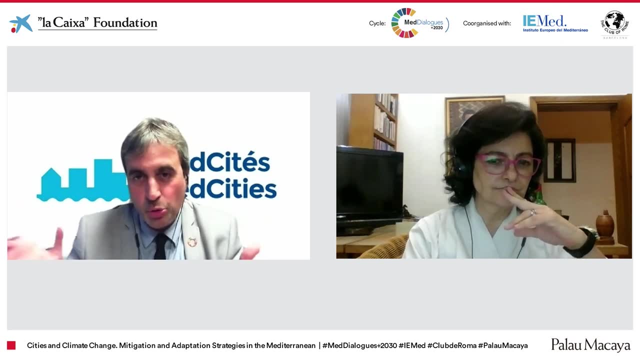 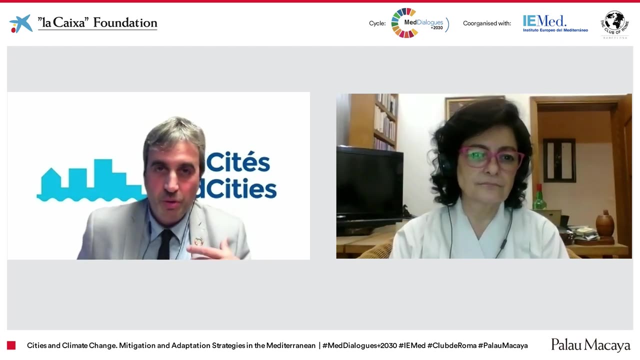 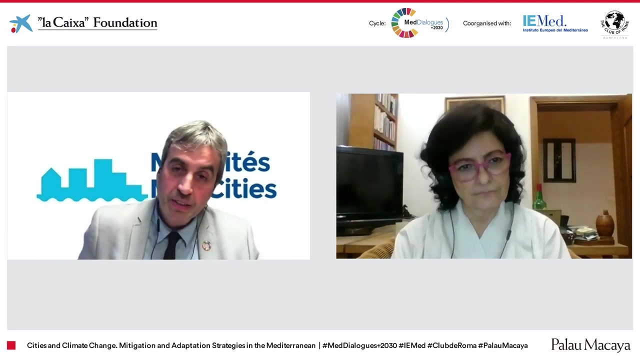 So it's some kind of contradictory And maybe it poses me a question of mitigation versus adaptation, and how many trends go to the adaptation instead of mitigate or restore? So? and we could do this with selecting waste instead of preventing the production of waste, or boosting the renewable sources of energy. 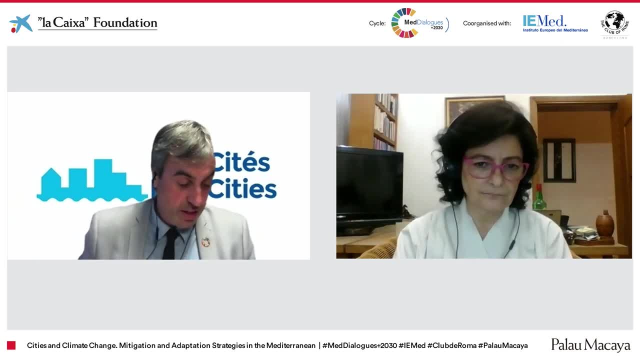 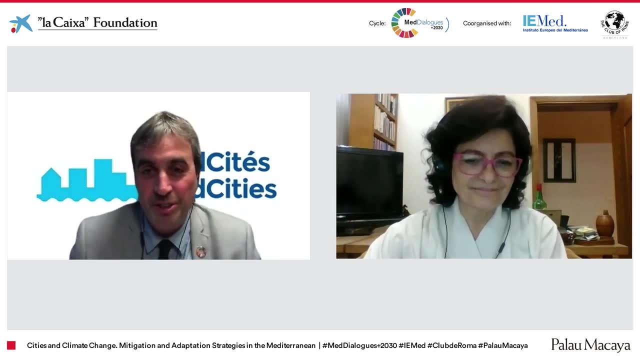 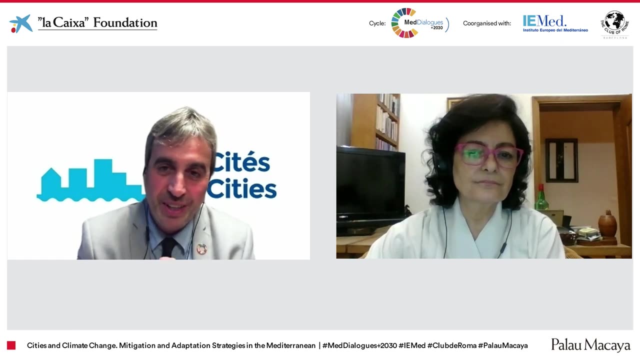 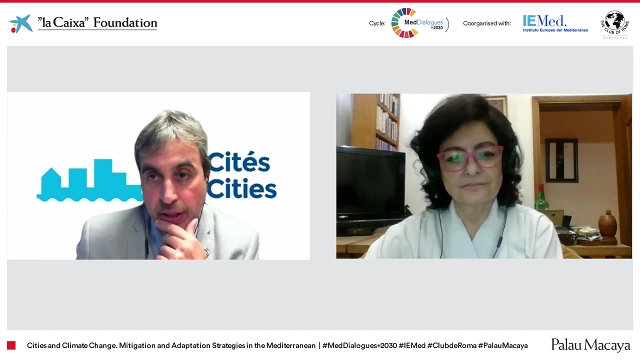 instead of saving energy, for example. So this is. or electric cars instead of public transportation. So no, we are not really changing the pattern or the model. So this is something that maybe you could react to this view of mine, And, of course, we are willing to see if there is someone from the audience. 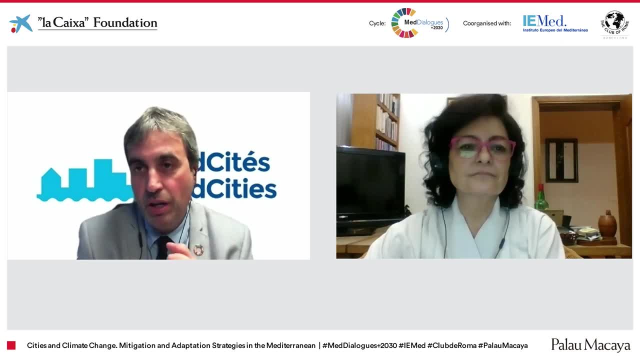 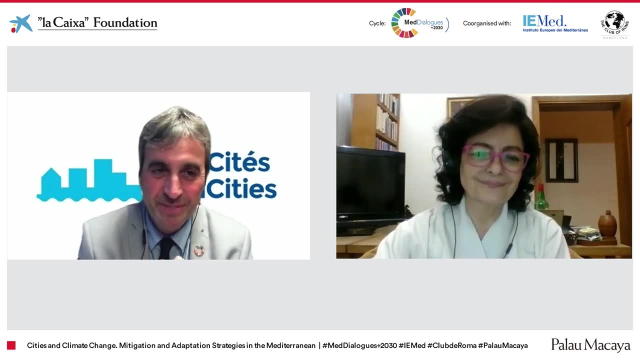 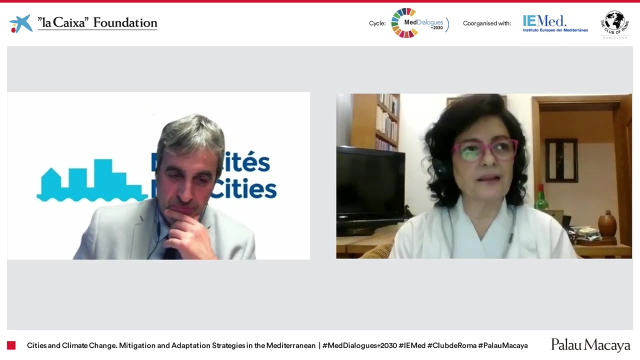 We would like very much to have your your questions from the audience, but maybe, Mrs Alamuddin, you would like to say something about my reactions. Yes, I mean, yes. I think the difference between, like, adapting or mitigating is how much power you have over the situation. 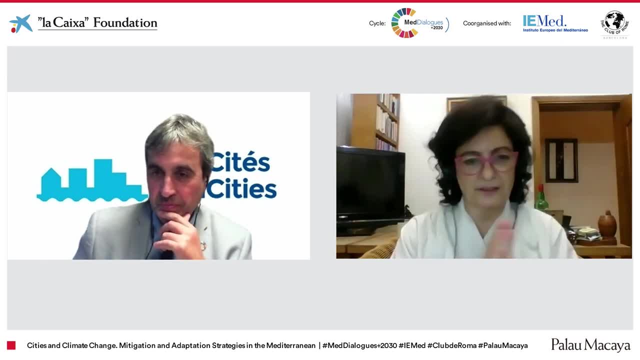 because if you are in control you can mitigate, but if you're not in control, then you need to adapt and you need to make the best of what you have, which is really the story of our lives in this country. So the issue of the solar 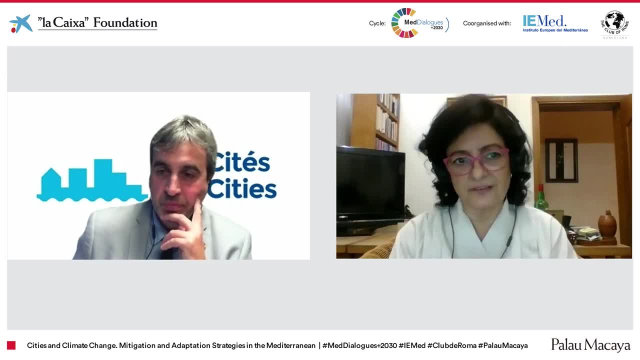 the issue of the canalization of the river happened in the sixties And for some reason, it seems, it was quite a common thing, because we have it again in the Abu Ali River in Tripoli. And so, given the terrible situation that the river became, 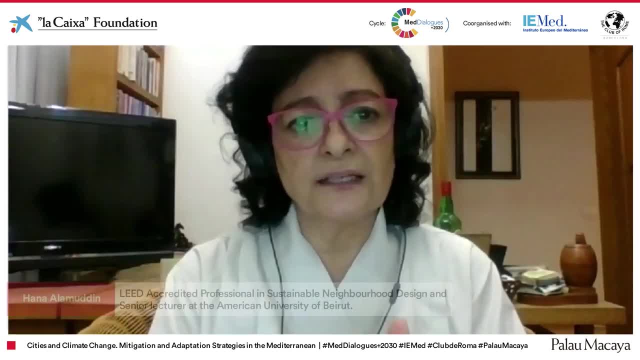 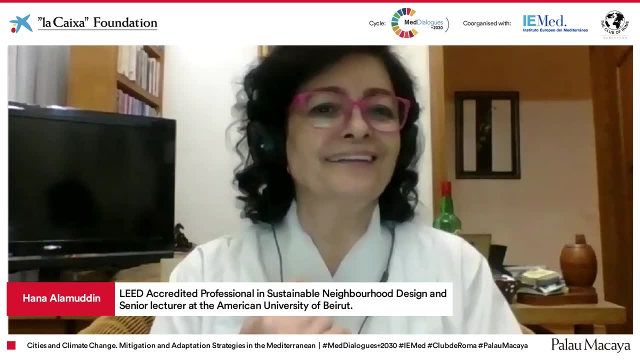 which is a sewer. they decided to try and do something which is more useful by installing solar panels. But funnily enough, the Adib Dada, who's one of my students, I talked to him today about this project and I said: 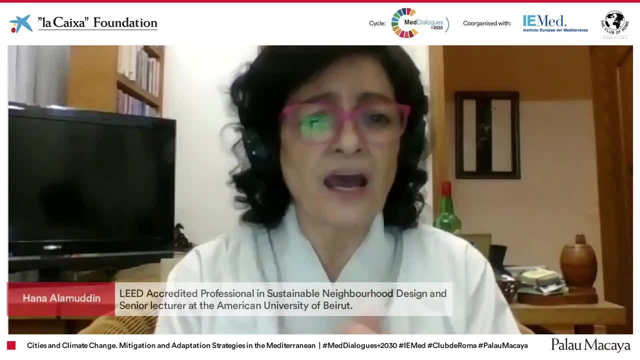 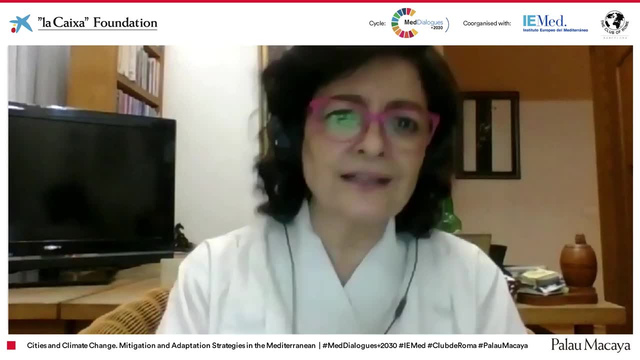 why did you do this? And he said: because I was very upset about them covering the river with solar panels. So I thought, okay, we cannot get the water back, We'll get the ecology back. And so it was his reaction to something that 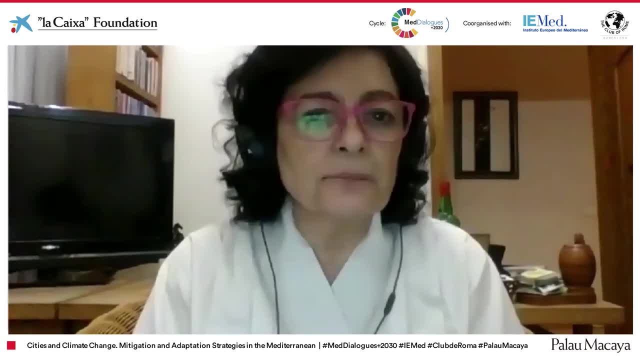 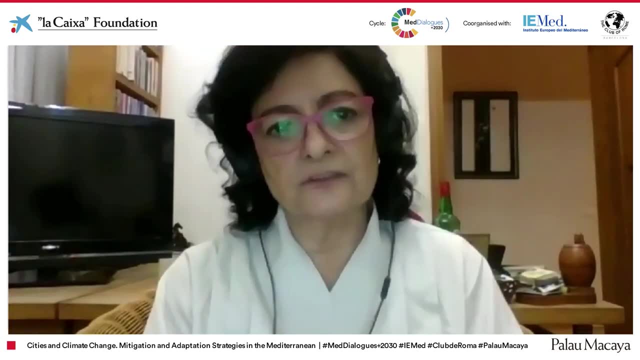 you know. on the other hand, I think it's a good project. I mean, what can you do Urban? Urban expansion has come right up to the river edge And anyway it's too late. So it's a good compromise between the two. 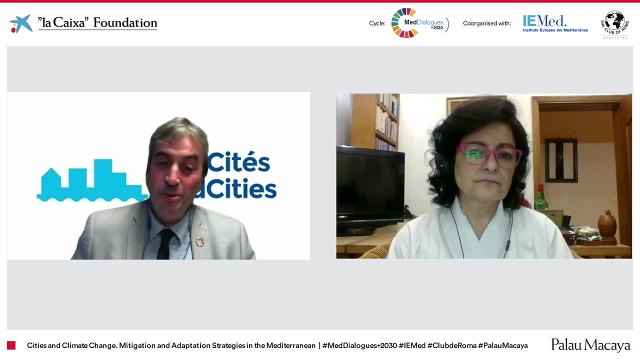 Yes, it's very interesting what you say. If you have power, you can do either one thing or the other. It's very interesting, of course. Yeah, I just want to say one thing. I think that you know, again, to look at, the issue is very global. 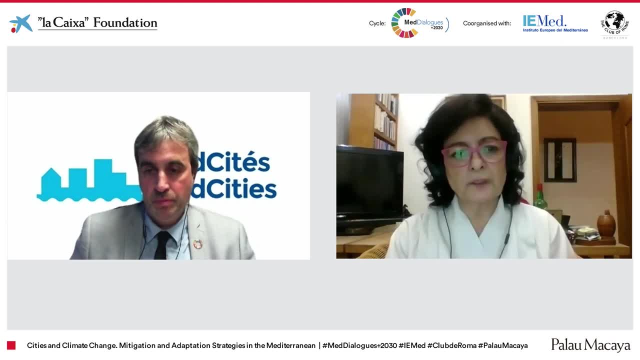 And I think that you know when I was doing my research: there's so many studies, so many reports done by donors and agents and so on, But yet there is no follow up. You know the studies are done and there is no. you know. 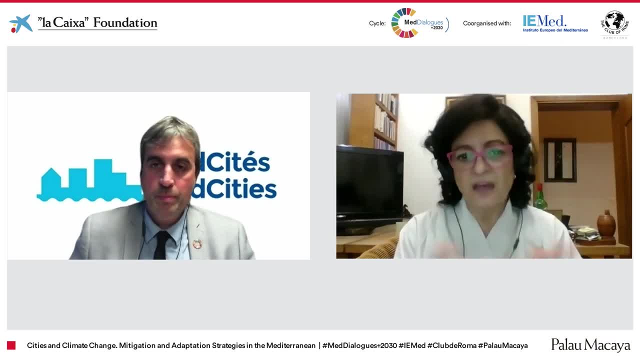 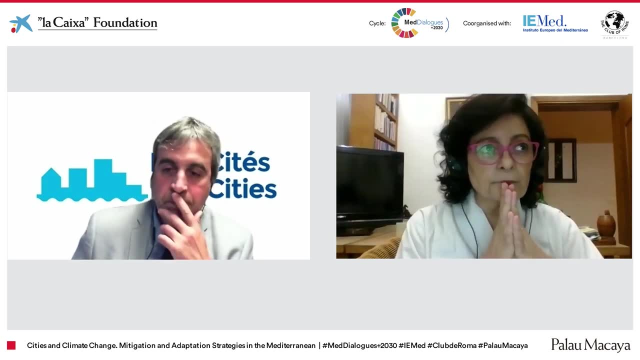 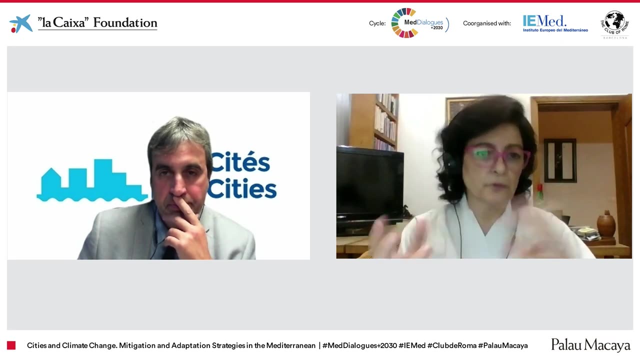 governments are not questioned as to what's happened, Like you know. why isn't it? Why isn't it being implemented? What's going on? So there is this issue of being responsible, And I think that it needs to be on both sides. 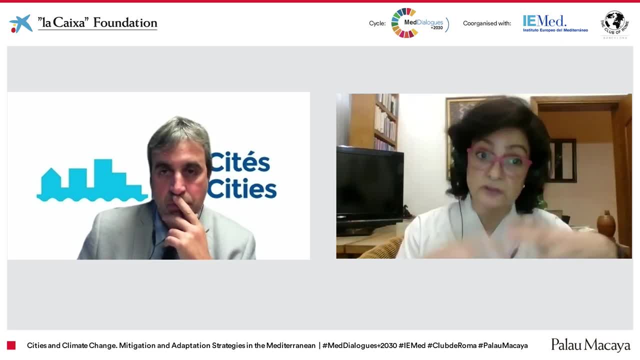 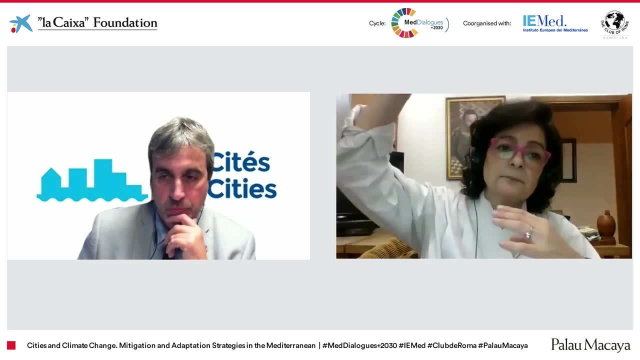 not just the receiver but also the donor. needs to follow up and needs to make sure they're dealing with the right people. needs to make sure that they're dealing with the people across the scales, from not just government but down to the municipalities and down to NGOs. 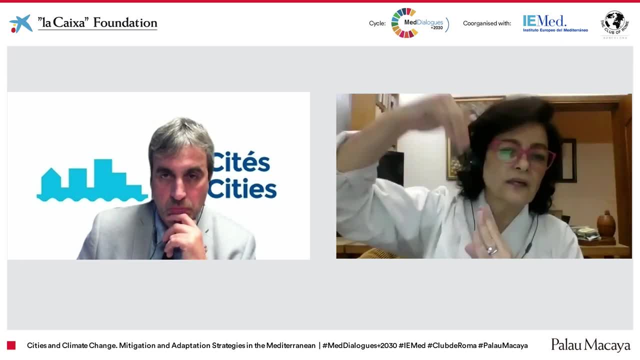 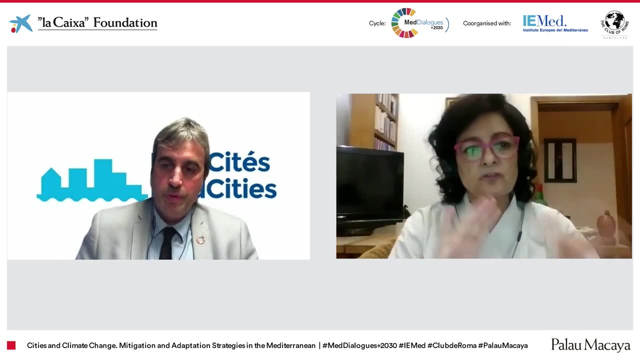 So you know, because if you just deal with government, then it stops there. But if you include the whole scale of the community, then there is always one that's going to carry on pushing. You carry on pushing for what needs to be done. 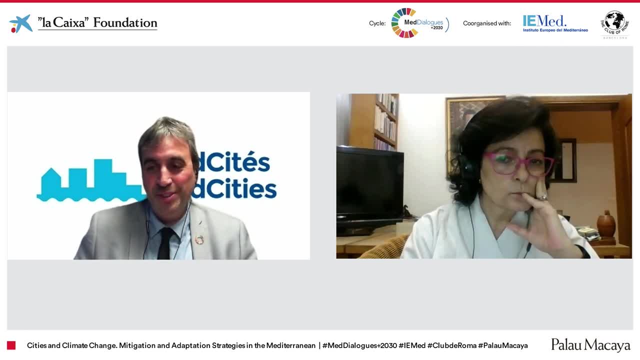 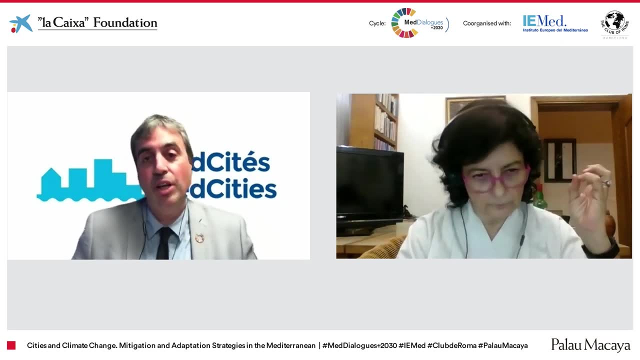 Very interesting, And this leads me to explain again what MedCities are doing. MedCities is this kind of link between the funders and the final receivers, And we know what exactly sometimes our members need, And we also need what the funders want to achieve. 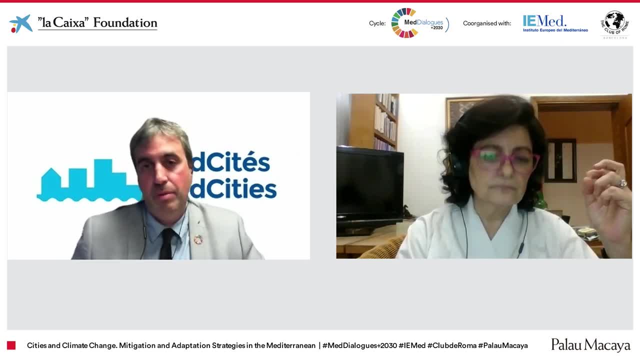 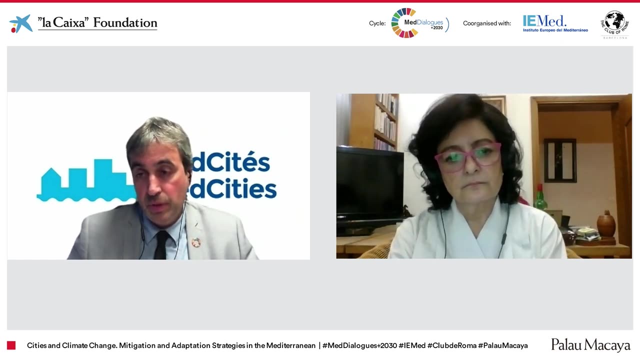 And we can transform these ideas into action, Maybe. So I think that much needed the union of municipalities in institutions like MedCities We have Hannah. we have two questions that the organization said that either we could answer you or me, But I think that one is maybe more appropriate to I could answer and the other for you. 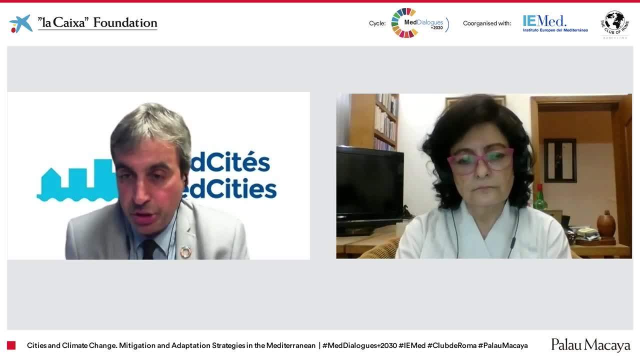 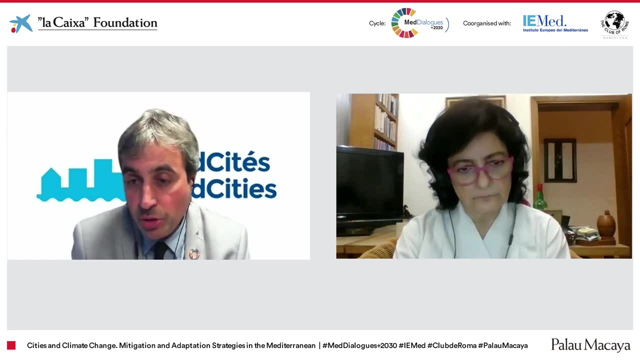 What do you think? One is: the panelists mentioned that the majority of municipalities lack the administrative and fiscal capacity to carry out sustainable projects. Could you give us some examples of how could cities improve their capabilities to implement greener urban planning and actions? This I could say something upon this. 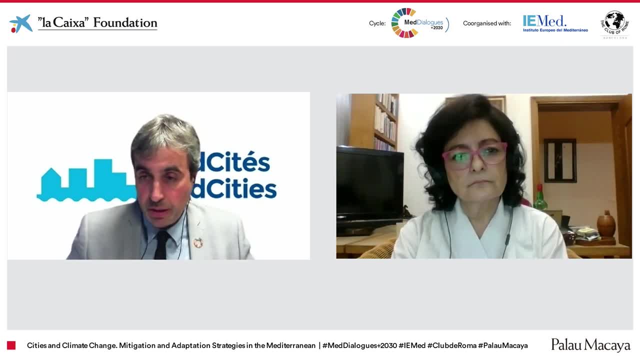 But of course you are free to say. And the second one will be: given that Lebanon suffers from dramatic electricity shortages, Are there any initiatives led by municipalities focusing on improving building energy efficiency or promoting sustainable energy like solar in the city? Will the current crisis lead to a spark new initiatives? 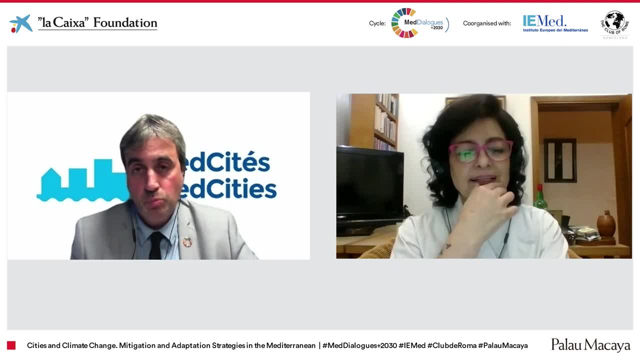 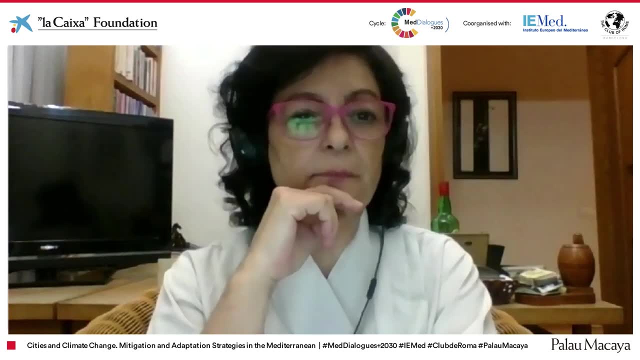 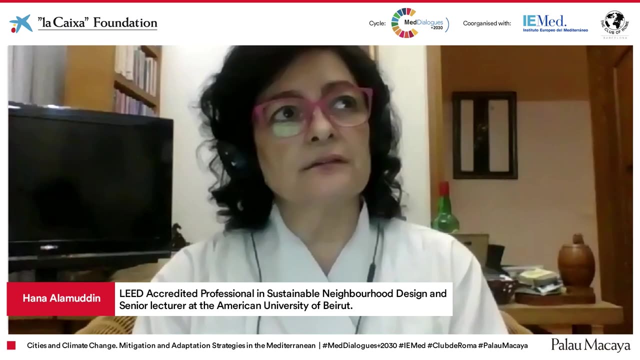 Please. Okay, I think that definitely the current crisis has woken everybody up And it's made people aware. Now The demand on solar panels has increased a lot And people have realized that not only is it expensive, it's also unreliable to depend on the local electric situation. 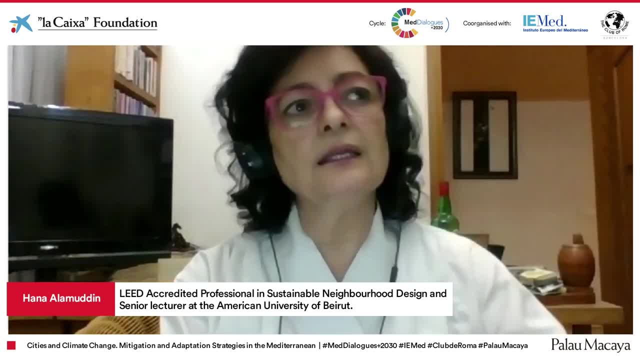 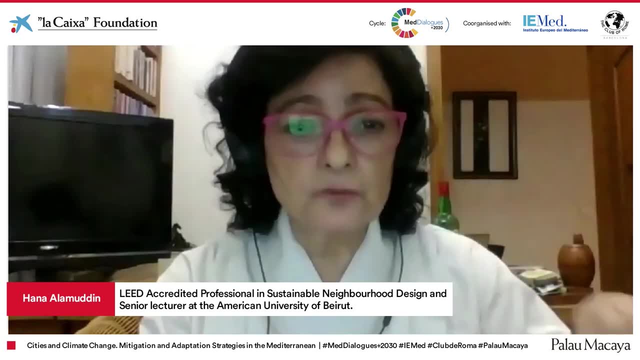 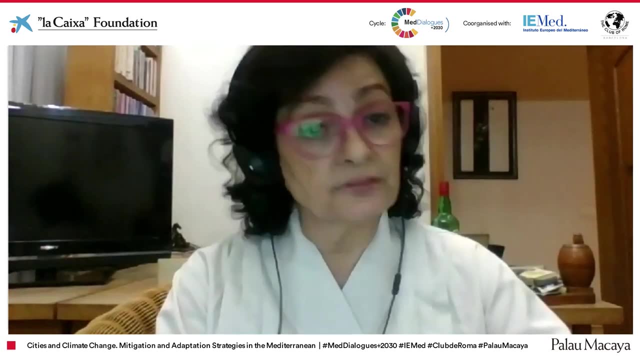 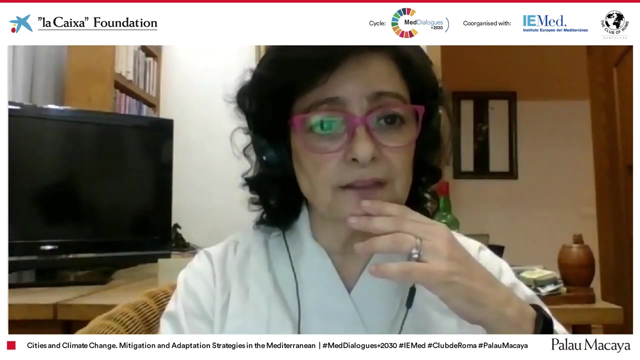 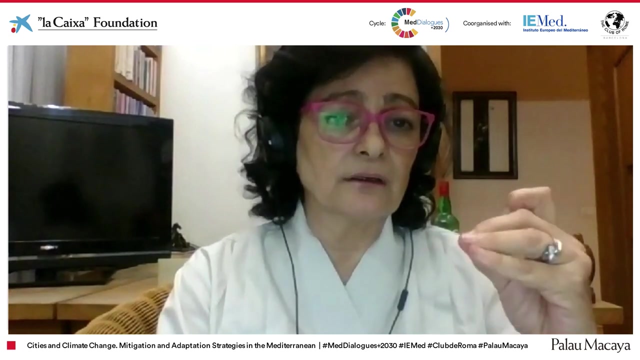 Now there is a legal issue here because legally the electricity has the monopoly to provide power. So in a way this needs also a change in the governance And change in the laws to allow different municipalities to function and to do that, But definitely at the private level. there is a lot of demand and increase in for solar panels. 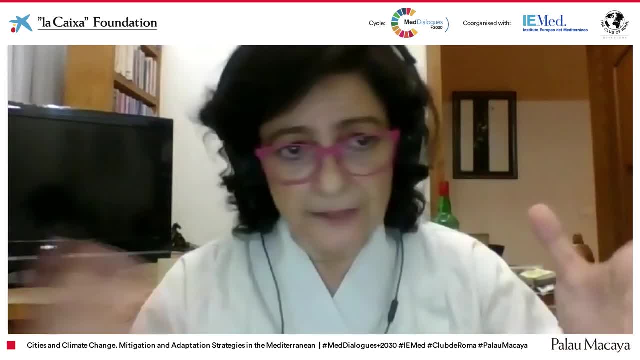 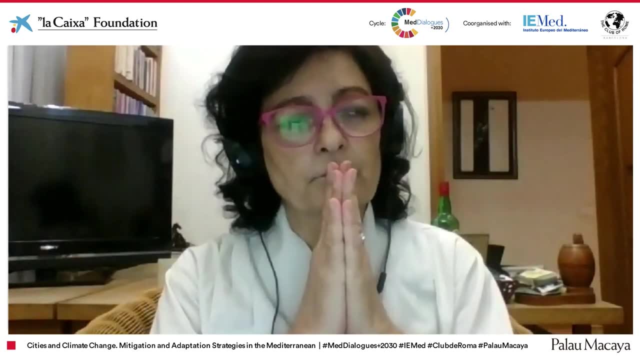 And I think that at the moment we are in the middle of the mess And I think you know, we're all just on survival mode. You know it's just like day by day, But there is a major change. There is a major change in the way people are seeing their lives. 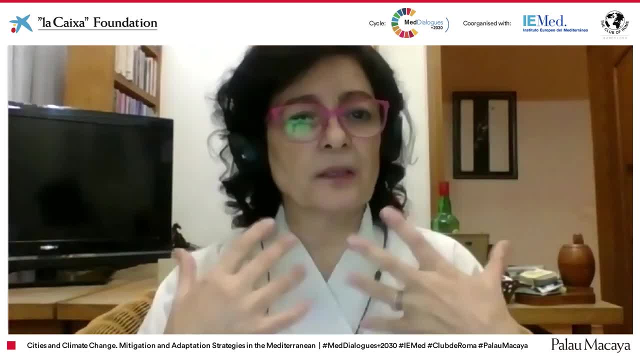 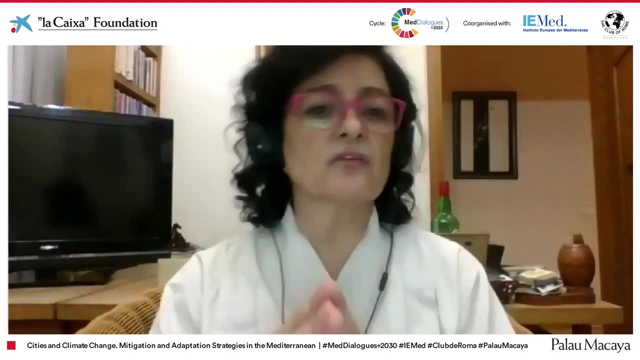 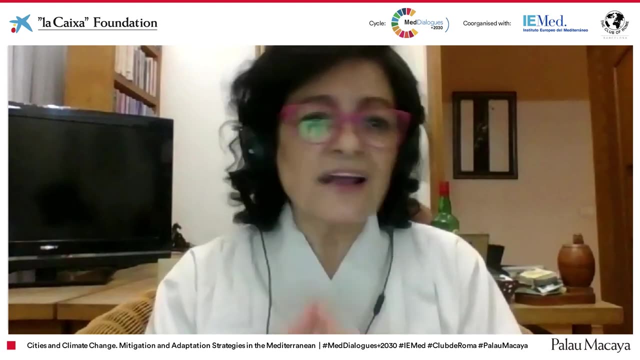 And even the way they are using money and buying things. And local industries have become much stronger because imports have become very expensive And so there's a lot of local products that have come on the market and so on. So it has been good in that sense. 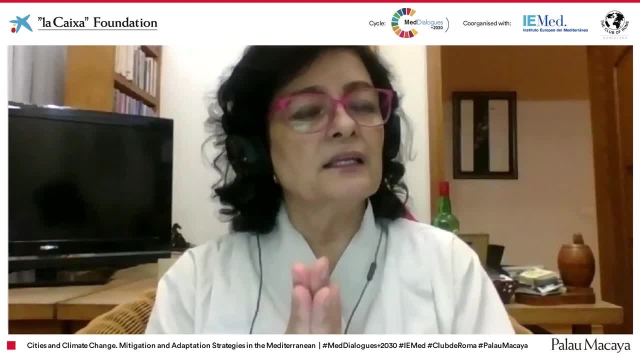 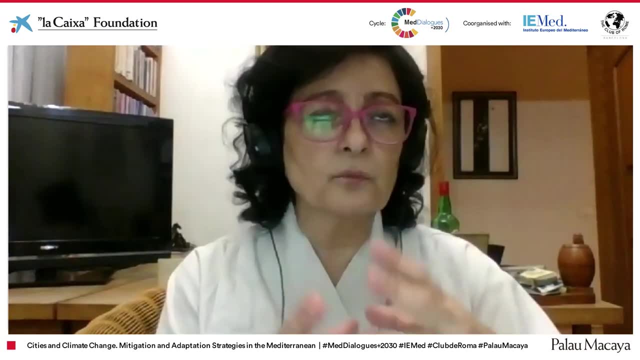 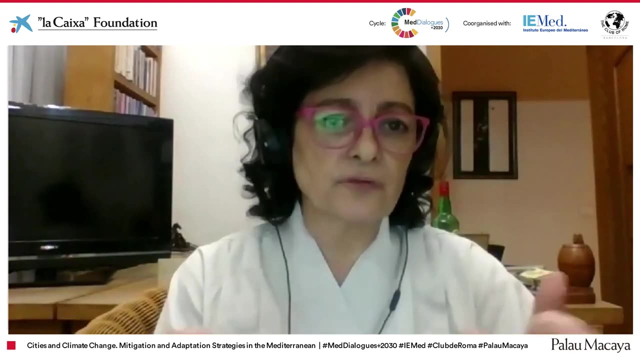 And people have realized that they don't have to have the old system. They can actually break away from it. But again, depending, one has to keep in mind that there is a whole political setup in this country that is in control of resources, of the legal situation, everything else. 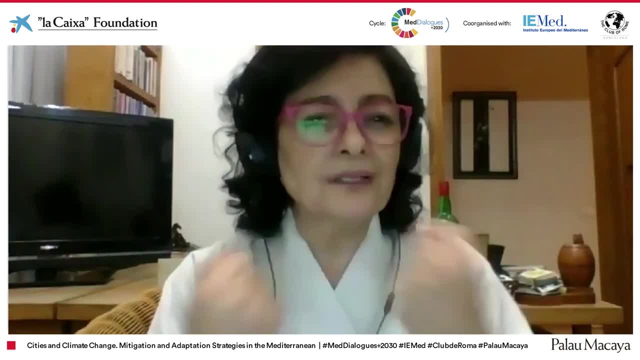 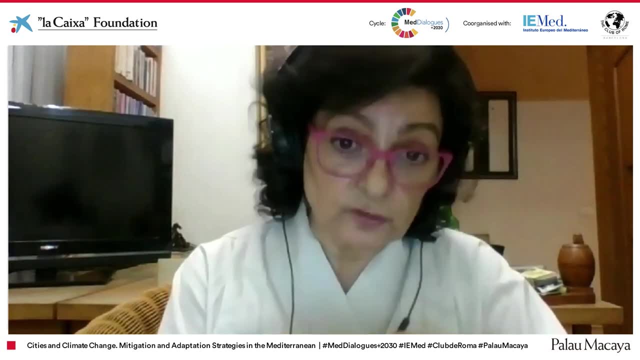 And there's a need to break that before you're able to really move forward. But hopefully they will be intelligent enough to realize that they need to change too, Because you know they're coming to the end of their lives. They're coming to the end of their logic, you know. 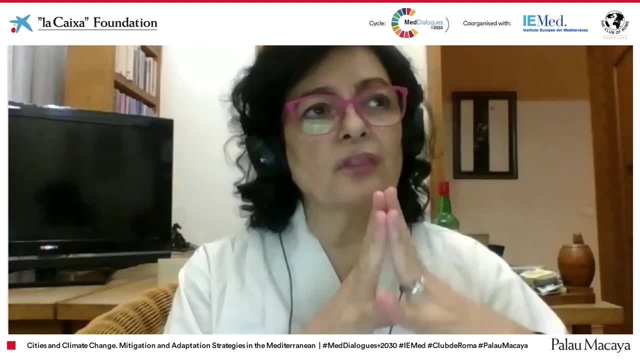 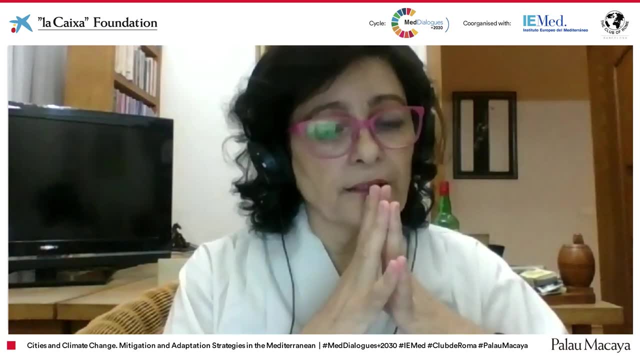 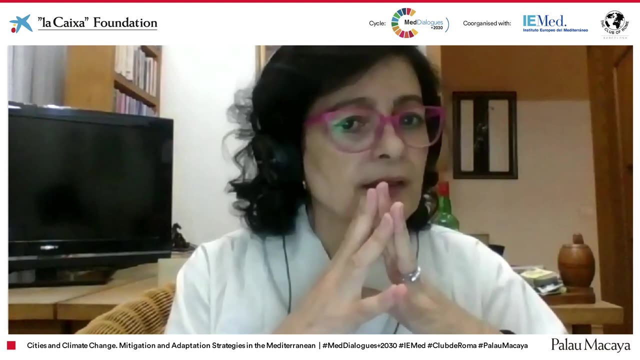 Unfortunately. I just want to say one thing: Just because the shooting stopped doesn't mean that the war has ended, And really it is something that one needs to keep in mind when you look at countries like Syria and Libya and you know, because really war can take very different forms. 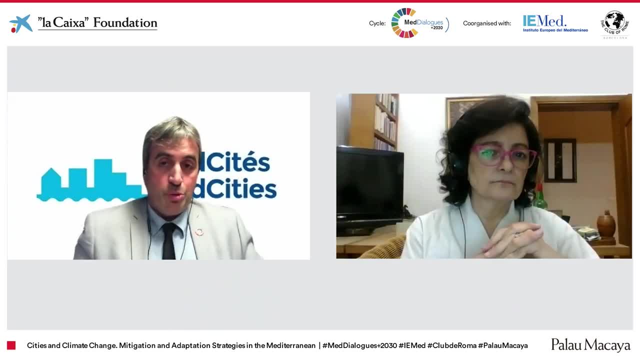 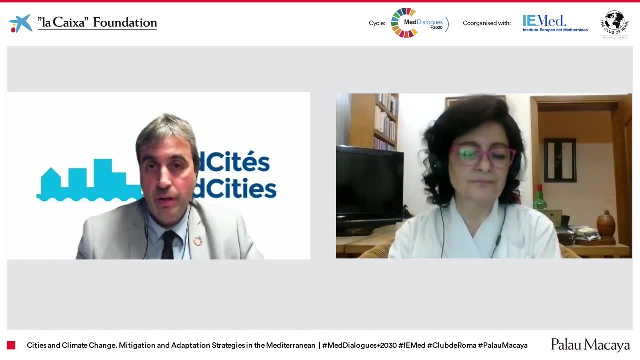 Sure, Very true, Very true. And when the guns stop, we take the attention to another way, to another place, And this is not what we have to do. Let me provide some ideas. regarding the first question, How could cities improve their capabilities to implement green urban spaces? 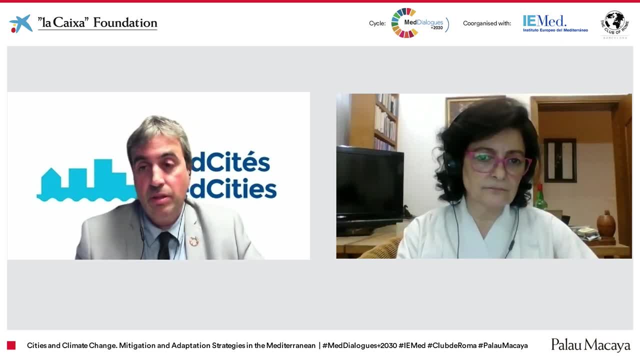 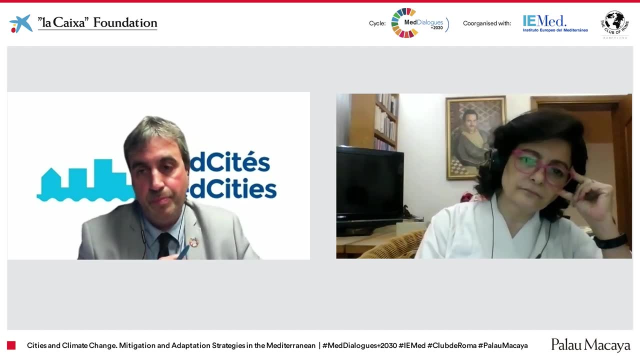 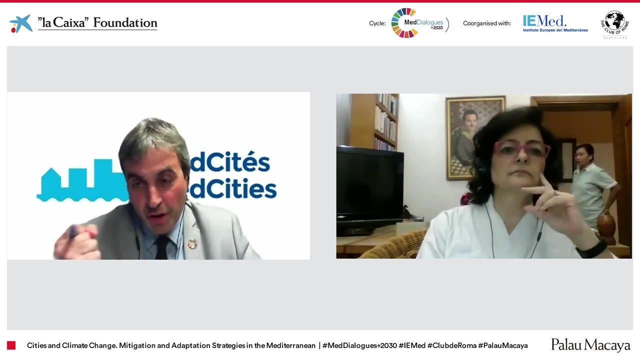 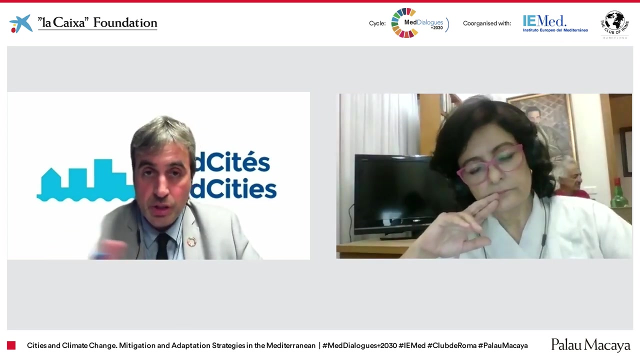 Well, for example, when you have the lack of competencies or the lack of possibilities, of capabilities. This is why networks like MedCities, for example, have their raison d'être, the reason of their very existence. For example, we promote the city-to-city cooperation, the city-to-city transfer of knowledge. 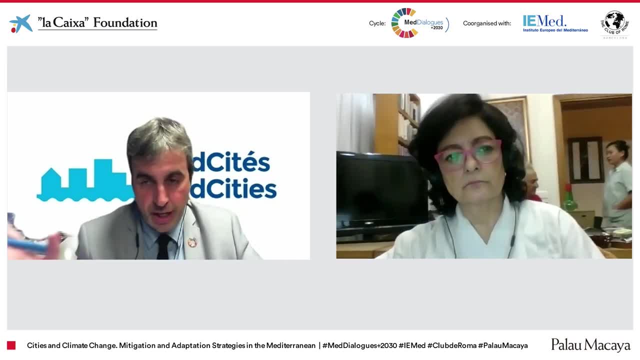 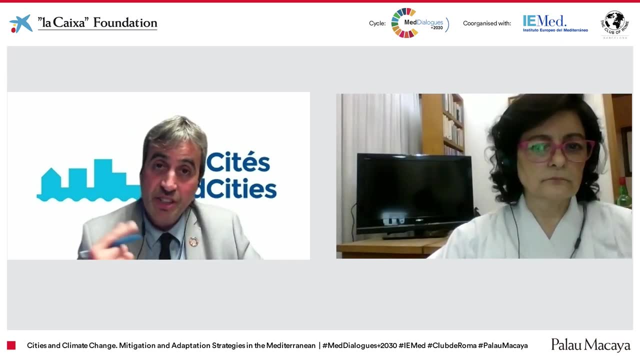 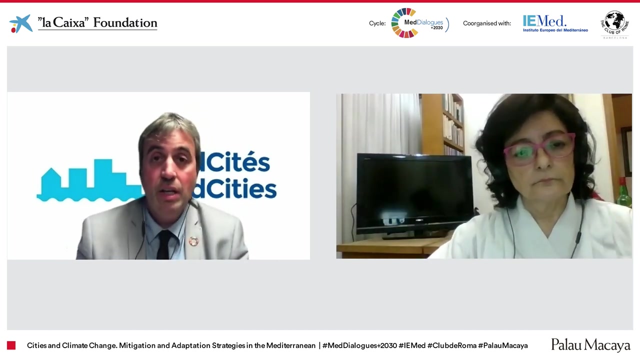 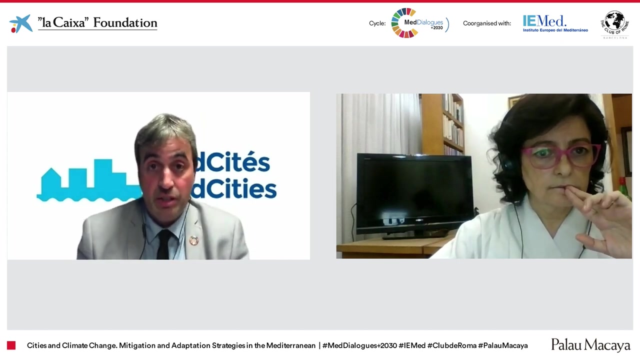 In fact, we have knowledge transfer centers in Tunisia and in Lebanon. Last year, for example, we conducted our first cycle of capacity sessions for our member cities, regardless of the projects that we have conducting with international funders. Thanks to the Barcelona metropolitan area and the government of Catalonia, we had some resources to make a general capacitation of our cities. 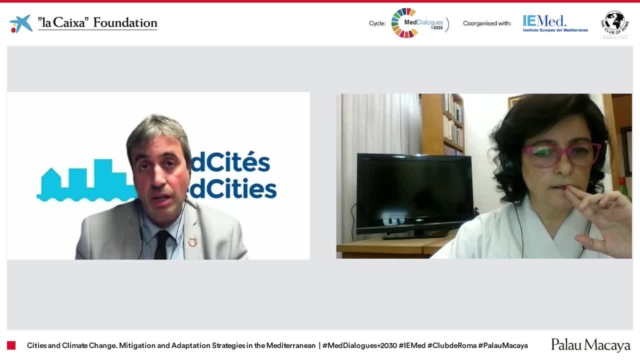 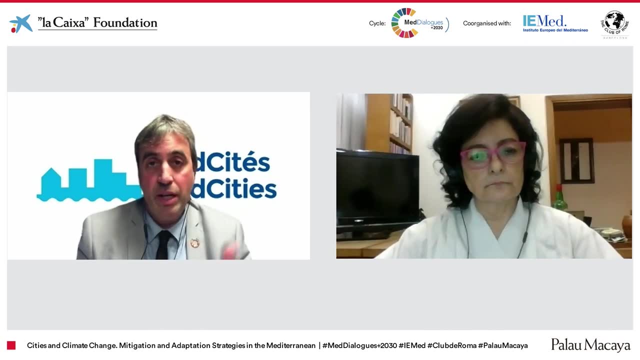 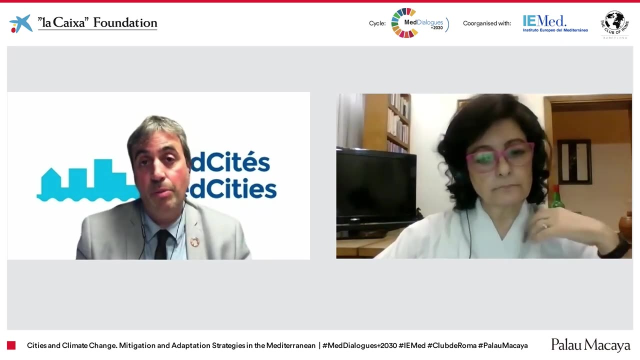 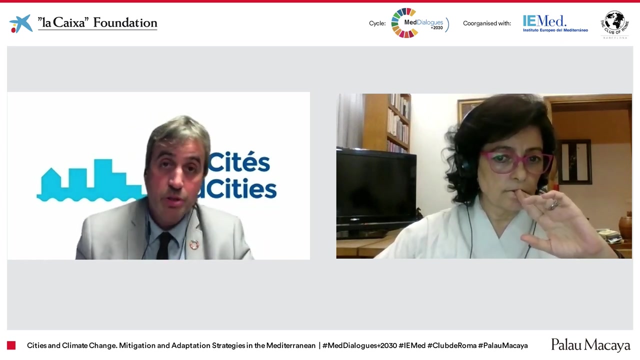 For the elective representatives and for technical staff. So we conducted four sessions, four cycle of sessions on waste management, energy, sustainable energy management, sustainable mobility and environmental management like nature-based solutions, And we were conducting these capacity sessions and with mentoring sessions with some of them, with our members. 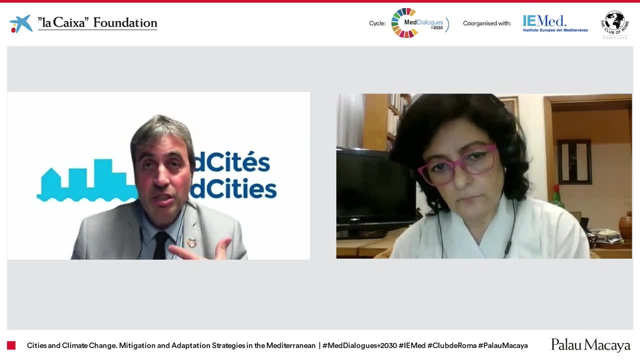 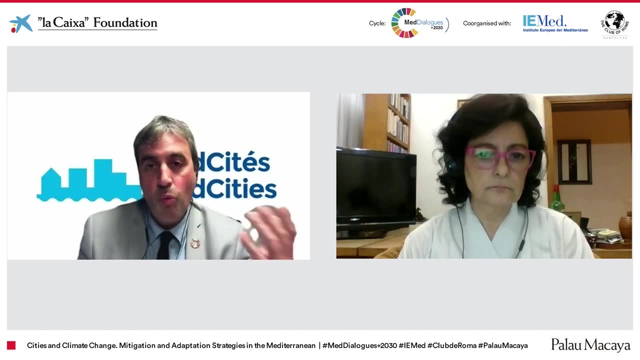 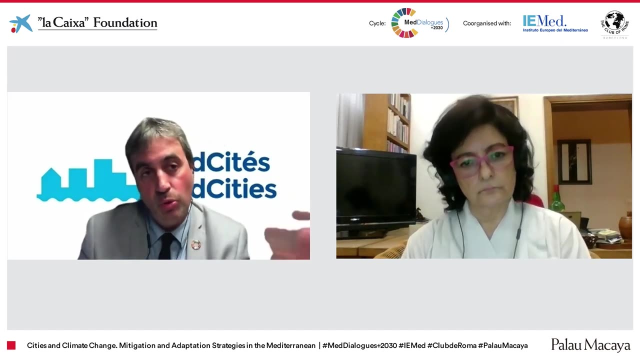 So it is possible. For me it's a challenge. It's a challenge. It's a way of transferring capital, money and also brain capital from one cities to the others, from the learnings and mistakes from ones to the need of capacity building of others. 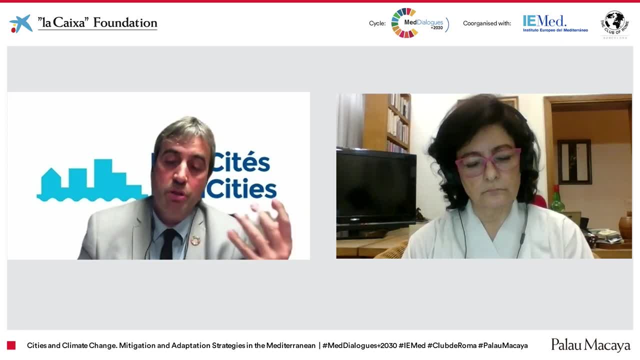 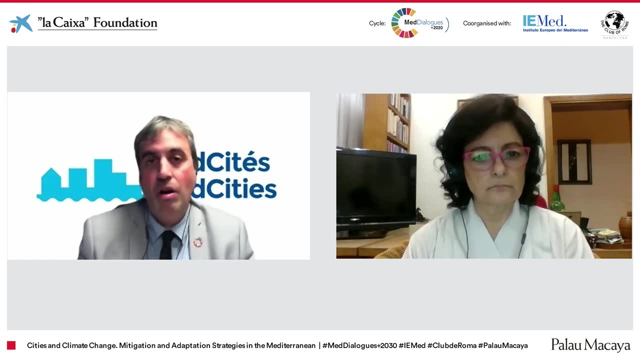 So there is room to do things. But of course it would be easier if each state would help every and each of their own And to asphalt their own municipalities to build their capacities. But when there is a lack of that, it's when appear international organizations like ours. 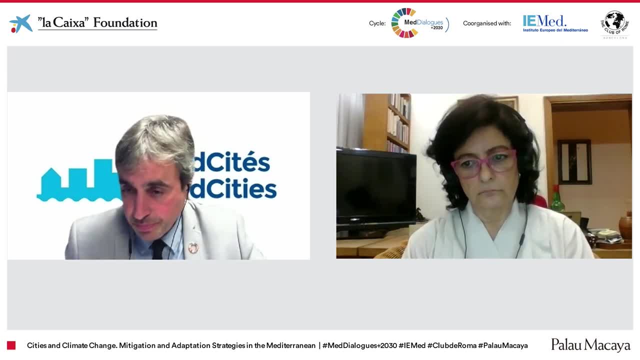 So there are possibilities there in that regard. Let me check if there are. yes, there are more questions. We have 10 more minutes. The third question: what can we learn from traditional architecture to adapt and mitigate climate change in cities? Hannah? 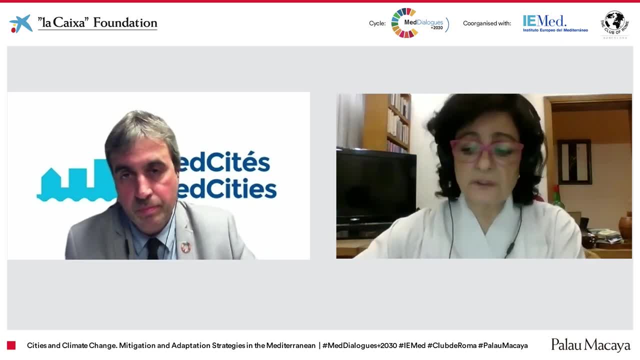 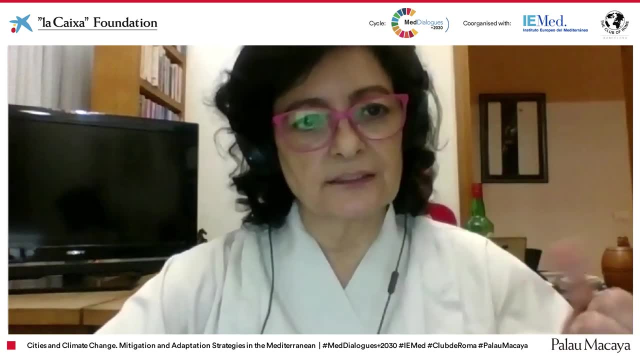 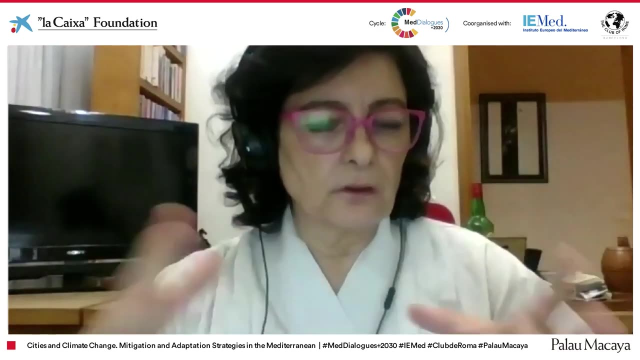 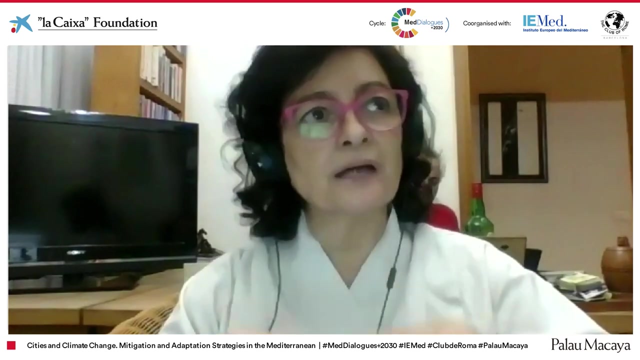 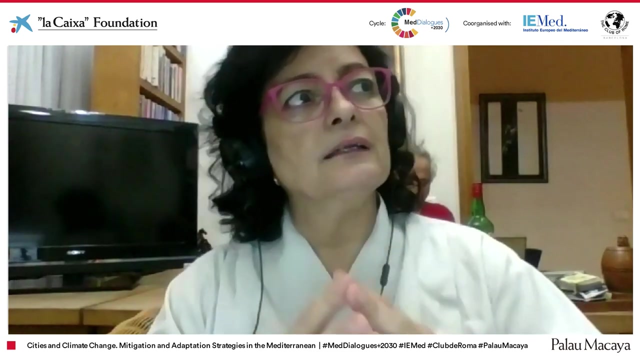 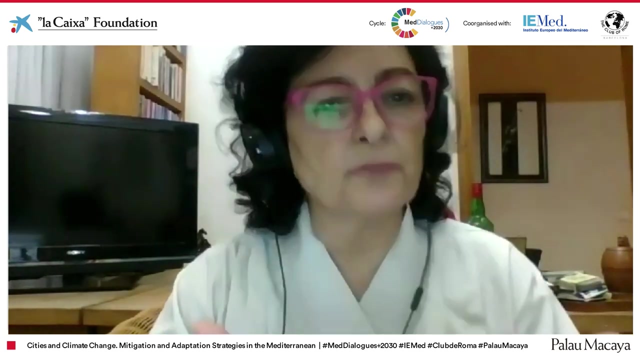 Yeah, sure. Well, the problem with cities is that it's a question of density, and so the whole nature of architecture of cities is different from your sort of traditional architecture, which tends to be, you know, independent units. However, there is a middle section here which is not the traditional architecture as such, but the mid-rise, ie the environments cities that were probably built, you know, in the 19,, before the start of the introduction of lifts, you know, as I'm certain, 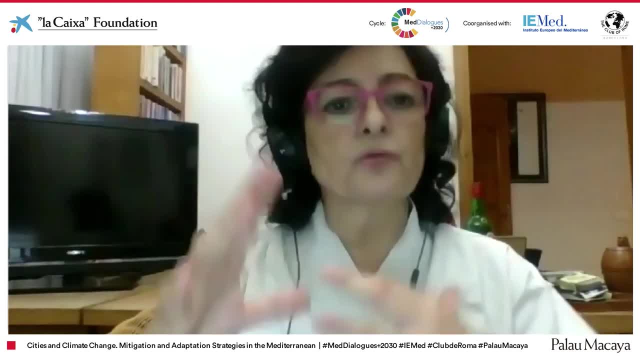 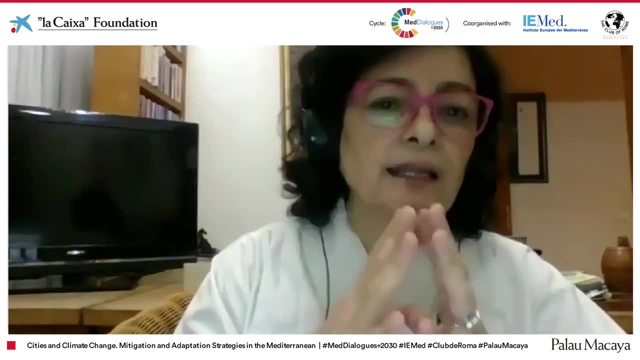 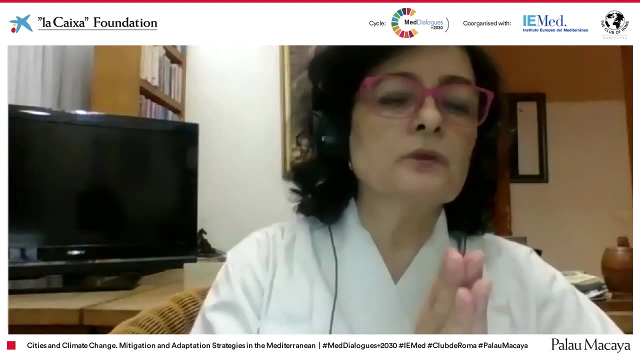 When there were no lifts, walk-ups, what they call the walk-ups, where we're talking about buildings that are six to seven stories high. They create a very interesting climate situation whereby you're able to control the microclimate with them and you're also able to control services and so on and the interaction of people with the street. 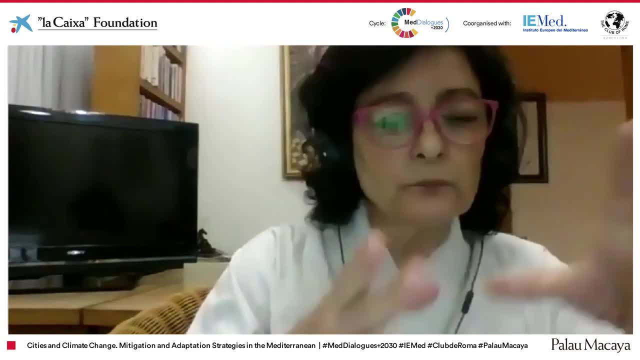 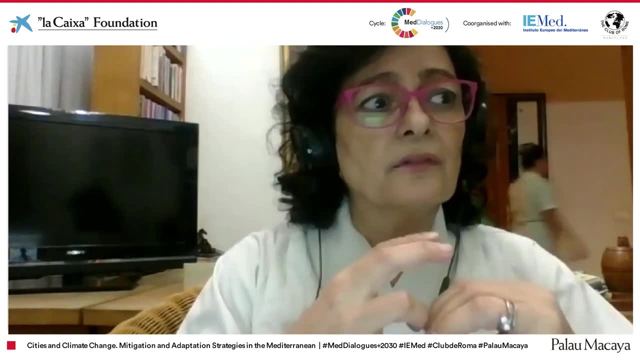 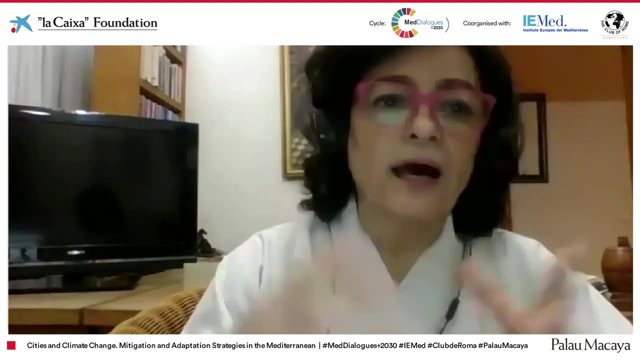 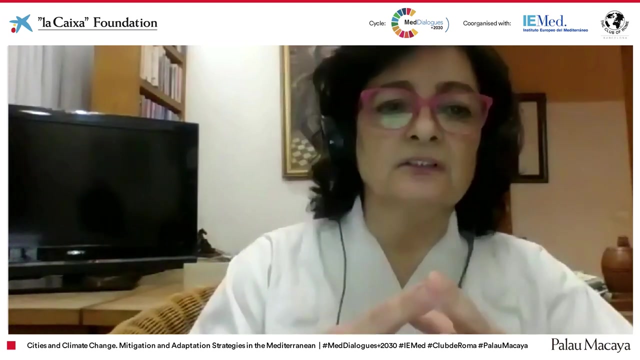 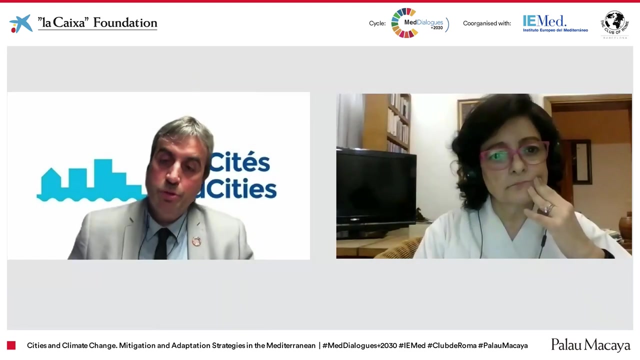 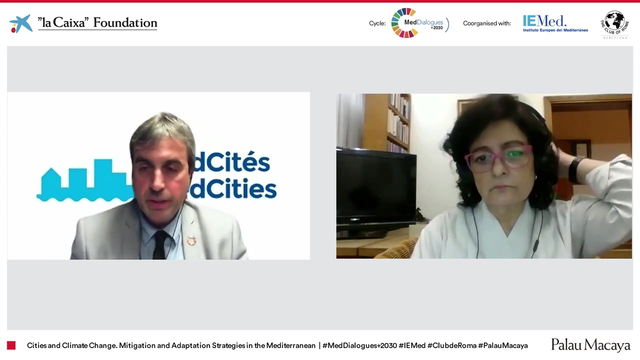 So I wouldn't go for traditional architecture but I would go for an architecture for cities that is really medium height, that has the density required to make buildings Right Interesting. Thank you. We have a fourth question and maybe I could provide some ideas. 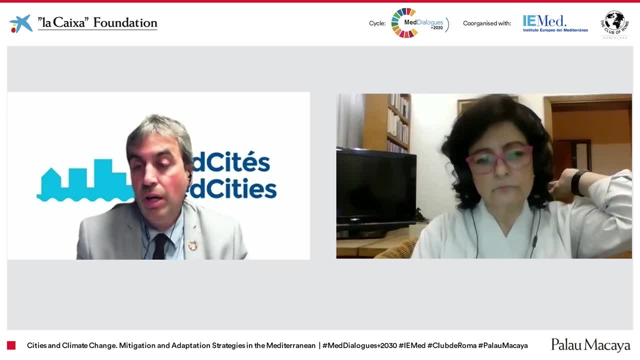 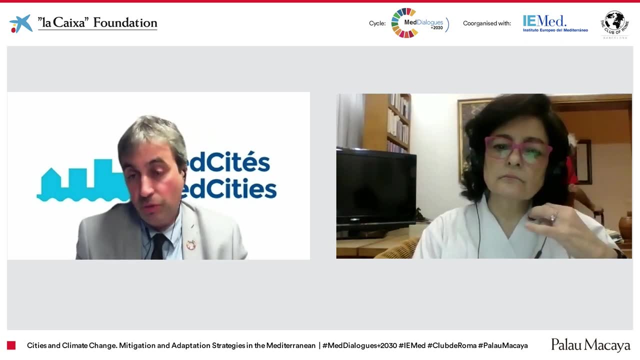 The question is: do you see inspiring examples- and you, of course. if you haven't inspiring examples in the Mediterranean regarding cities fighting climate change, of course, Could you mention a successful case of a city from the northern Mediterranean region and one successful? 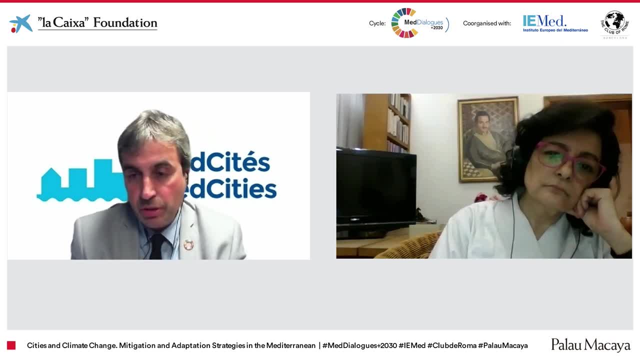 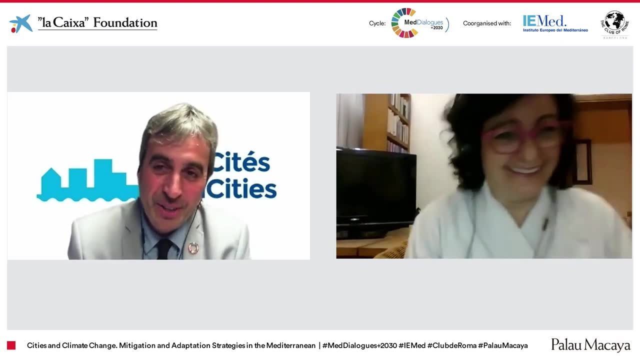 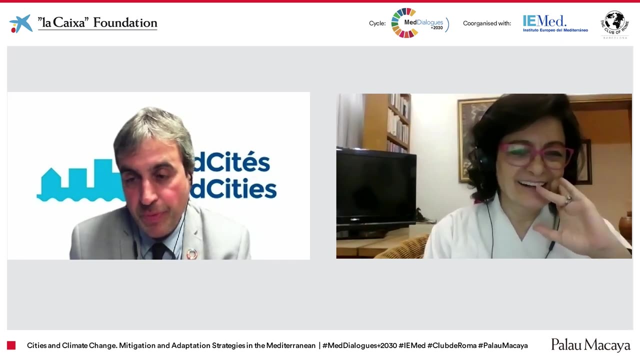 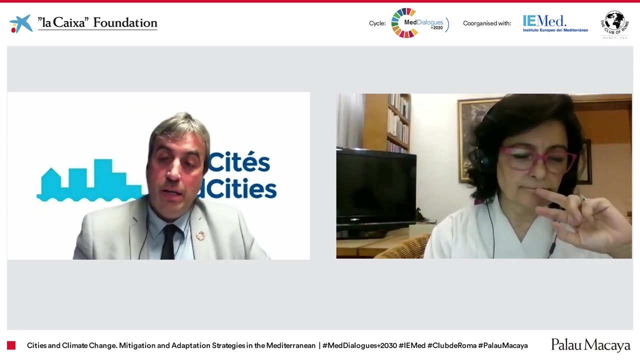 example from the northern region, so from this other region, apart from Lebanon. Lebanon is a disaster case. You showed some bad examples and some few good examples, also in small cases, Small scale cases. Well, yeah, there are some, I could say. 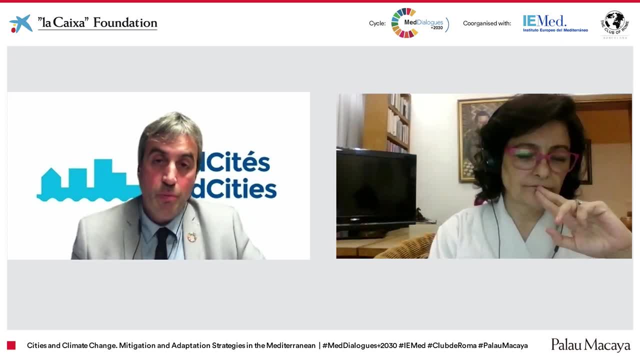 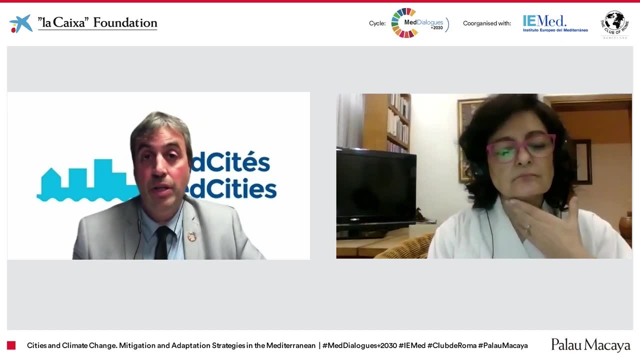 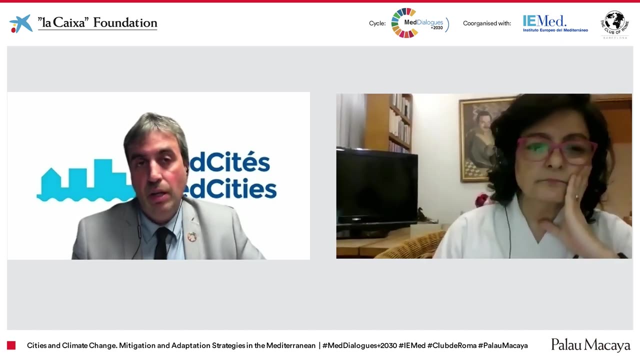 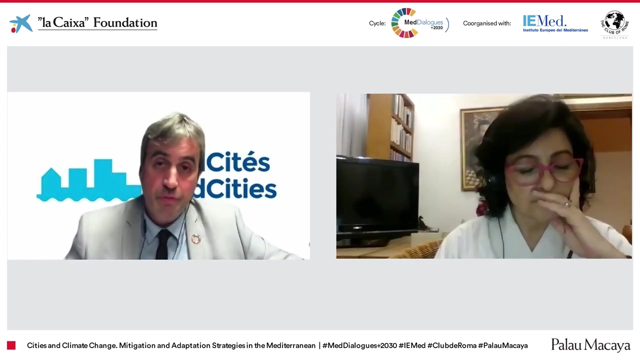 Let me not speak about maybe one. I can speak from one city, for example, a city where I am now. in Barcelona, They have officially declared the climate emergency, so they have also a planning for green spaces. They have conducted in this house, in Barcelona, in fact, with Metropolitan Vision, they have conducted a restricted area. 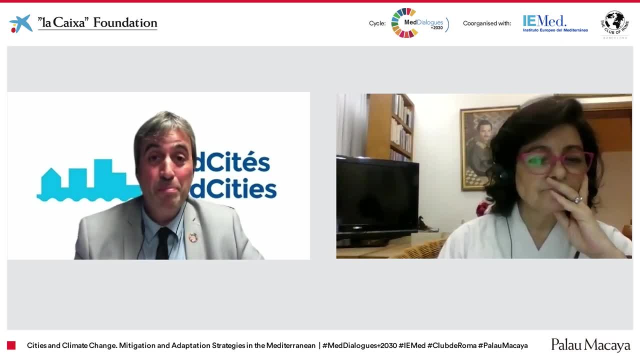 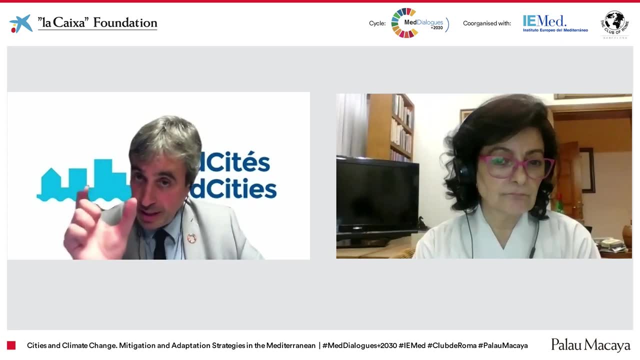 for some cars. Some cars cannot enter not the city centre but a great part of the metropolitan area. Some cars that don't have, they don't wear a specific label regarding their emissions, they can not enter to the metropolitan area. so this is a good example. I think that the country has garlic. 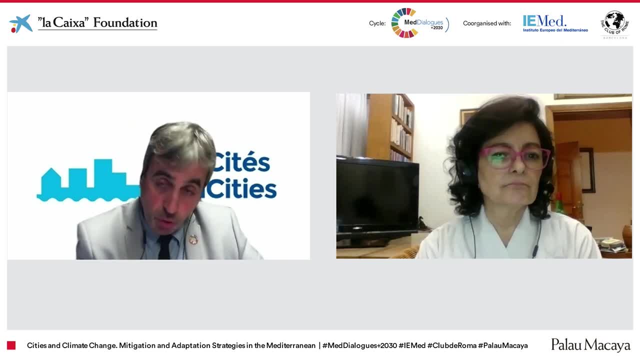 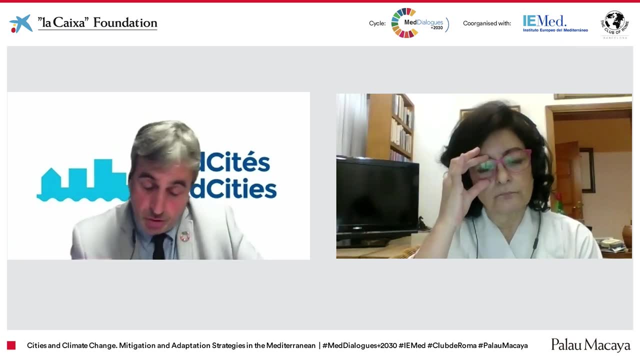 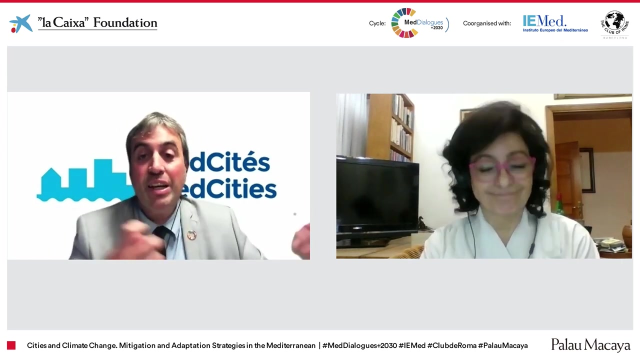 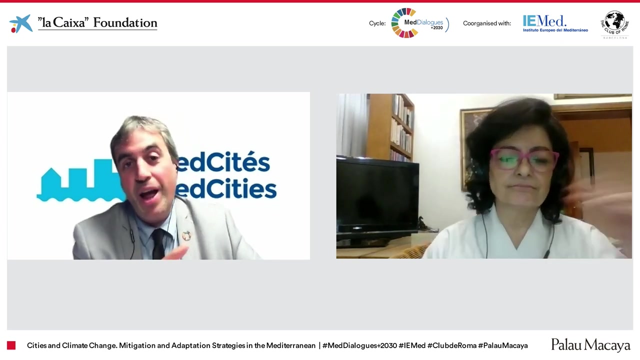 The people fighting local pollution, which is not always the same as climate change mitigation, but of course it has a link, And Barcelona is increasing more and more public spaces, like the Liazon D'Uz that you have showed in Beirut. More and more, they are making the pavement, deconstructing the grey pavement to put green or brown areas. 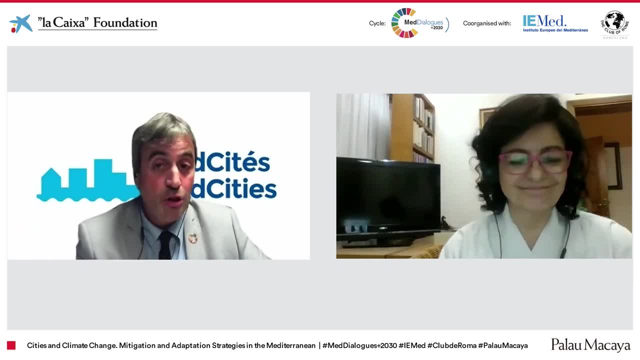 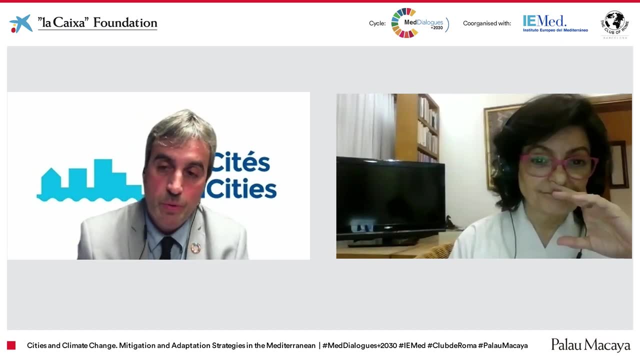 Some are green and some are without any vegetation, but are not grey, are brown, with the soil directly. You can see the soil. So in order to To have less reflection of the temperature, for example from the pavement, or being more habitable, more democratized, more livable, 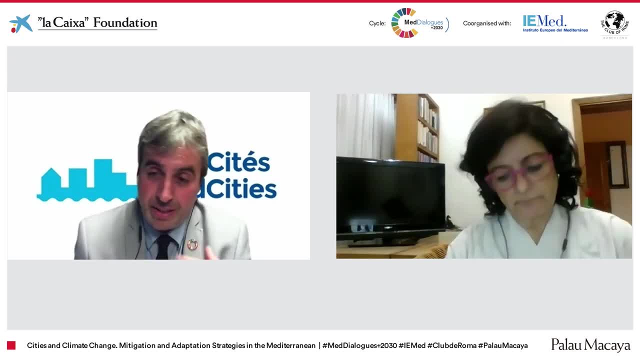 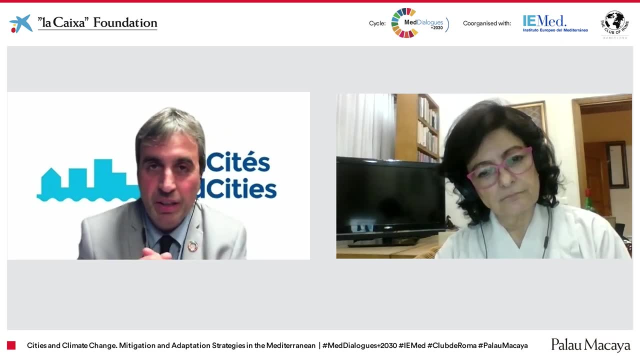 And in the south I would like to highlight: in present time it is not still, it is not a successful case yet, but it will be Estonia, the capital of Tunisia, which is conducting the strategic plan. We are the leaders with metropolitan areas. 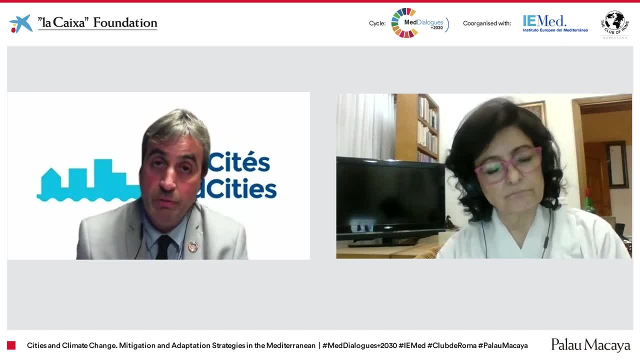 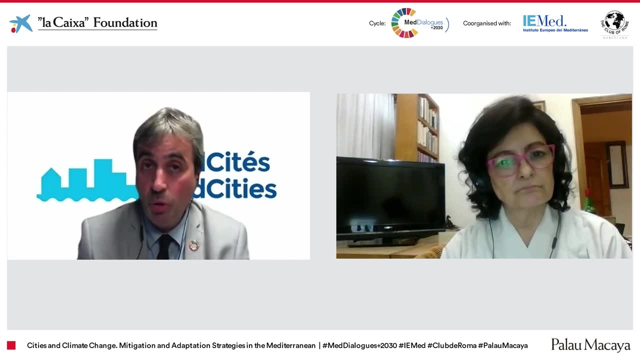 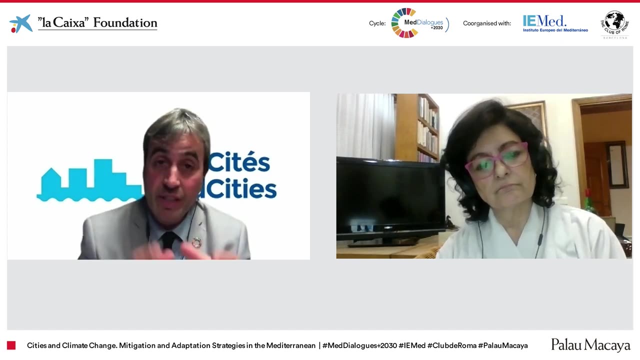 Barcelona and the municipality of Tunis were conducting the strategic plan for four years of the Tunis capital city, linked to the Sustainable Development Goals, So it is awarded by the European Union in order to precisely localize the Sustainable Development Goals of the Agenda 2030. 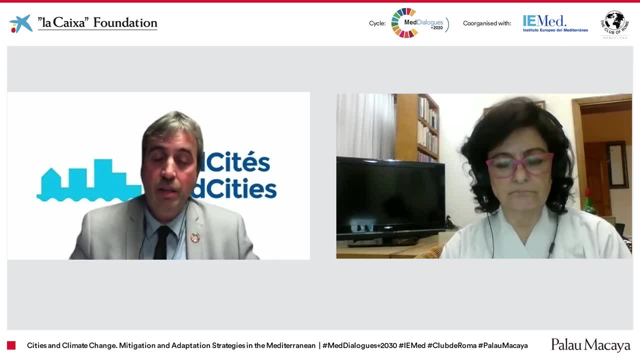 So, with a holistic vision of tackling the climate effects. どうやって são os protestores o que fazem para realizar o problema and the and the causes of the of the climate change? So I invite you to follow this project called Ass sensible tunis, which cities can provide to you, any of you, the audience and hannah information to this project, because 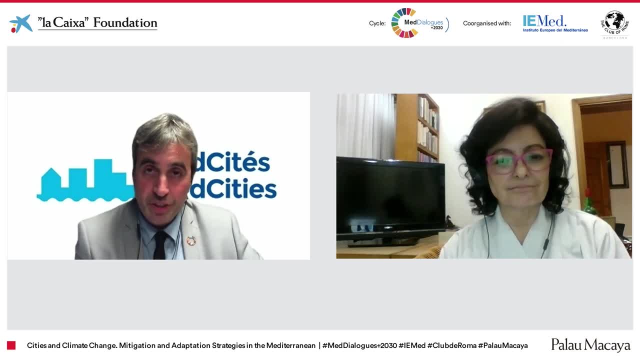 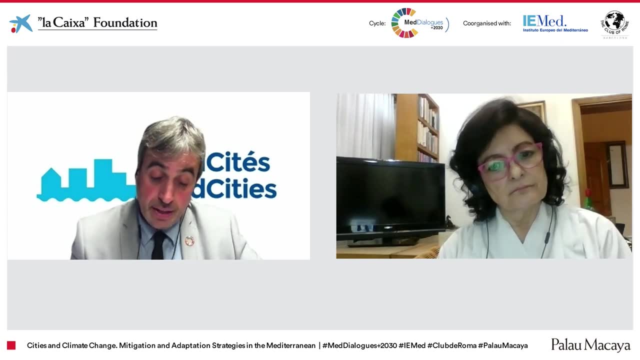 Only you inhabit. this is regarding us, is watching us. many, many institution are. regarding in the final phase, we have The final phase, the third phase of the strategic plan. the final phase of the strategic plan is The final phase. the third phase of the strategic plan is d seguida temos uma nodema do projeto vinculado à gestão do Tículo 다음에 pela Yunnan. e έ believer que há o еще golpe e contribuído aثر do Tículo r diligent em perd Half Part. 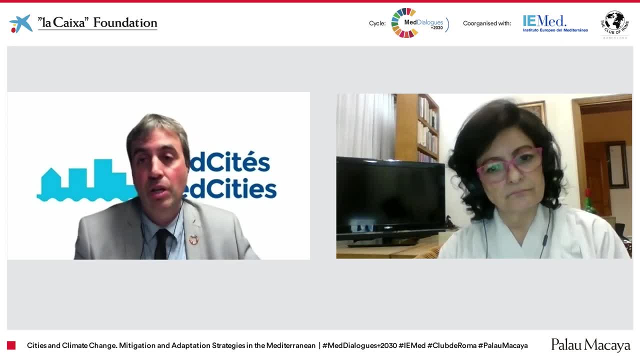 how to capitalize to other cities in Tunisia and in the region. So we will be able to learn from our mistakes and successes from this process, And I don't see any other question. Yes, there is a fifth one, maybe the last one. 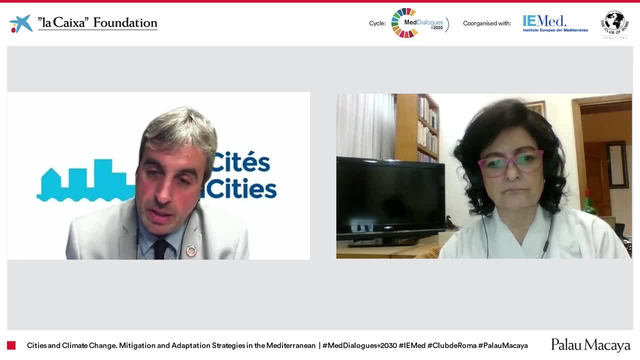 So, Hannah, what will be the role of cities during the COP26?? Will the voices be heard during this crucial event? This is a good one. Maybe did you understand, Or maybe I could repeat What will be the role of cities during the conference. 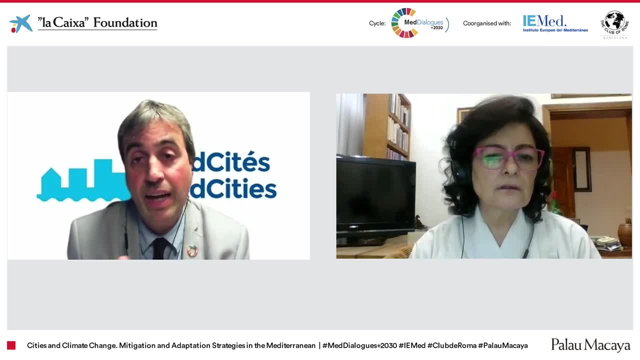 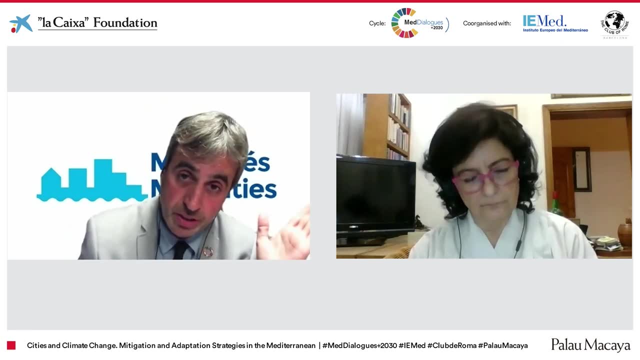 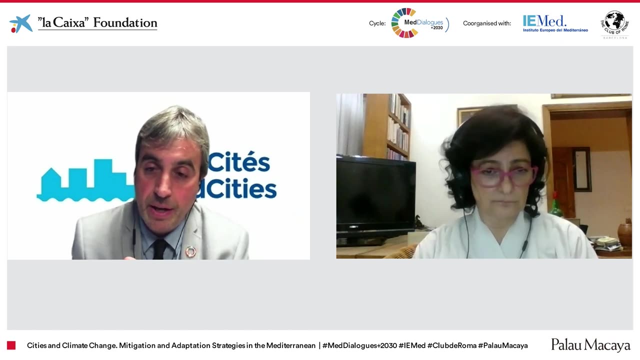 of the parties, 26 in Glasgow. the climate summit that will be held in the COP26? In the United Nations summit, like the Paris one in 2015,. that will be held this year in Glasgow, In fact next month, Will the voices of the cities be heard? 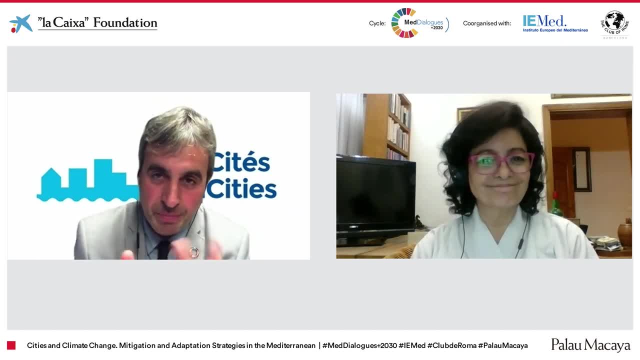 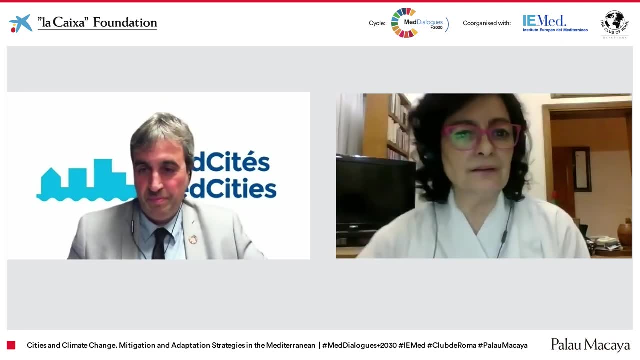 during this crucial event. I have my opinion. Maybe you can express yours. Be free. Well, I mean, I think you are more. it's more appropriate for you to answer this, because you're more up with that, you know. So.